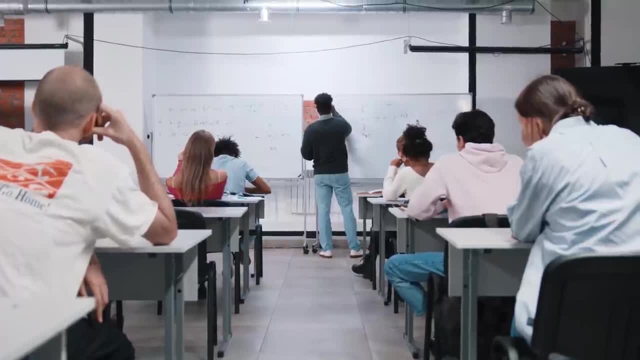 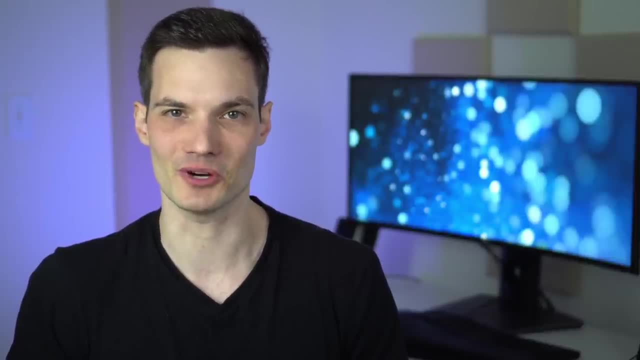 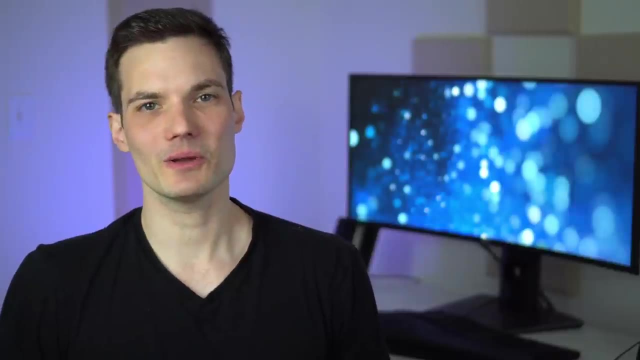 course, that'll give you all of the most essential tools. If you want to jump around this video, I've included timestamps down below so you can jump to the section that interests you the most To get started. you might be wondering: well, why should I even learn how to program? How is this? 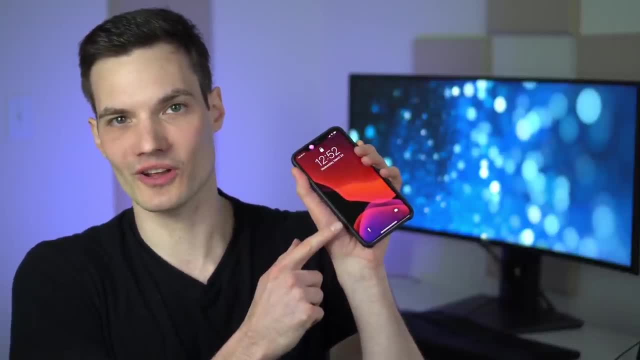 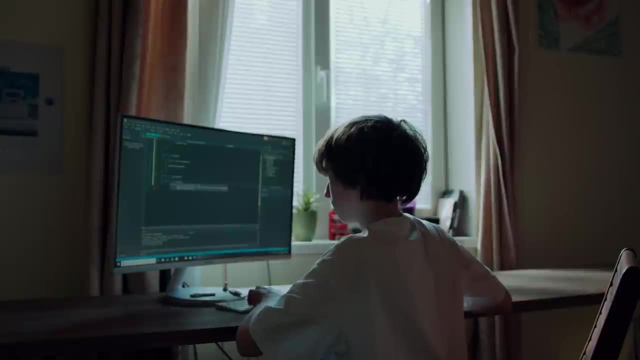 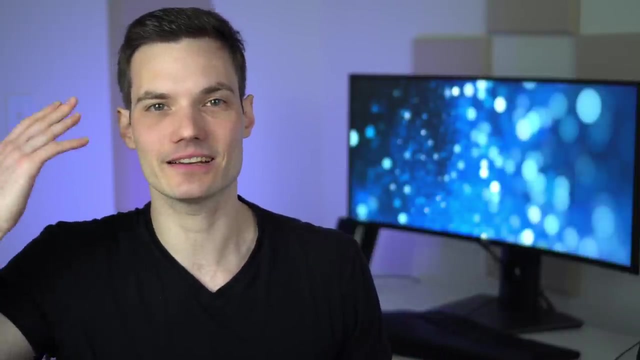 going to benefit me Well. anytime you go on your phone or anytime you go on your PC, you're experiencing the output of something that someone has programmed, so you're realizing the benefit. Think of it this way: To program allows you to take maybe an idea that's in your head. you can 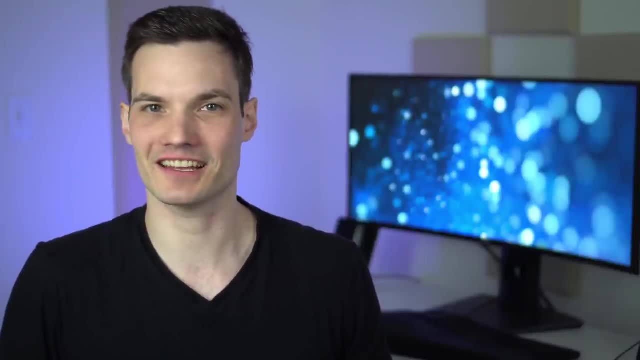 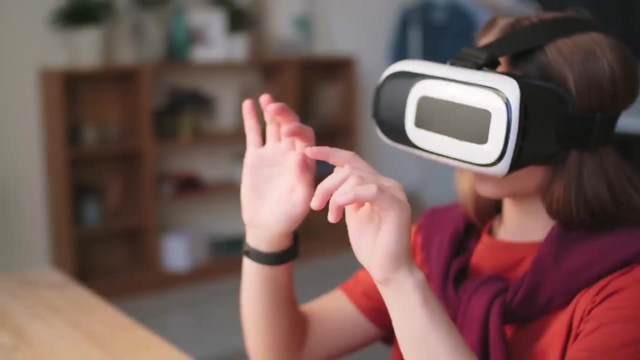 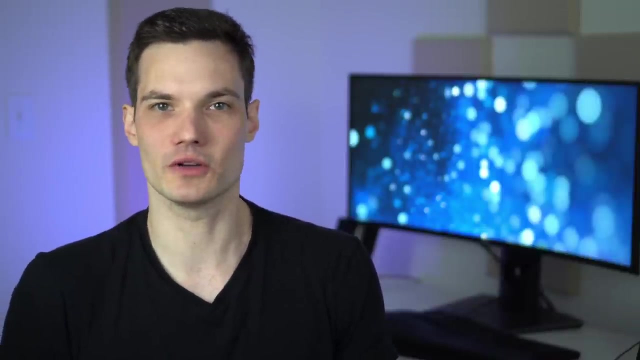 put it into a series of steps that the computer can understand and execute. How cool is that? So, for example, maybe you have a game that you want to create, Maybe you want to create an application at work to help simplify what you do on a daily basis. By programming, you can do all. 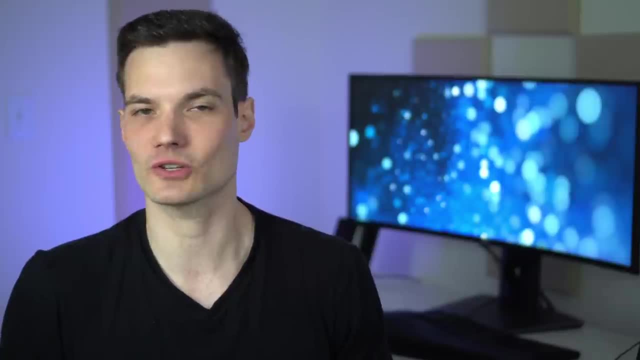 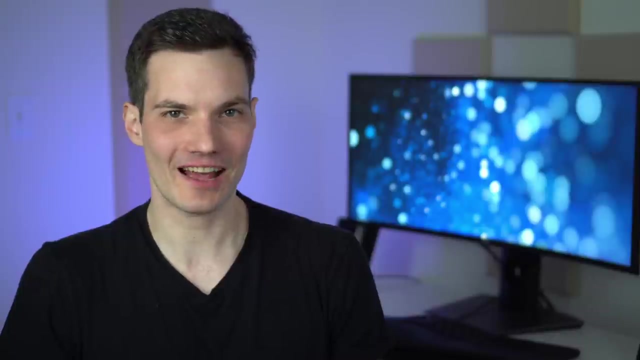 of those things. It's an incredibly powerful skill to learn how to use. Okay, so you want to learn how to program, but why Python? There's so many different programming languages out there. You have C, C, Sharp, C++, Java, JavaScript, PHP, and the list goes on and on. 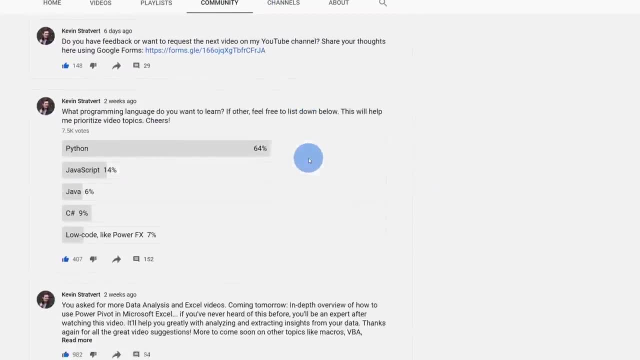 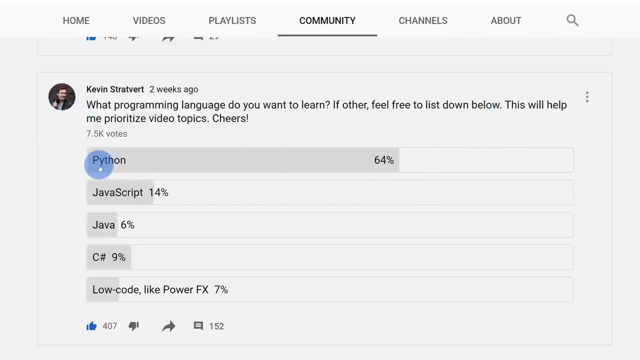 Well, recently on my YouTube channel, I asked all of you: what programming language do you most want to learn about? And overwhelmingly, far and away, Python was the clear winner. It was something like 65% of you wanted Python, And it kind of 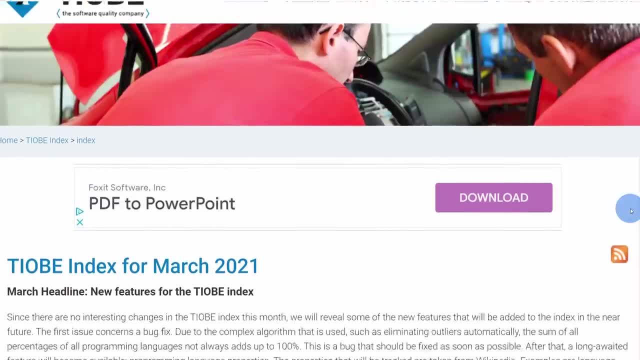 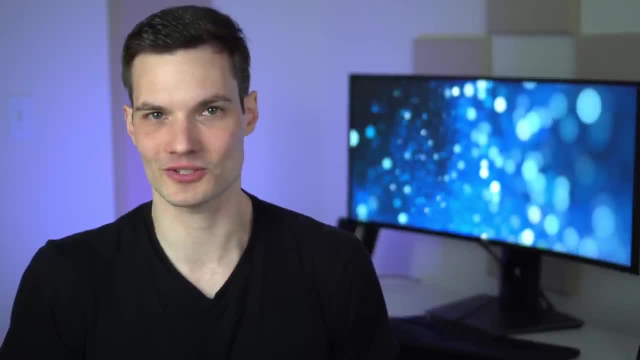 depends. When you look at the lists of the most popular programming languages, Python tends to be right near the top. It's been around for a while. It's also pretty easy to use and also understand. When you code using Python, it tends to be a very concise programming language. 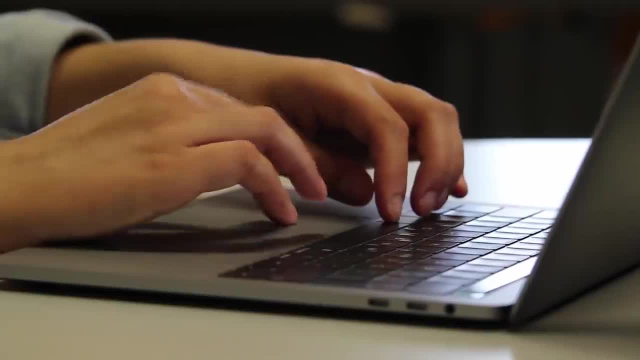 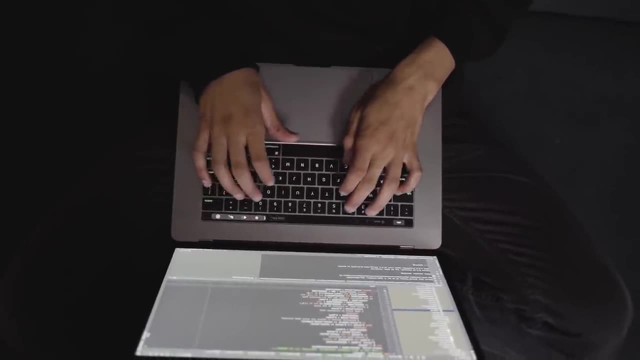 It's also a good general purpose programming language, And what I mean by that is you can write all sorts of applications. Maybe you want to write a web app, an internal company tool, a game, or maybe you just want to conduct some scientific analysis. 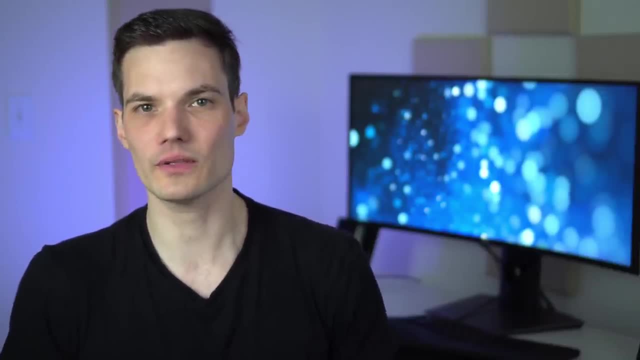 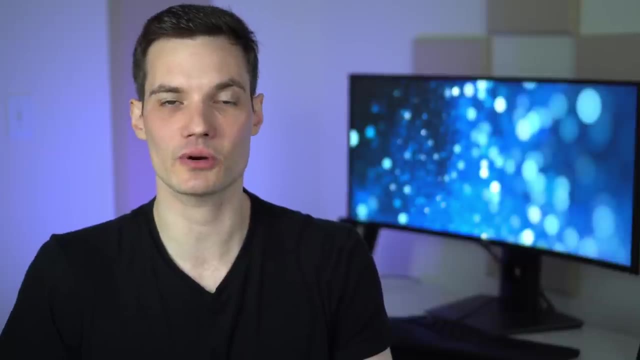 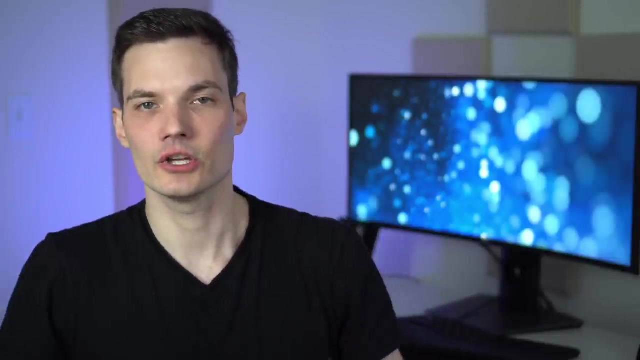 You can do all of that with Python And all the things that you learn today related to Python. you can take these same concepts and you can apply it to other programming languages as well. And really fundamentally, you just want to take some idea you have, you want to turn. 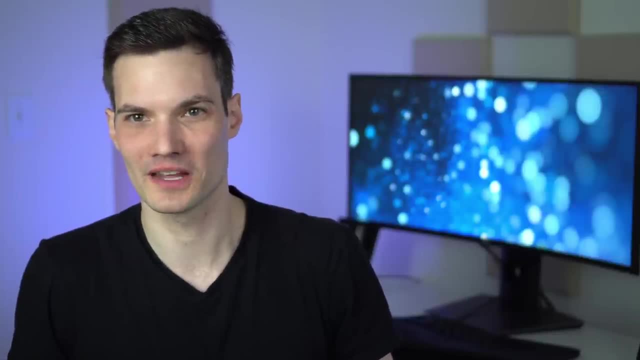 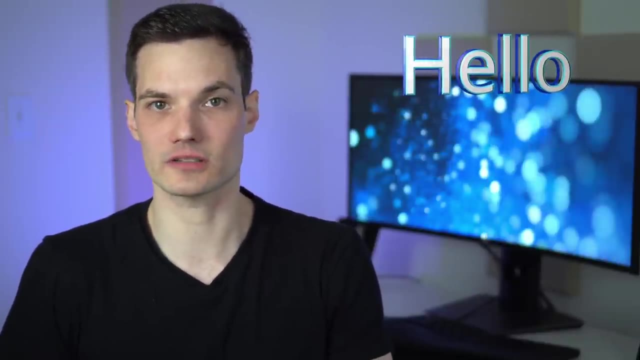 it into a series of steps that the computer can execute And in a sense it's kind of like a different language or a spoken language. So in English I say hello, In German I'll say hallo And in French I'll try my best. 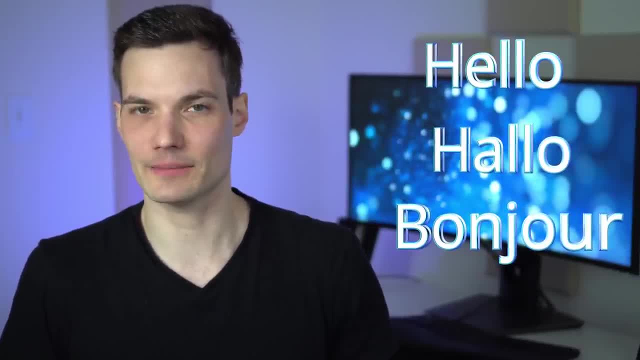 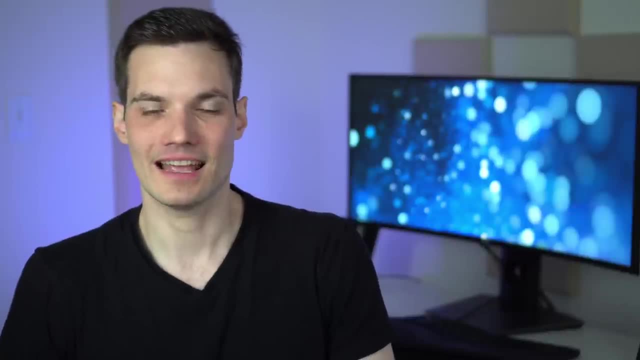 I'll say bonjour, And all of those communicate the same idea. I'm just saying hello, but it's a slightly different way of saying it or speaking it, And that's the same with a programming language. They have different syntaxes. 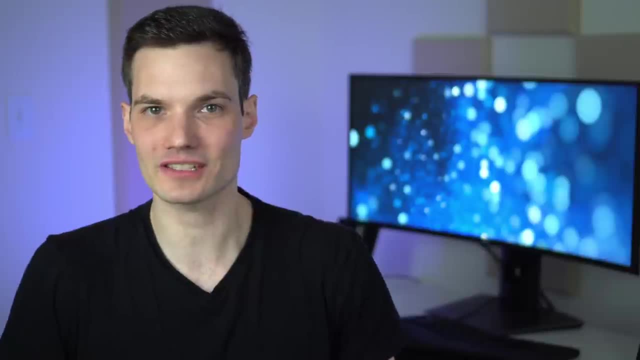 They also have different rules, But at the end of the day, you're simply trying to communicate something to the computer because you want the computer to do something for you. Now, of course, each programming language, You might have its strengths or weaknesses, but you're really accomplishing the same objective. 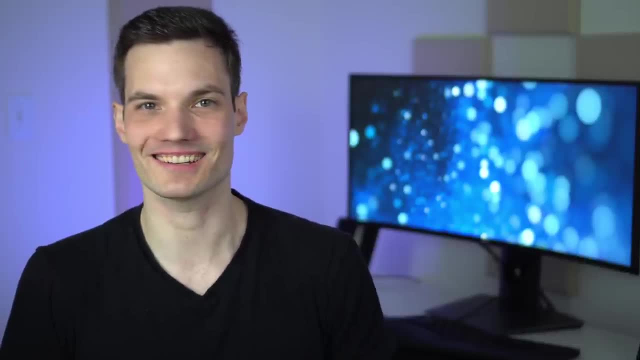 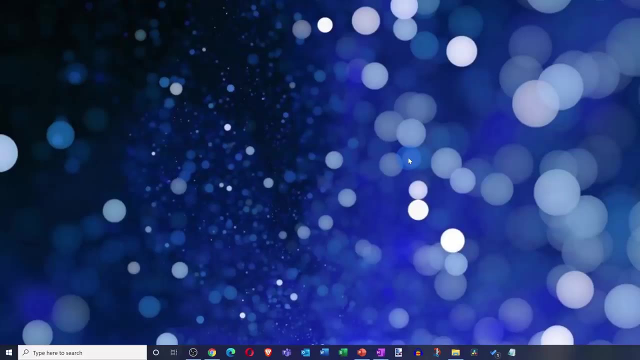 All right. So why don't we jump on the PC and let's get started with Python Here? I am now on my PC And first off I want to check if I already have Python installed To do that on Windows 10, simply go down to your taskbar and, within the search field, type in command prompt: 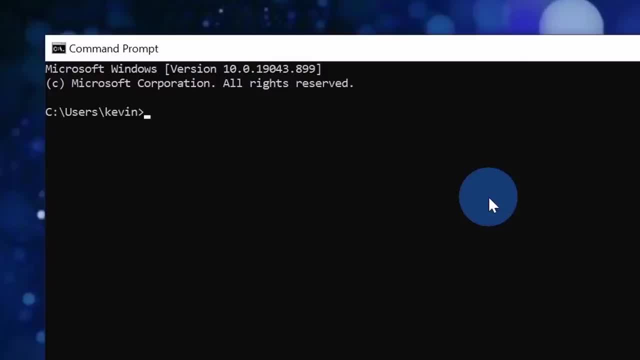 Once you type in command prompt, Click on the best match. This opens up your command prompt and to check for Python, simply type in Python and then type in dash, dash and version. If you have Python installed, it'll tell you the version of Python that you have. 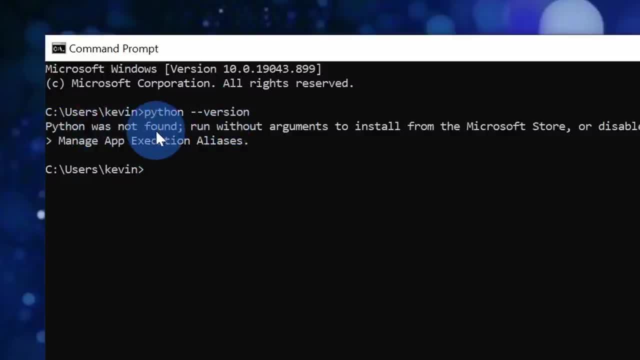 And here you see, I just type this in and it says: Python was not found, So I need to go and install Python. If you already have it, you can skip the next step. If you don't have Python, like me, stick around and I'll show you how you can get Python. 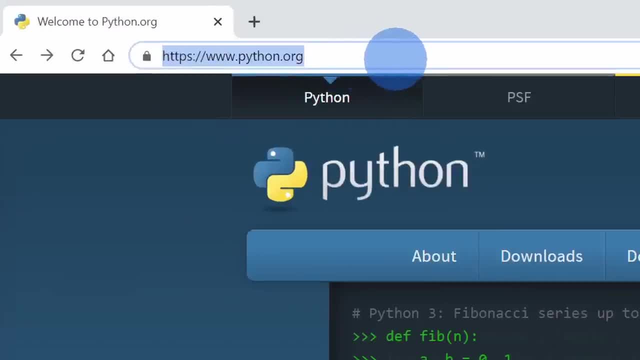 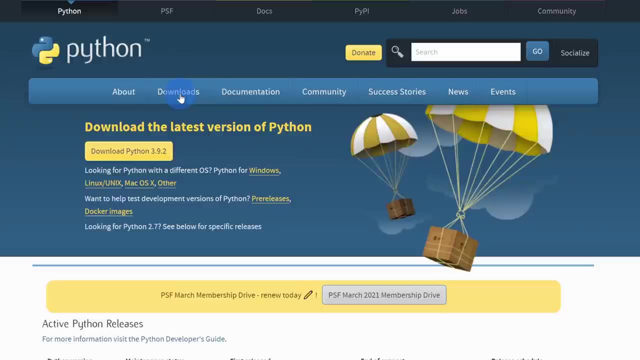 To get Python, head to the website pythonorg and that'll drop you on the Python homepage right near the top. You'll see a button right here for downloads. If you click on this, it'll identify what operating system you're on and it'll recommend the best option. 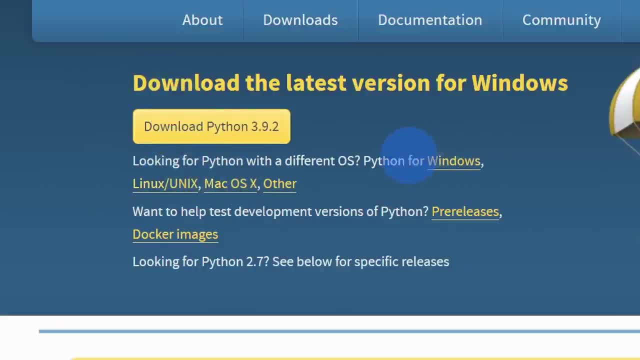 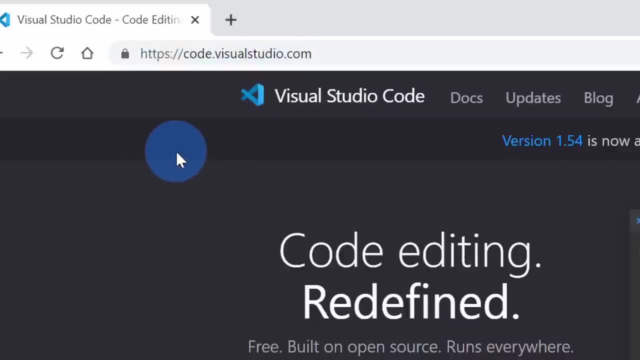 If you're watching this video, please make sure to hit that like button. If you're watching this video, please make sure to hit that like button. If you're watching this video, please make sure to hit that like button. And once you land on the home page, you can choose the operating system that you have. 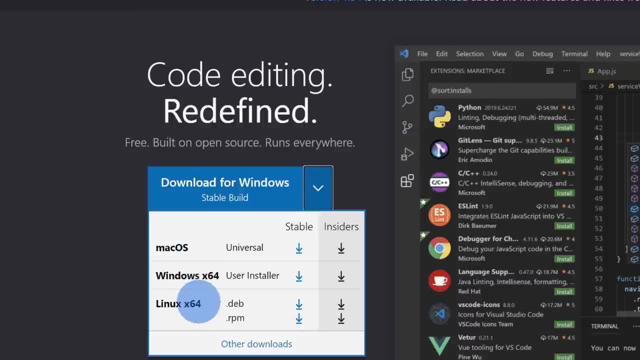 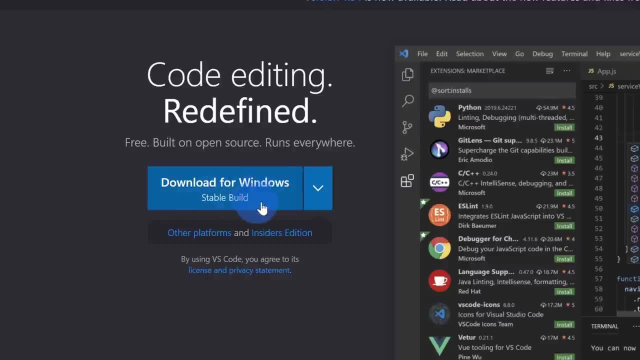 Here. when I click on the dropdown, you can get it on Mac, Windows or Linux, so it supports all of the different major operating systems. I'm running Windows today, so I'll click on download for Windows and I'll go with the. 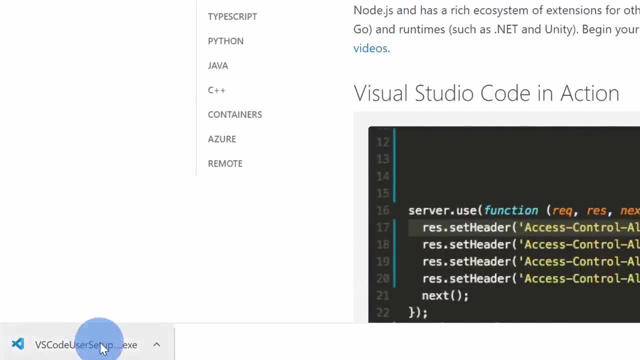 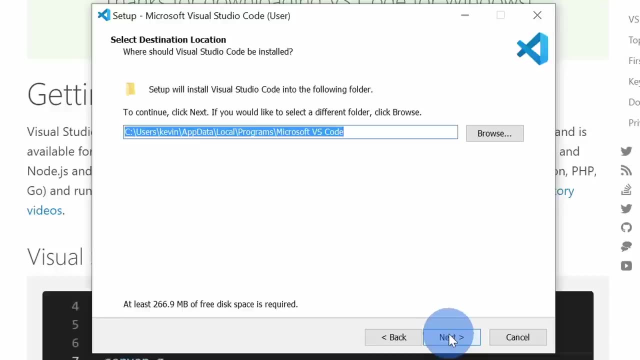 stable build. Once the download completes, down in the bottom left-hand corner, click on the exe. This opens up the setup process. I'll agree. I'll click to accept the agreement and then click on next. I'll go with the default location. I'll click on next. 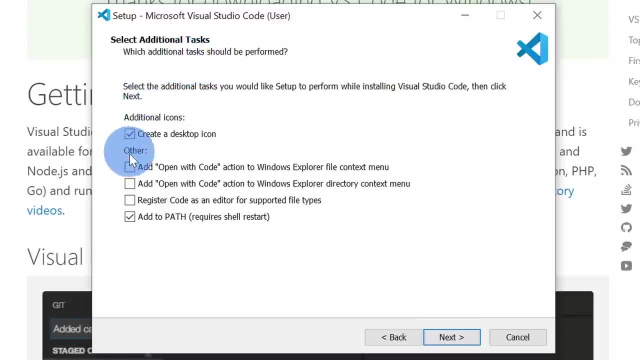 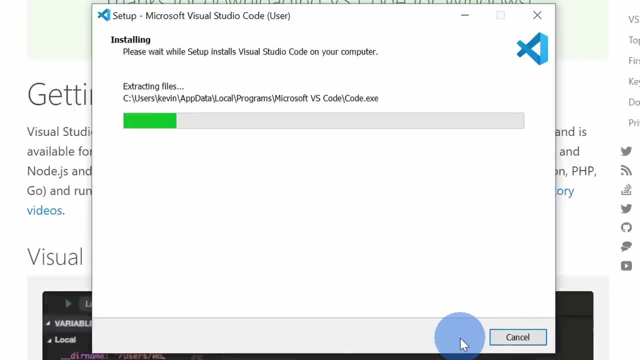 You'll then get a screen that says select additional tasks. I recommend checking all of these different boxes. Next, let's go down and click on. next, On the last screen, let's click on install. This will now go through and install Visual Studio Code on your computer. 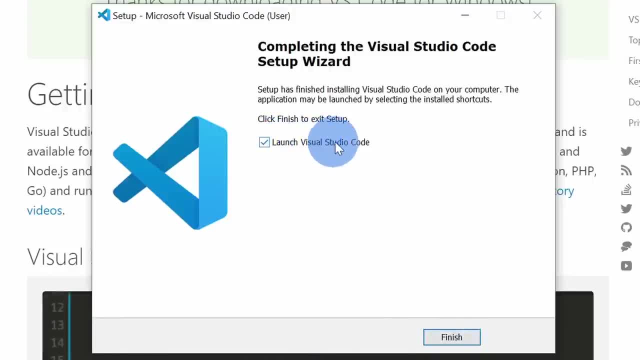 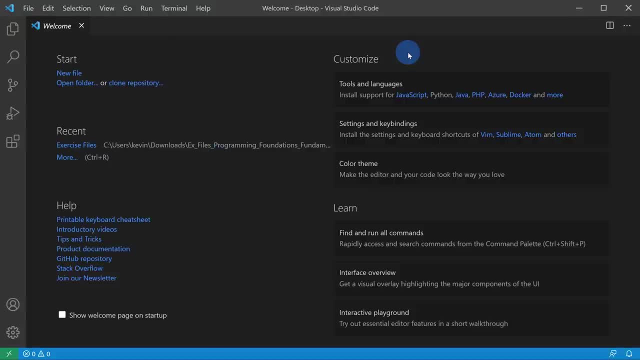 Once you're all done installing, let's click on finish and launch Visual Studio Code. This now drops us into Visual Studio Code and by default, we'll land on the welcome screen. If you ever want to get back to this screen again, you can click on the help menu and. 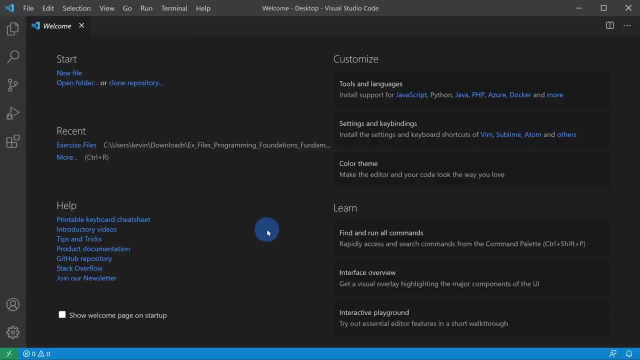 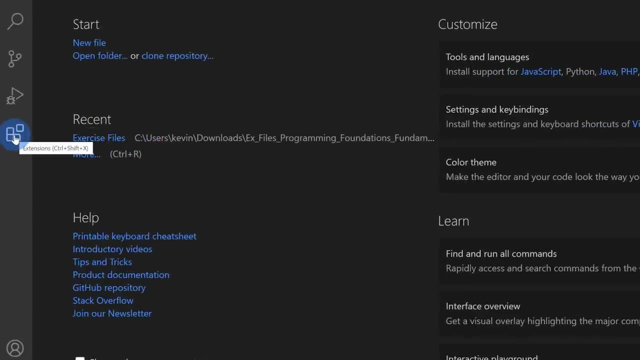 then click on welcome and that'll drop you right here. There are a few things we want to do before we can start writing code in Visual Studio Code Over on the left-hand side. there's an icon here for extensions. Let's click on that. 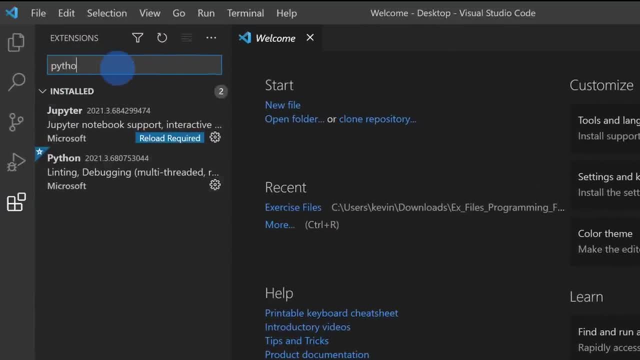 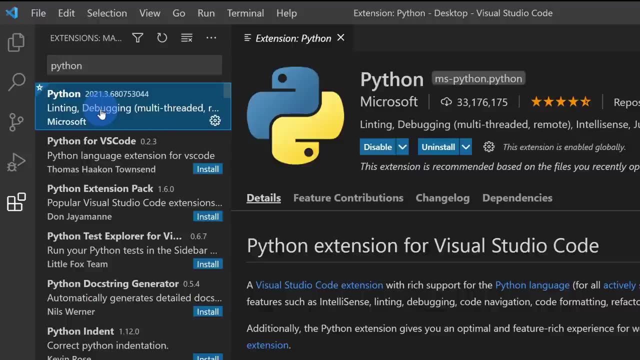 This opens up extensions and up here in the search field type in Python. We want to install the Python extension. When you type it in, you should see Python at the very top, and when you click on this you'll see that it's Python by Microsoft. 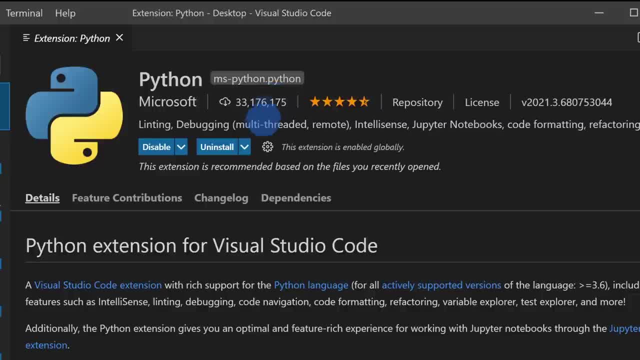 It should have something over 30 million downloads and right here, if you don't yet have it, you can install this extension. We're going to need this, so click on install and make sure you add it Once you finish installing the extension. we also want to select Python. that we just 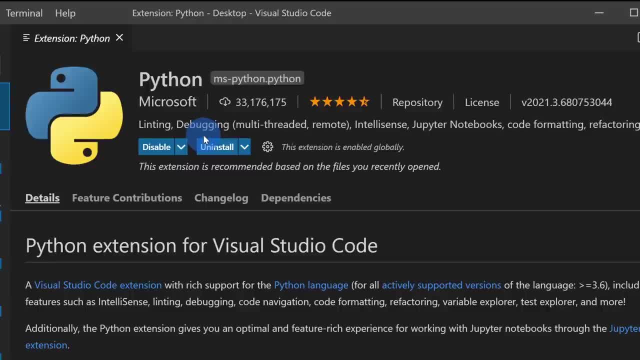 installed as the interpreter for Visual Studio Code, and this is really easy to do On your keyboard. press control shift and P at the same time. That's it. That's control shift and P, and that'll open up this screen right here. 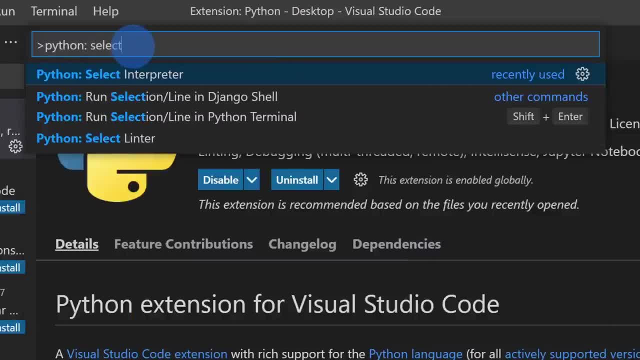 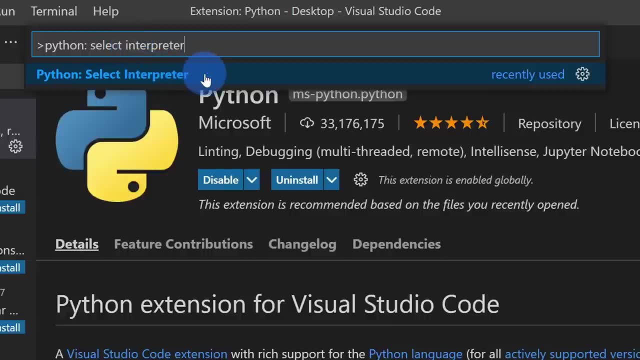 Up here, type in Python colon: select interpreter. This will allow us to select the interpreter that we want to use. If you remember in Notepad when we wrote our code, it interprets that code. so we basically want to tell Visual Studio Code what interpreter we want to use. so I'll select this option. 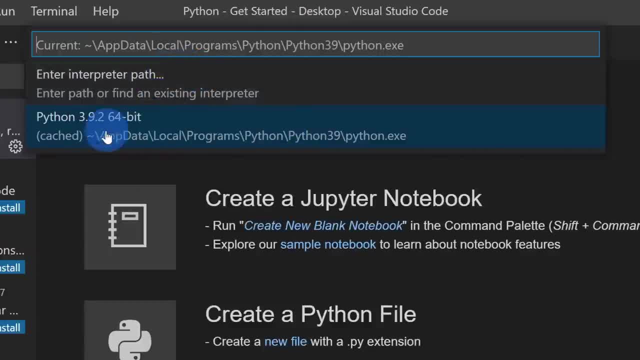 right here and now I can choose my interpreter. Here you'll see Python 3.9.2, so this is what we installed just a moment ago. so here I'll select this as my interpreter, and now we're all set to start writing code. 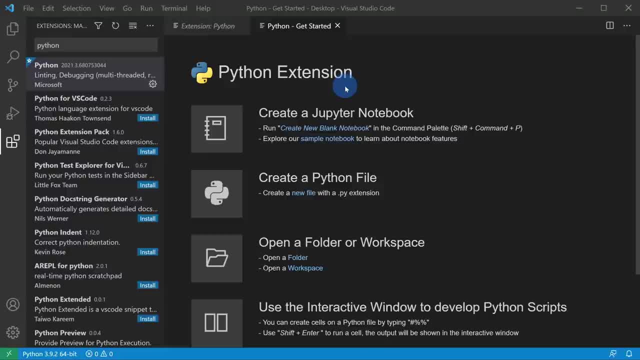 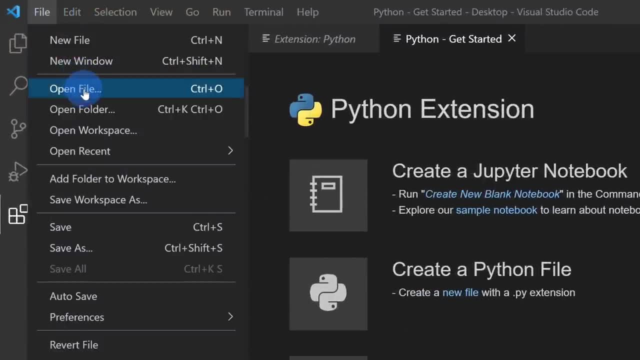 in Visual Studio Code To get started. why don't we open up the hello world file that we created previously Here? I'll go up to the file menu and I'll go to open file. This opens up my file picker and here on my desktop I see my hello world file. 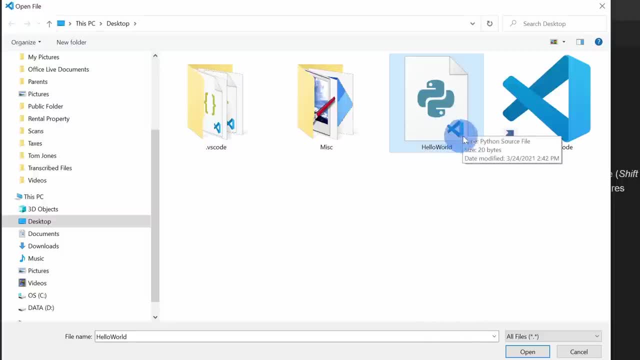 Here you'll also see that this type of file is not a file picker. It's a file picker. This file is now associated with Visual Studio Code. This is the Visual Studio Code logo. I'll select this file and then click on open. 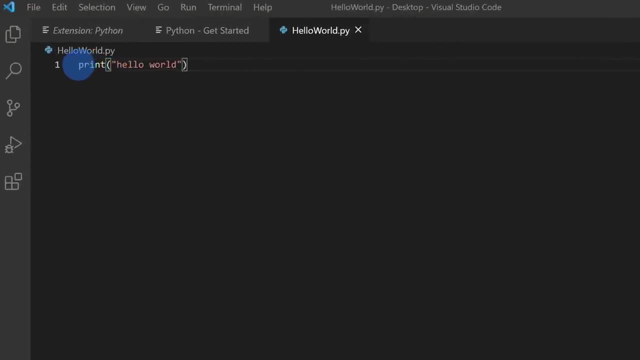 Now that I've opened the file, you should recognize this. This is exactly what we wrote into Notepad, except this time we have it open in Visual Studio Code. Now you'll start to notice some of the benefits of using an IDE or an integrated development. 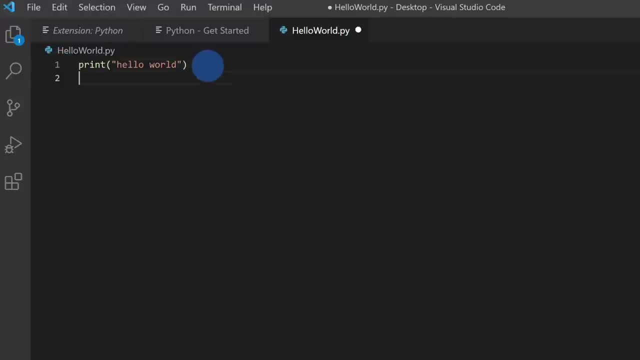 environment. First off, I have line numbers now. so here, if I add additional lines of code here, I get all of the line numbers over on the left-hand side In Notepad. we didn't get that. Also, when I write in this function called print, it highlights it in different colors. 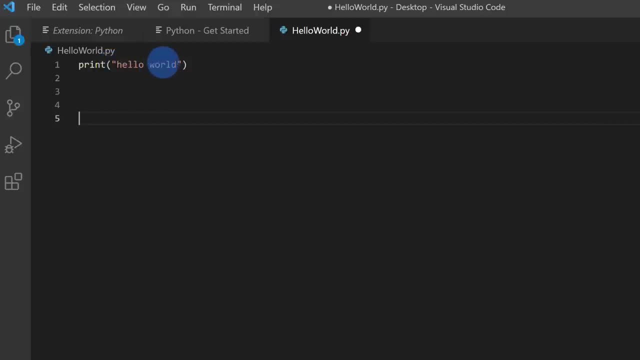 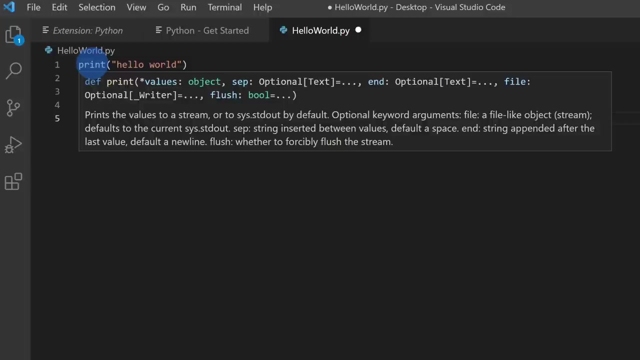 so I can identify what is the context or the text that it's printing and what is the function. so here I get different colors. Also, when I hover over print, it gives me some helpful suggestions on the type of content that I can enter within this function, so this will make it a lot easier as we start. 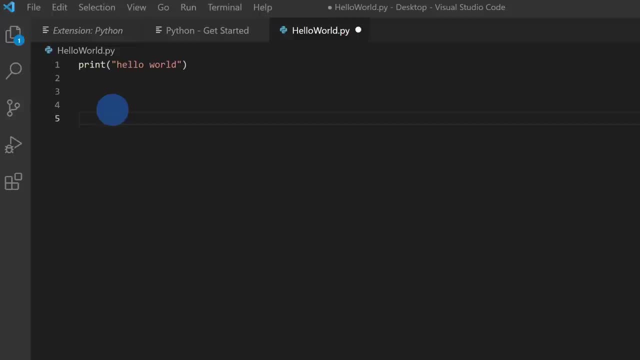 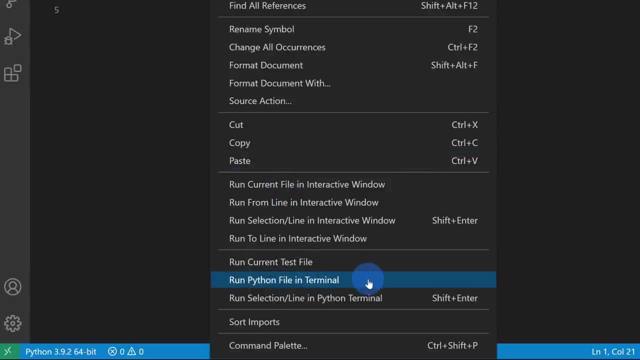 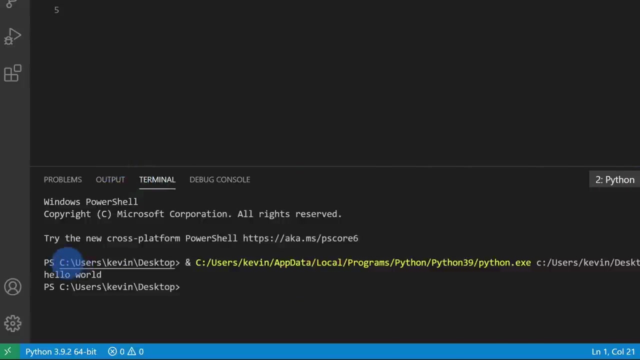 writing out our code. Now I can run this code directly in Visual Studio Code. I'll simply go up here and I can now right-click. Right down here there's an option that says run Python file in terminal. When I select that, it'll open up a terminal on the bottom of the screen and here I can. 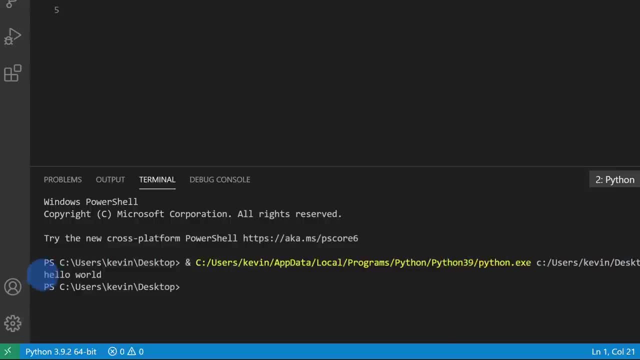 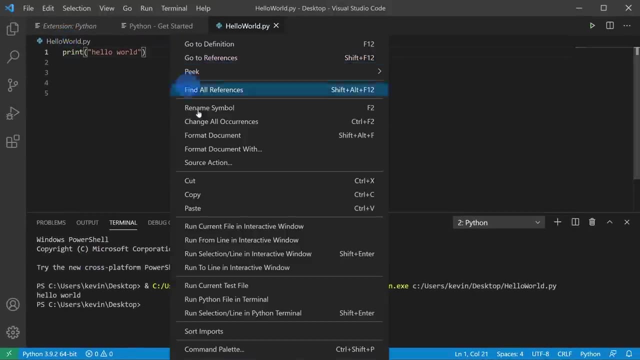 see that it executed or interpreted this file, and here it prints out: hello world. so it gives me the output of this code right up here, Along with right-clicking on the screen and running the Python file in the terminal. I'm going to run this code. 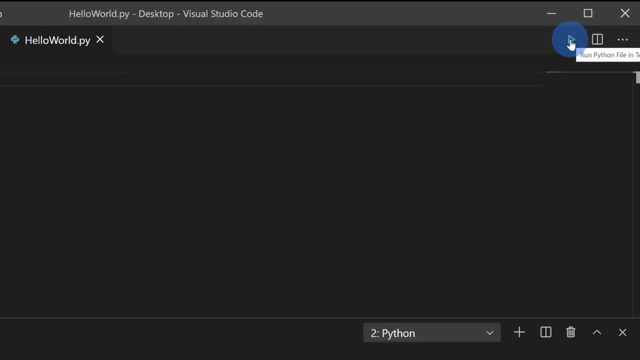 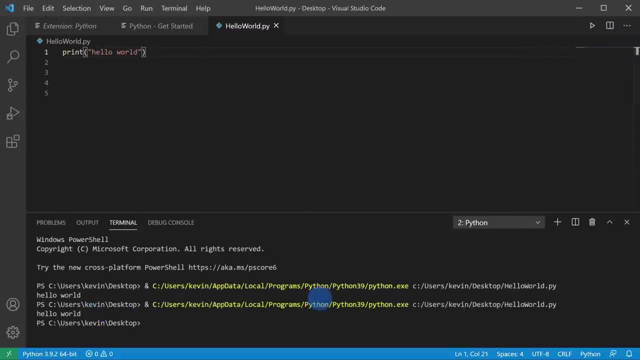 I can also go up to the top right-hand corner and I can click on this play icon. This will also run the Python file in the terminal. so when I click on this, here too it ran this file, and here too I see hello world. so this is just another way probably. 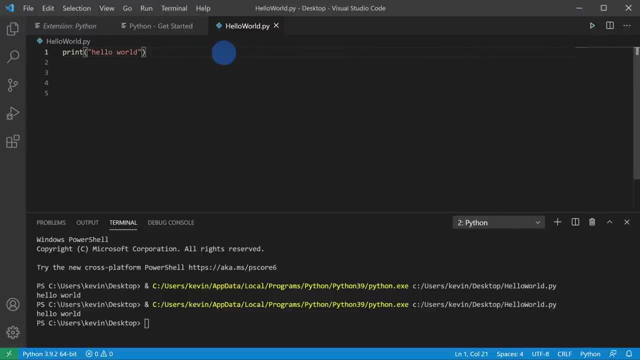 a little bit easier to see the output of your code Now that we know some of the basics of how to start writing code and how to run that code. I want to show you how we can start working with operators to work with numbers. 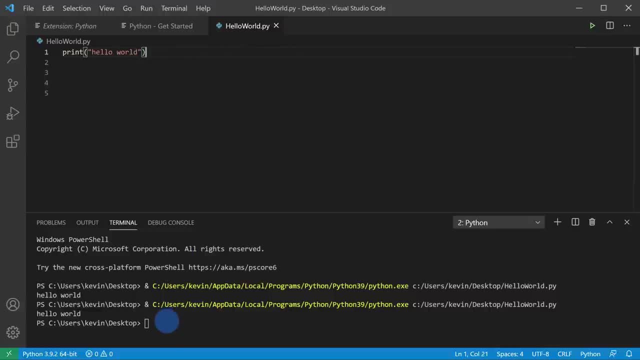 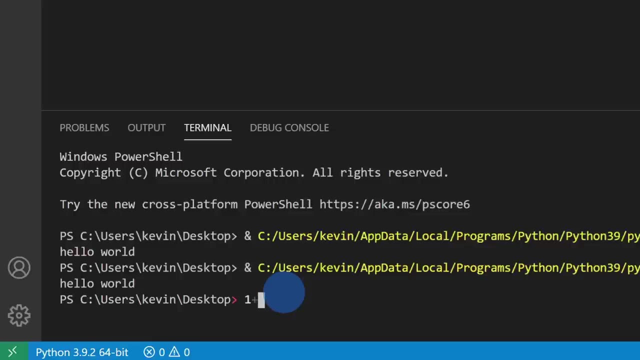 and here I'm going to type two. I'm going to type in two, so I want to do that as well. And then I'll go down here to the terminal and, just like we did earlier in the Python terminal, I can type in here. so here I'll type in one plus two and I'll hit enter. 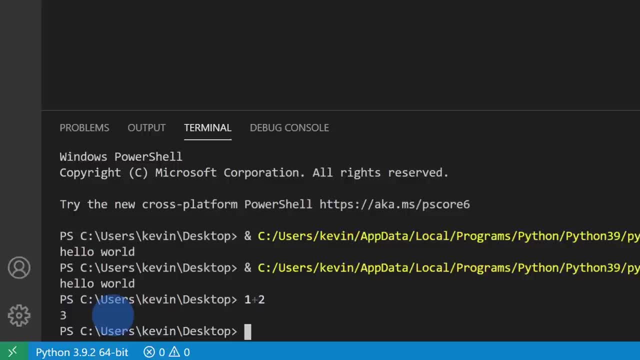 and here it interprets that code and it evaluates it to three. so, just like we saw earlier, One of the things is, you'll notice, when I typed in one plus two, I didn't include any spaces, and spaces or white space don't impact the calculation at all, so I could also type 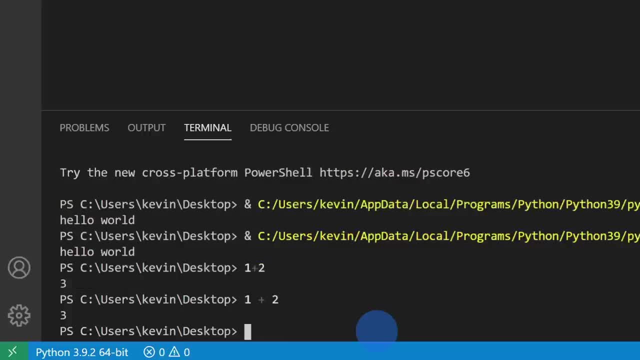 in one space, Yeah, and then hit enter, And there too it also evaluates it to three. So using white space can actually make your code more readable. So you could type it in like this or just include some white space. It won't affect what the outcome is. With Python I can use all of the standard. 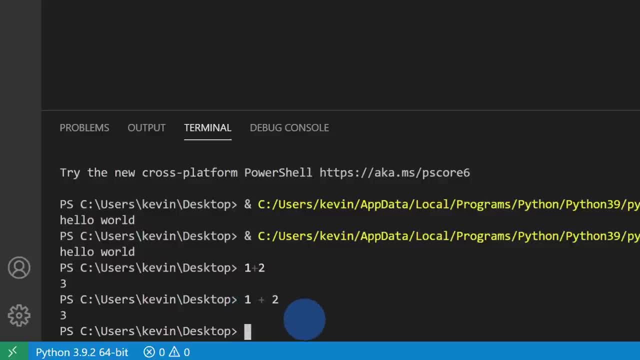 operators. Right up above I showed you how you can do addition, but here let's say five minus two. I can also do subtraction, and there it evaluates that to three as well. I could do multiplication, So let's say four times four. Now with multiplication I enter in an asterisk. 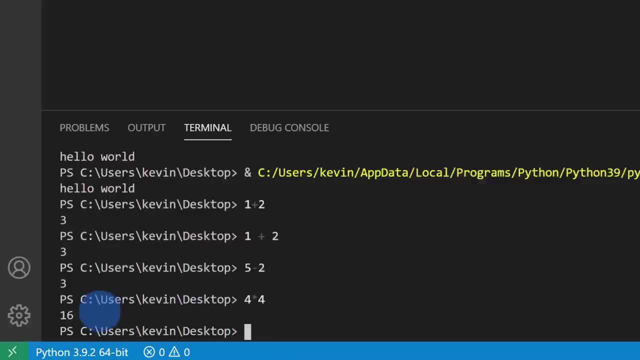 That's the multiplication symbol. Here I'll hit enter and it evaluates that to 16.. I could also do division. Here I'll take 10 divided by five, And here for division, division is the forward slash, And then I'll hit enter and that evaluates to two. Now with Python, let's say that you start. 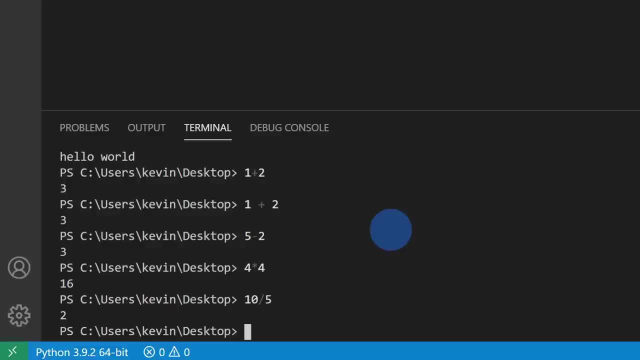 using multiple operators. So maybe you're adding and then you're multiplying. Python follows the default order of operations. So let's say: let's say that you're adding and then you're multiplying multiple operators. So let's say that you're adding and then you're multiplying. So let's say: 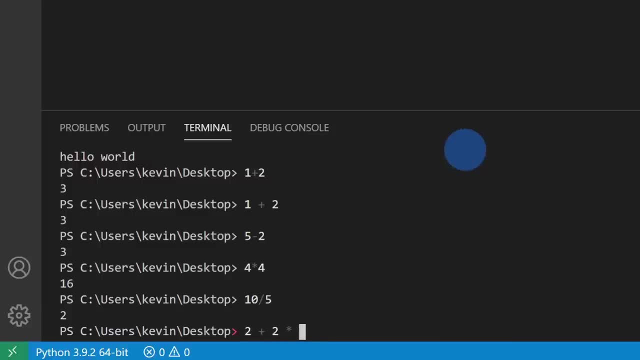 enter in two plus two, and then I want to multiply by five. What do you think this will evaluate to? Is it two plus two, which is four, and then times five, which is 20?? Or is it two times five, which is 10, and then you add two to that which is 12?? Well, here, if I hit enter, 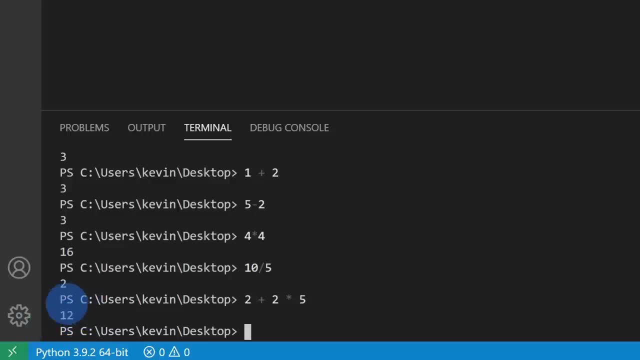 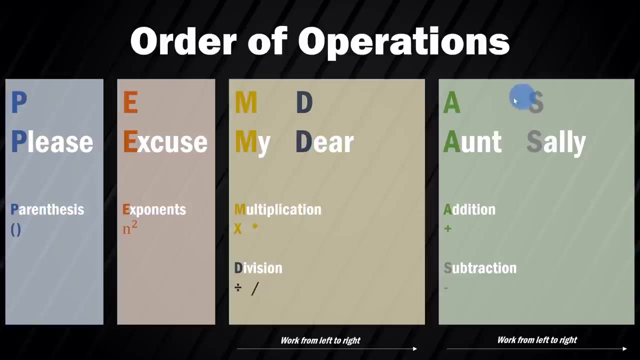 it evaluates to 12 because it's following the default order of operations. Multiplication comes before addition. If you've ever heard PEMDAS- or- Please Excuse My Dear Aunt Sally- before, that's how you know what's going on. So let's say that you're adding and then you're multiplying. 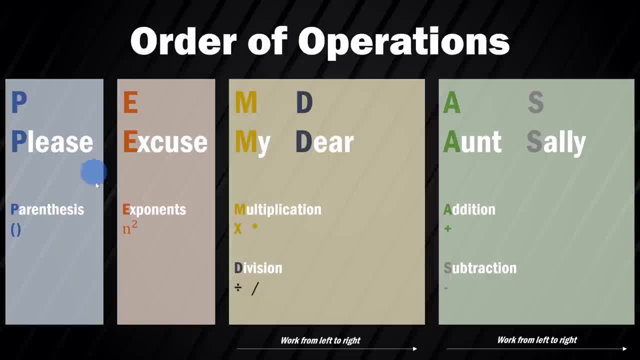 multiple operators. So let's say: let's say that you're adding and then you're multiplying multiple operators. So let's say that you're adding and then you're multiplying what the order of operations is: First it'll evaluate whatever's in parentheses, then it'll look at any exponents. 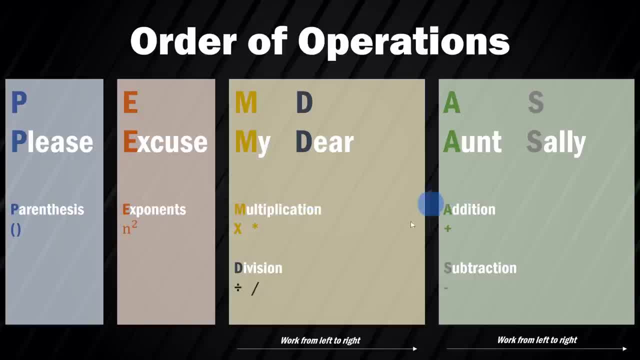 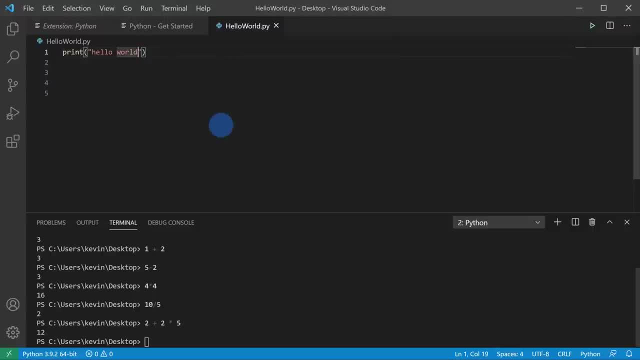 followed by multiplication and division in the order of left to right, and then it'll look at addition and subtraction, also in the order of left to right. Up above I could also enter in my expression up here. So here I'll get rid of hello world, and here I'll say: let's print out two plus. 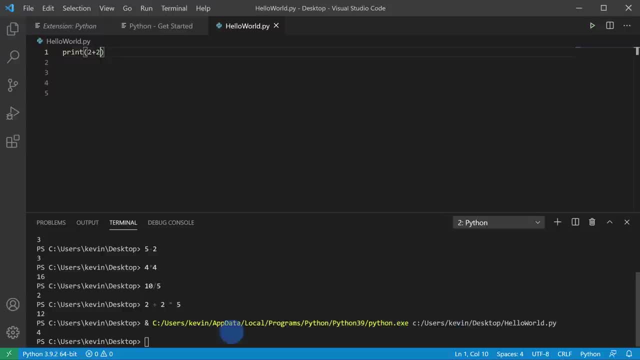 two. Here I'll click on run and here you'll see that it executes this code and here this also evaluates to two plus two. So let's say that I'm going to print out two plus two, and here I'll to four. If I want to use an exponent, I'll come up here. let's remove the plus symbol. 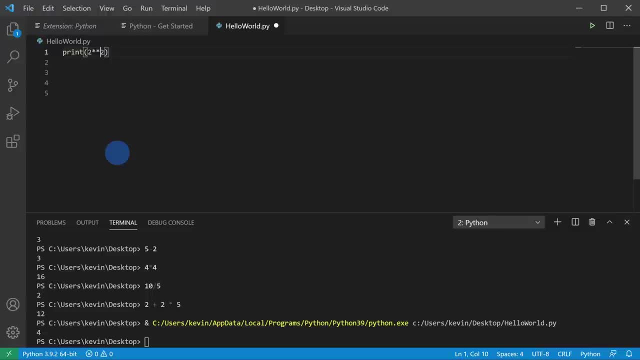 and here I'll enter two asterisks. So this will be two to the power of two. And here, if I click on the play button here, that evaluates to four. Two times two is four. But let's say I want to do a two to the third. Here I'll evaluate and it comes out to eight. I also have access to the. 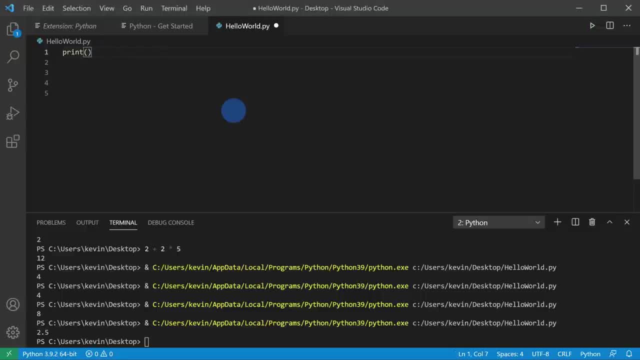 floor operator. So let's take an example here. Let's say I want to calculate five divided by two, and here I'll, And right down here I see that's 2.5.. So I have a remainder of 0.5. But let's say I don't want to. 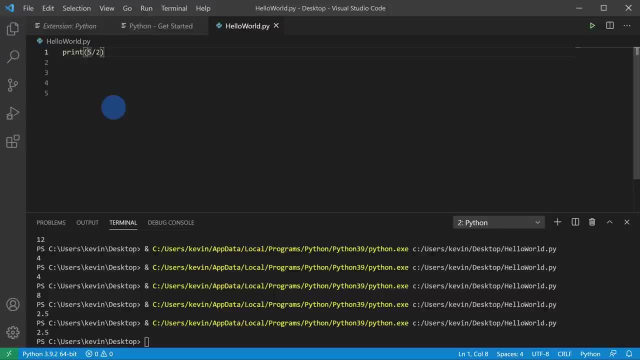 know what the remainder is. I just want to know how many times it goes in without a remainder. This is also known as the floor. I could insert another forward slash and then I could run it, and here it tells me that it's two. But let's say, I just want to know what the remainder is. I can. 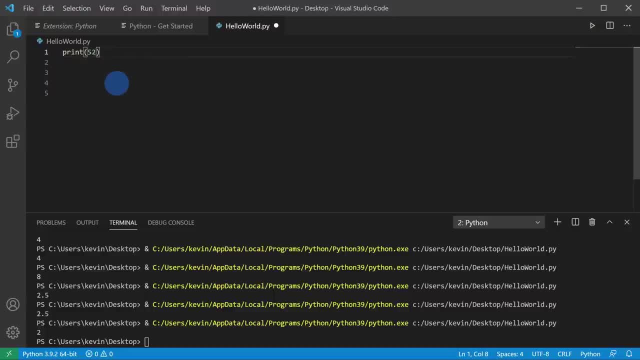 use the modulus operator for that. I'll get rid of the forward slashes and right here I'll type in the percent symbol, Then I'll hit go, And here I'll type in the percent symbol, And here I'll hit go. And here it tells me that the remainder is one, As I'm entering in numbers up above. 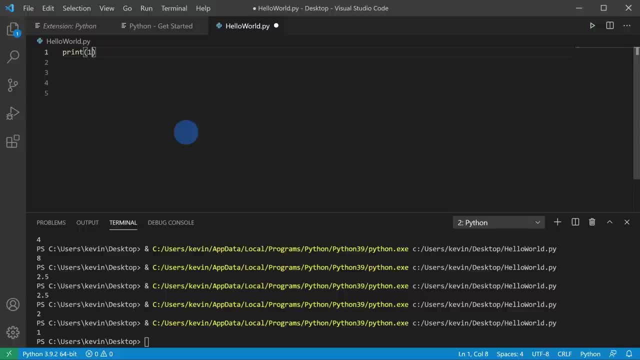 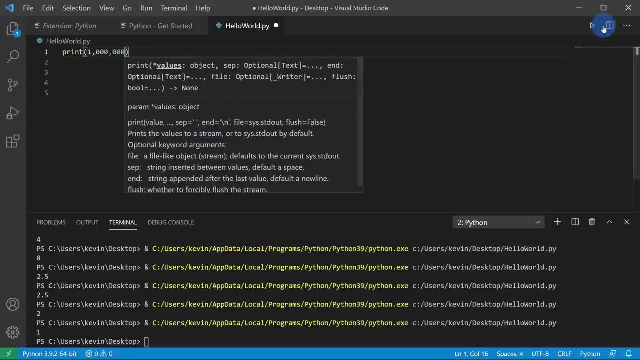 and as I'm working with numbers, let's say that I enter a very large number, So let's say I enter in maybe one million. Now I could go through here and I could enter a comma and then I'll type in the zeros And if I hit go here, you'll notice that it doesn't print what I expect it to. 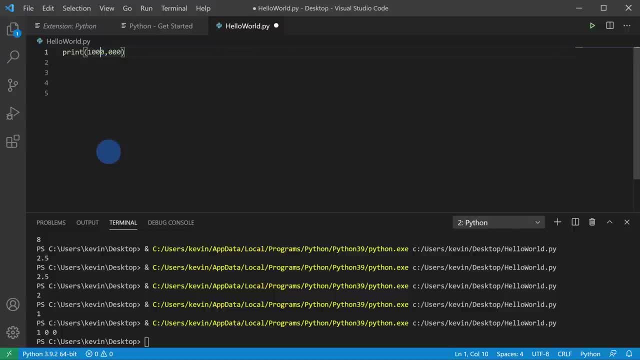 That's because we don't want to use commas as we're entering numbers. Instead, when you enter a number, just enter it in as is and then hit go And here it prints exactly what I want it to print. So you don't want to use commas when you're entering in numbers, Now that we've entered in. 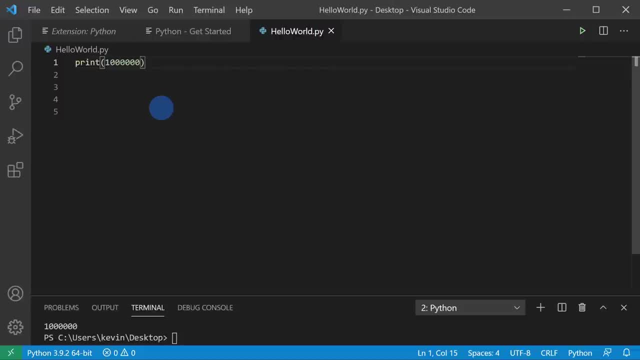 some numbers and we know a little bit about the basics of how you can work with numbers and operators. let's start working with some text, or what's referred to as strings. Let's say that I want to print what's up Now. earlier we printed out hello world, and it's the same concept here. 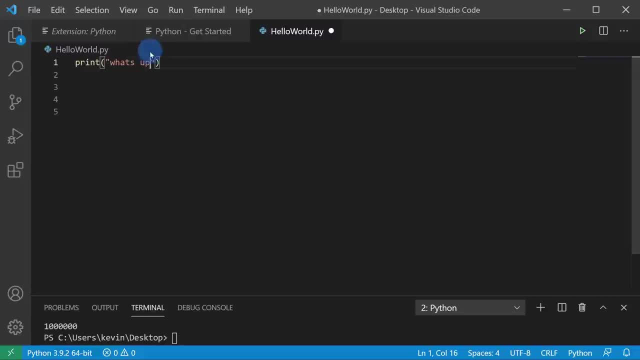 I'll insert in double quotes and then I'll type in what's up. So here's what's up, and I'll click on this play icon and down below you'll see that the output is what's up. Now I surrounded what's up. 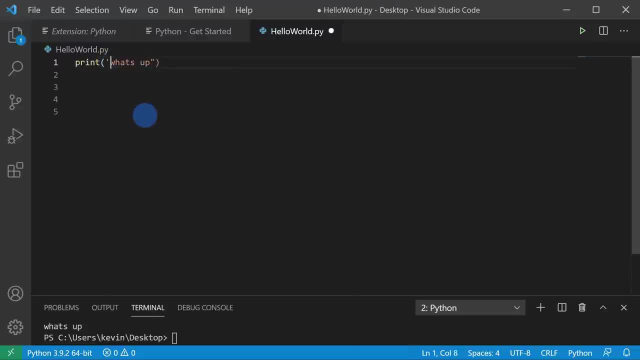 with double quotes. Now, instead of using double quotes, I can also use single quotes up here. So if I enter in single quotes and then hit play, here too, you'll see that I get the same output. So I can choose whether I want to use double quotes or single quotes. So why would I want to use one? 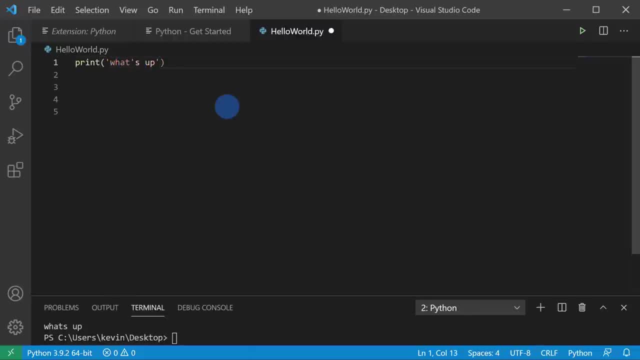 versus the other. Well, here, what's up should actually have a single quote, So I'll insert a single quote there. Now, one of the problems is, when I enter a single quote here, it thinks that this is the end of the string, And so now, if I try to run it, I get a syntax error down below. 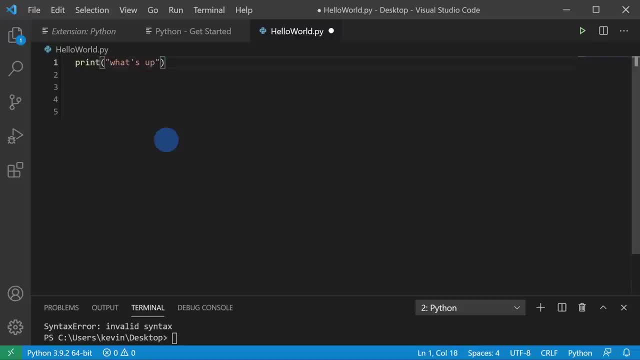 So instead I can use double quotes here, and I'll use double quotes at the end, and I could use a single quote in the middle, And then here I'll run it, and it works properly. Now, let's say you wanted to use double quotes within your text. Well, you could surround it with single quotes. 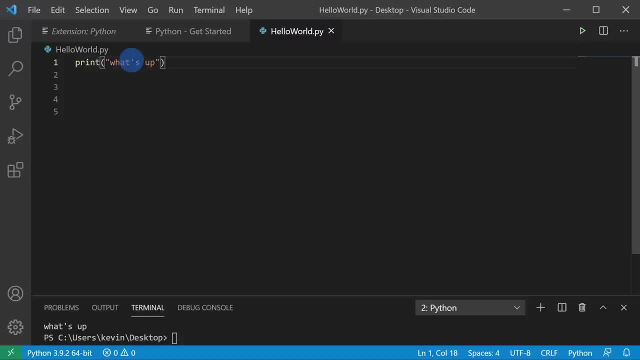 and that way the double quotes would show up Now here too, just like we saw before. white space doesn't impact how the code runs, So if I want to insert a space here and maybe insert a space there and another space here, and I run this code here, you'll see that I get the exact. 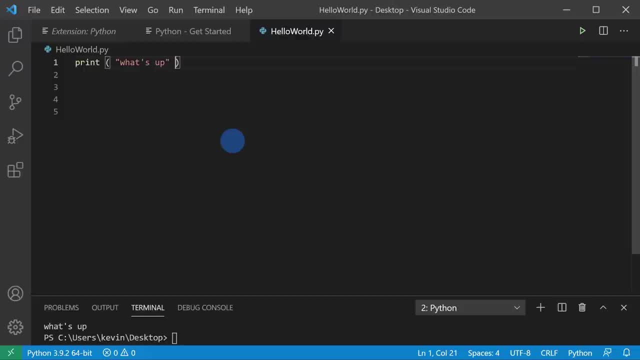 same output. So, once again, by using white space, that can help make your code more readable as you're going through. We now know some of the basics of working with numbers and also strings, but what if you want to make sure you explain what's happening in your code? How do we do that? 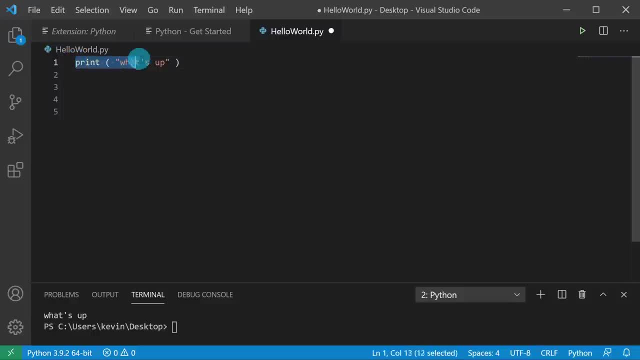 Well, we can use something called a comment. So let's say that I have this code here and I want to explain to someone what this does Here. I'll bring this code down to the second line and I can insert a comment by entering in: 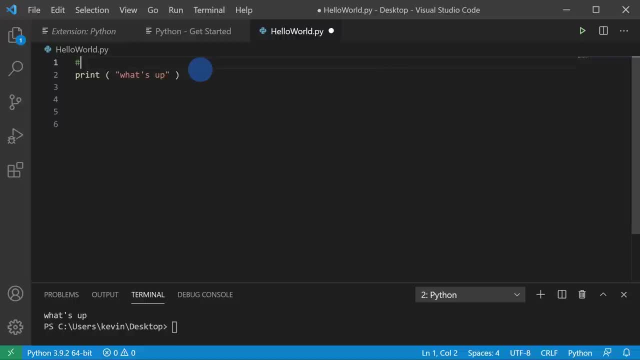 the hash symbol or the number sign or the pound symbol. So I'll enter that and here I can say: this prints some text. I've now typed in my comment and let's run this now, and here you'll see that this doesn't affect. 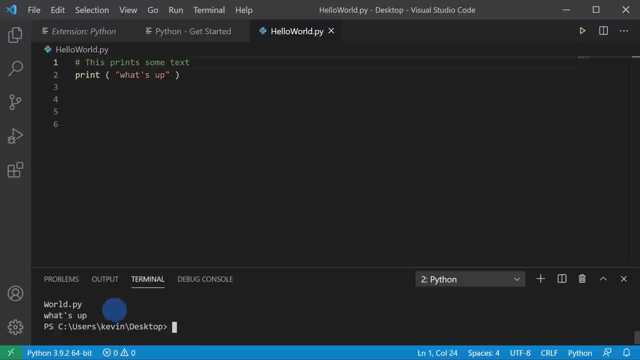 at all what appears down here. I simply get what's up. So, just like we got before, Now I could also take a comment and I could put it on a line with code. So here I'll put it. after my code, I'll hit run, and here too, you see that it just gives me what's up. Now one of the neat. 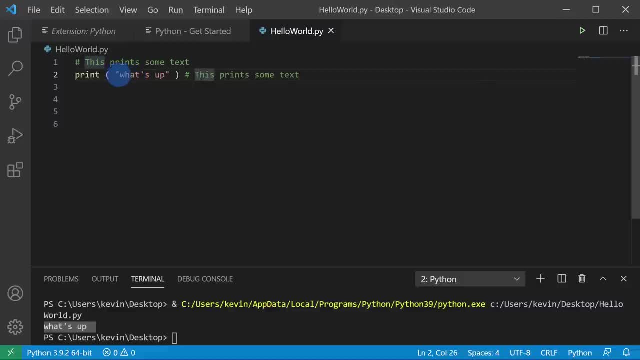 things is. let's say, I start writing a lot of code and it's starting to get fairly complex. I can comment out a line of code. I'll put the hash symbol in front of my code and, here you see, it turns green. So this is the IDE's way of telling me that this is a comment. 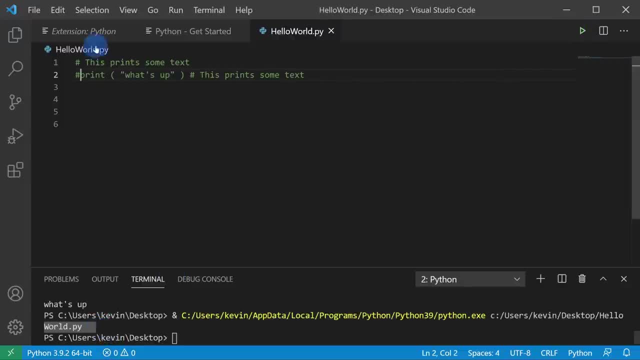 and here now, if I hit run, you'll see that I get no output. That's because I commented out this line of code, So here I can bring it back by removing it. and now here, if I run it once again, it shows me what's up. So comments are pretty valuable as you're writing code. 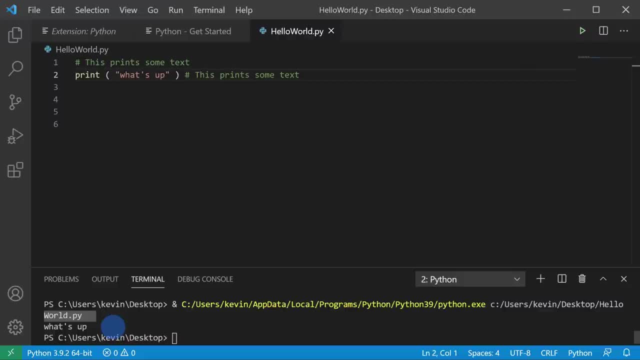 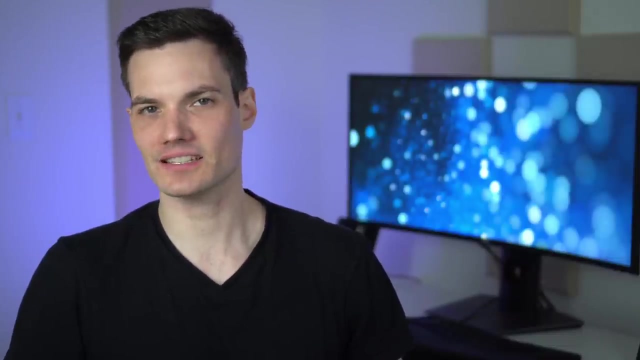 not only to let other people know what's happening in your code and what different blocks of code do, but you can also use it when you're troubleshooting to cancel out certain areas of your code until you're ready to test them again. Next we're going to look at how you can use variables and the easiest way to explain. 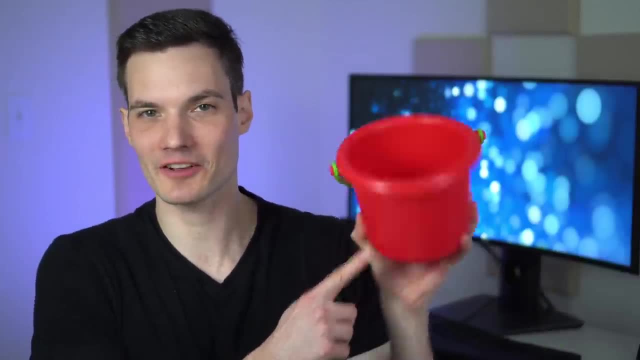 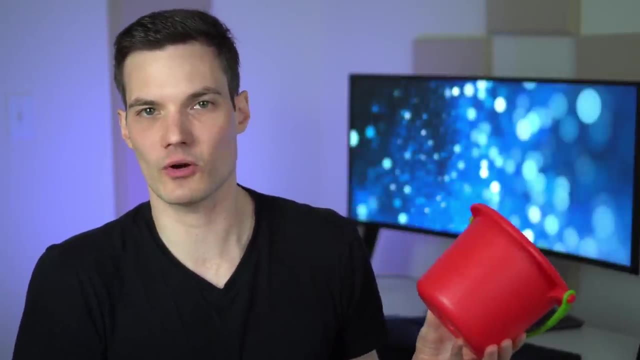 a variable is to use this red bucket that I have here from my son. So let's pretend that this red bucket here is a variable and we can name the variable. why don't we just call it red bucket, just to keep things simple? 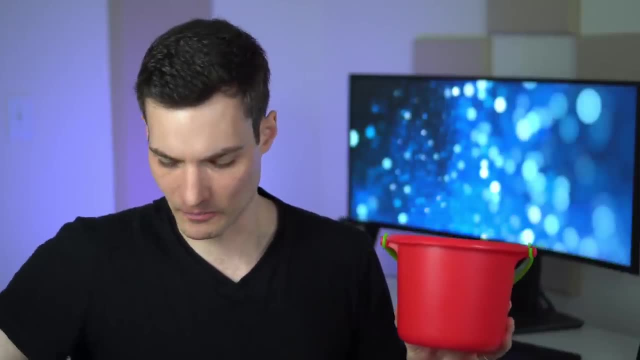 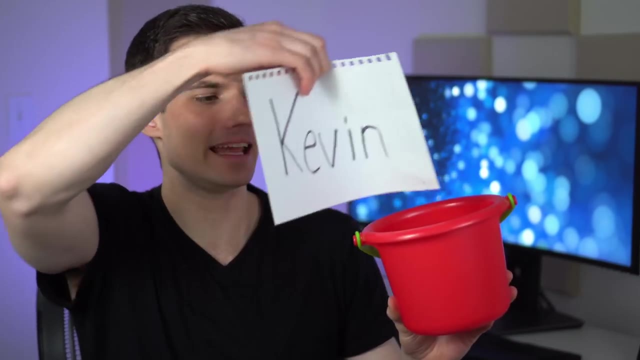 Now I can assign a value to this variable. So let's take, for instance, let's say I want the red bucket to equal my name, Kevin. So here I have my name, I can take this value and I can assign it to this variable. So now, if you say, well, what is the red bucket? Well, right here. 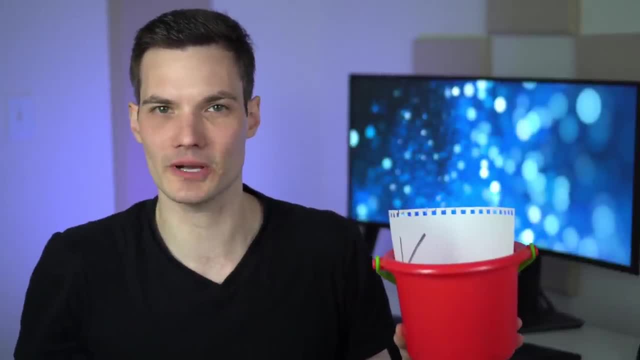 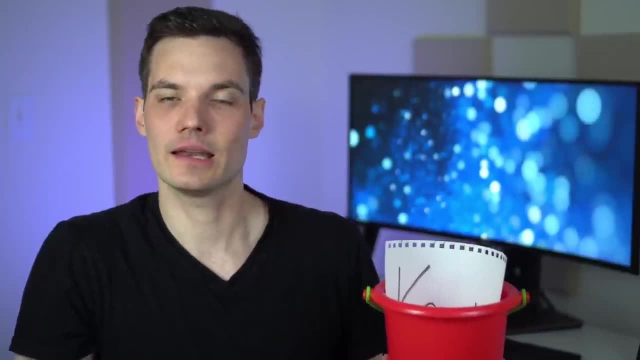 bucket is currently Kevin, So once again, I've assigned that value to it, and this is a string, or basically my name is referred to as a string. It's just a set of characters. Now I could assign other types of data to this variable as well, So maybe I say well, actually. 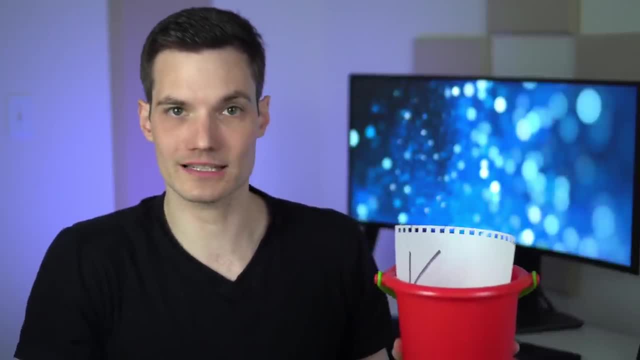 I want the red bucket now to equal a number, so maybe I want it to equal the number 8.. So I'm going to say, red bucket, you're now equal to 8, so I'm going to take my name, we're going to. 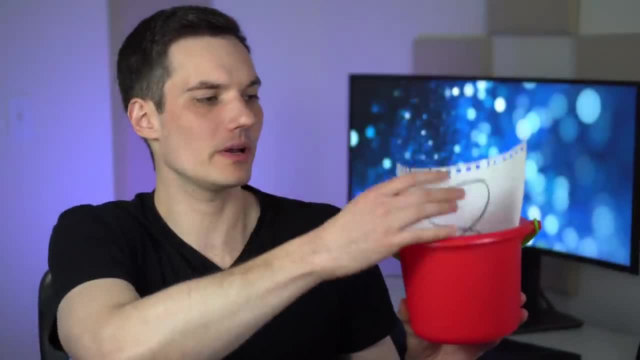 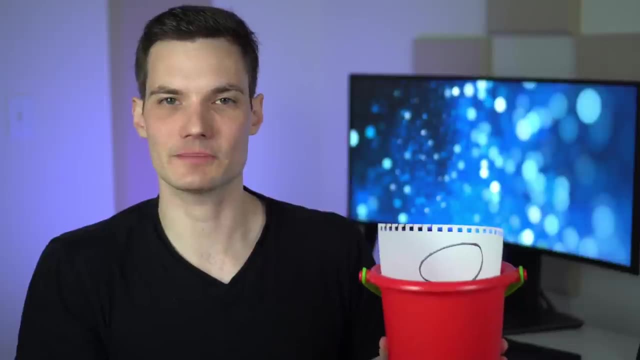 pull that out, and here I'll take the number 8 and we'll put it in the bucket. So now, if you ask me, well, what is the red bucket? Well, it's currently the number 8.. That's a general concept of a. 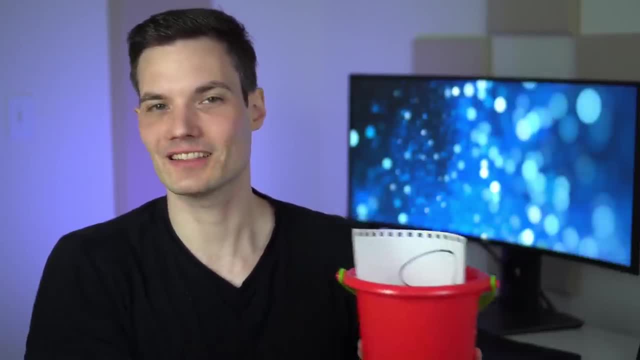 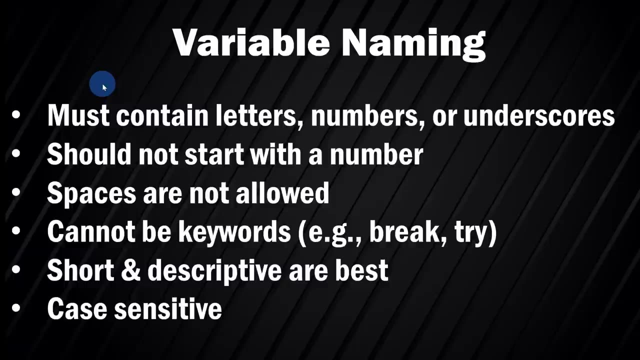 variable. The variable can hold different values. Let's jump in now and see how we can use variables To create variables. there are some rules that we need to follow. This is the syntax that Python looks for. A variable should only contain letters, numbers or underscores, And. 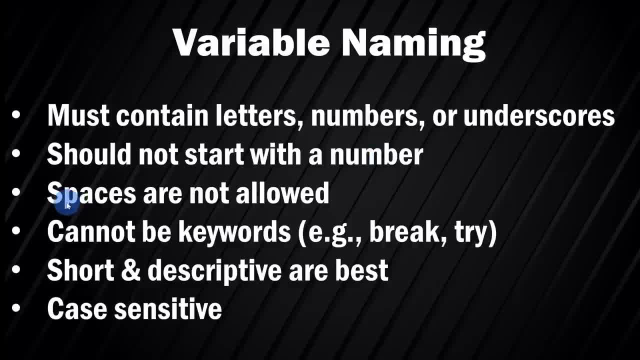 also. we just need to make sure that we don't start with a number. We can't use any spaces in a variable name. We also can't use any known keywords to Python, like break or try, And ideally we want to make sure that a variable name is short and descriptive. Those work best. 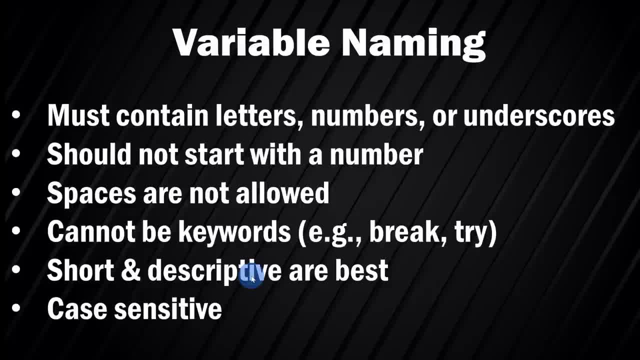 So, for example, with the red bucket- well, that was simply called the red bucket, So it's pretty short and also descriptive. Also, variable names are case sensitive, So if I wrote red bucket with a capital R and another one with a lowercase r, Python would view those as separate variables. 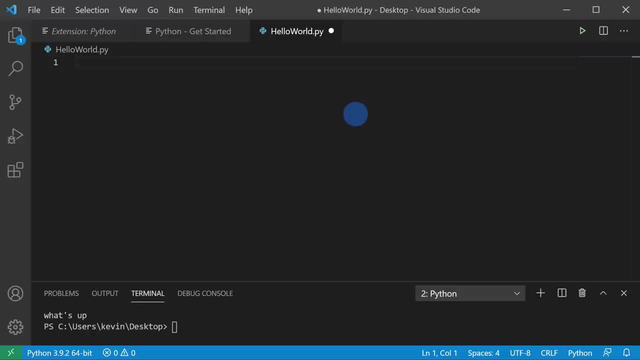 So case sensitive, sensitivity matters, Okay. so let's create our first variable And, just continuing the example, let's say I want the variable to be called red bucket, So I'll give it this name. And now I need to assign a value to this variable, just like I did with the bucket, So I'll type in red bucket. 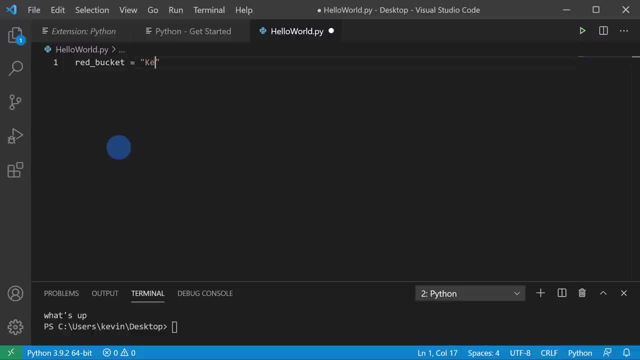 and then I'll type in the equal sign and I'm going to assign it the value of Kevin, my name, And here I'm using just a single equals sign. So what this does is it will assign this value to this variable. So now here I could hit enter and let me run this, And here nothing shows up. yet 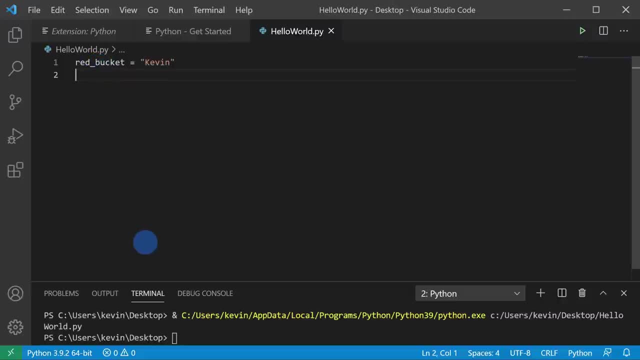 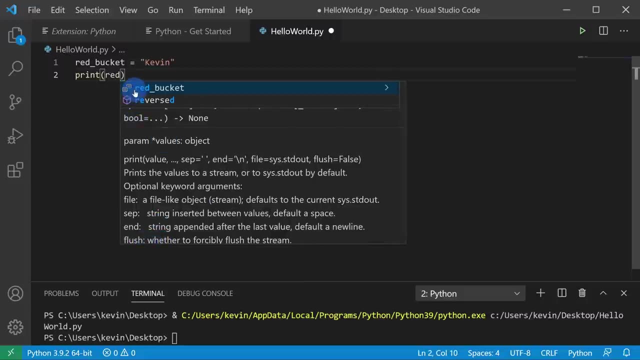 because I've assigned this value to this variable. The next thing we could do is actually print this out. So here let me say print and let's type in red bucket. What's nice is because I'm using an IDE. it recognizes that I created a variable called red bucket and I could just click on it. 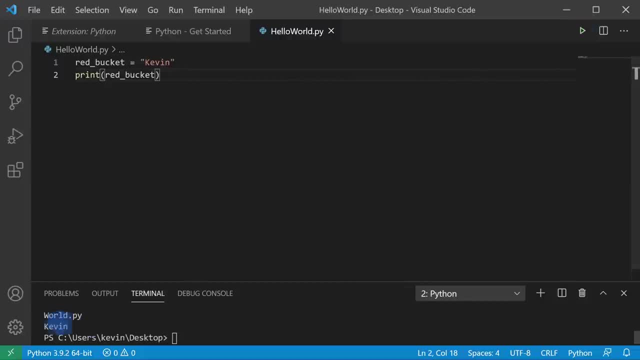 here. Now, if I click on the play icon here, it'll print out Kevin. So it's printing out the value that Kevin assigned to the red bucket. Now let's take another example here. Let's say I add another line and let me copy this first line and I'll paste it into the second line. 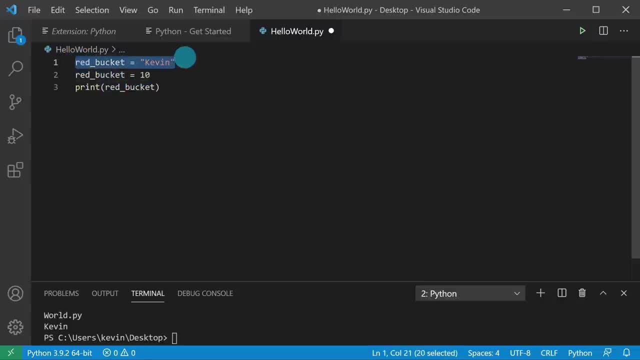 And here I want to assign 10 to the red bucket. So here I start out by assigning Kevin, then I assign 10.. What do you think will print out? Let's click on the play icon and here it prints out 10.. And the reason why is: well, first it assigns Kevin to red bucket, and so that's the. 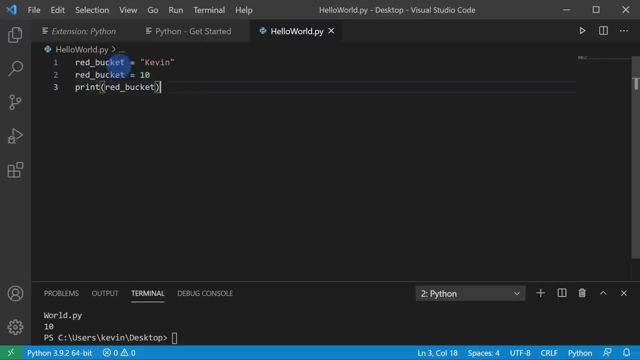 current value. But then on the next line of code it assigns a 10, to the red bucket. So the 10 overwrites Kevin. And then when I print out the red bucket, it's taking the last value that was assigned to it. So the way to think of this, back to the bucket. 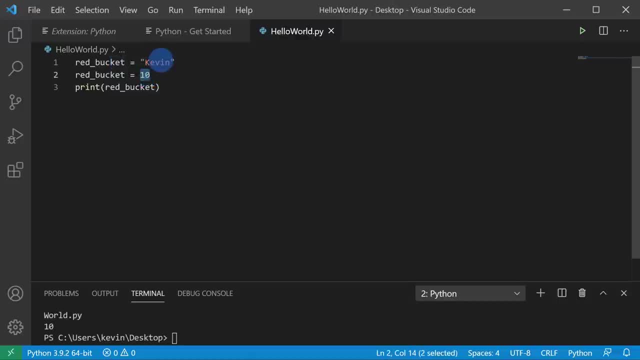 example is I put Kevin in the bucket And then, when I put 10 in, I have to take Kevin out and then I put 10 in. So at the very end, when you ask, well, what's in the red bucket? Well, the 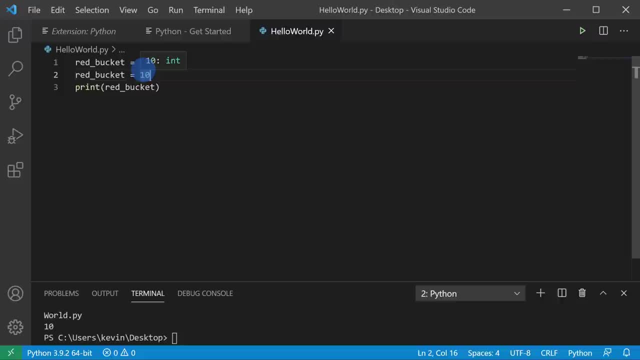 number 10 is in the red bucket because that's the last item that I put in. One thing that's really neat about Python is when you're defining your variables, you don't have to assign your variable a type. So here, for example, for the red bucket, I assigned it my name, and that's also known as. 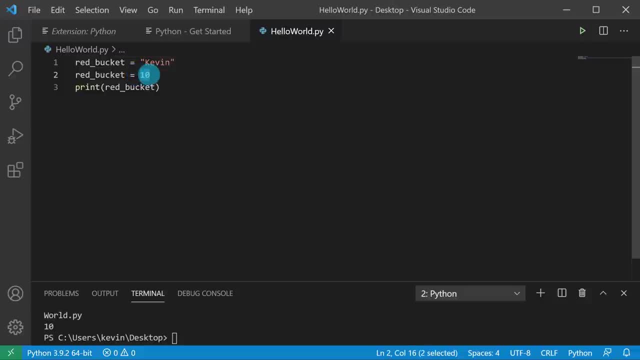 a string And next I assigned a number which is an integer. but I don't have to go and say, well, the red bucket is a string or a red bucket is an integer, It'll automatically know what data type that I'm assigning to that variable. So down here in print I can type in type: 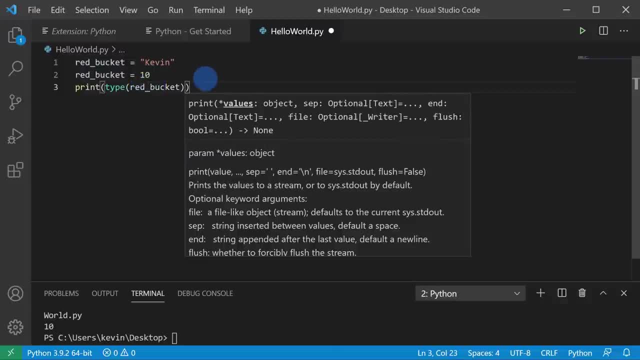 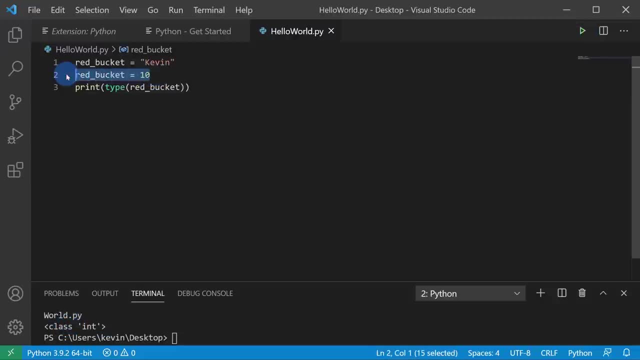 and then I'll open and close the parentheses around this variable. And so now let's run this, And here it's telling me that it's an integer. So basically, here 10 is assigned to red bucket. And so it's telling me: 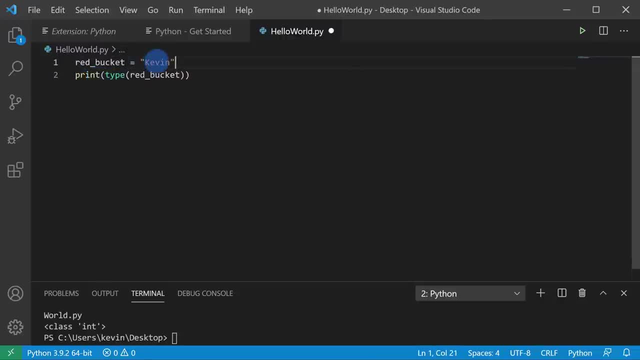 that that's currently an integer. Let's get rid of this line right here. So now Kevin will be assigned to red bucket, And when I run this here, you'll see that a string data type is assigned to this variable. Now let's say that I want to get rid of a variable, So maybe I don't have a need. 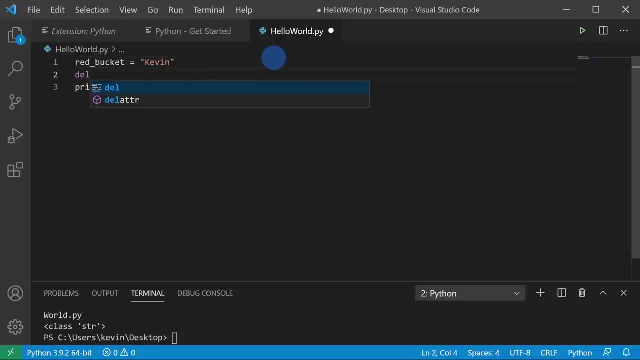 for the red bucket anymore. Down here I can type in D, E, L, Basically delete, and this will delete a variable. And here I can type in red bucket again. I'll select the suggestion. Let me get rid of the type in the print. So I just want to know what is red. 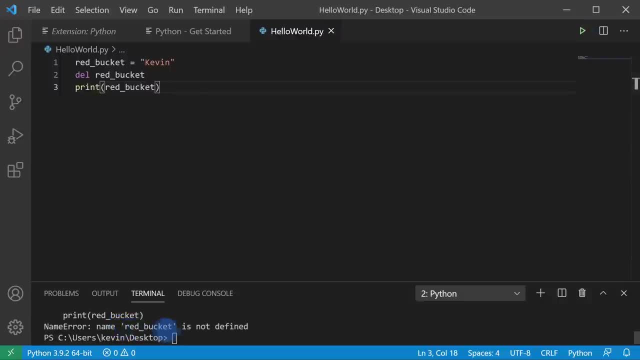 bucket. So if we run this now, I'll get an error because it says red bucket is not defined. And that makes sense, because here I created the variable, I assigned a value, here I deleted the variable and here I try to print the variable but there is no variable anymore called red bucket. 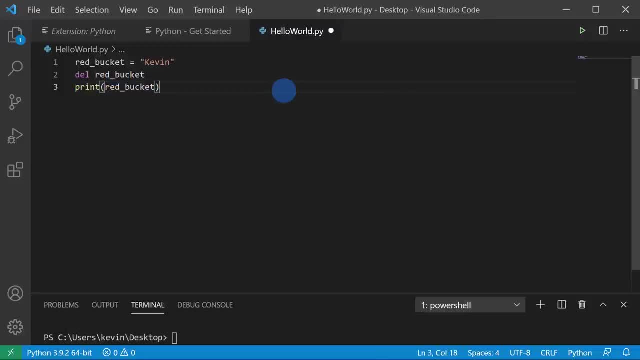 because I deleted it right up above. Next, I want to show you an example of how you can request input and then you can take that input and assign it to a variable. So, right here, I simply typed in Kevin and I assigned it to this red bucket. but I want to 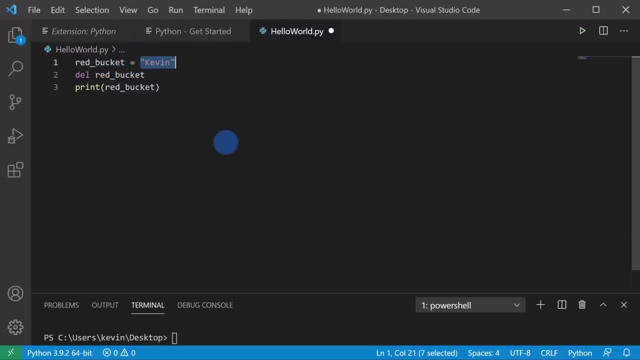 allow input. So right up here let's delete Kevin, or delete your name that you entered in, And here we'll type in the input function. Here I'll open the parentheses and let me type in double quotes and maybe I'll ask the question: what do you want to put in the bucket? I'll enter a question mark. 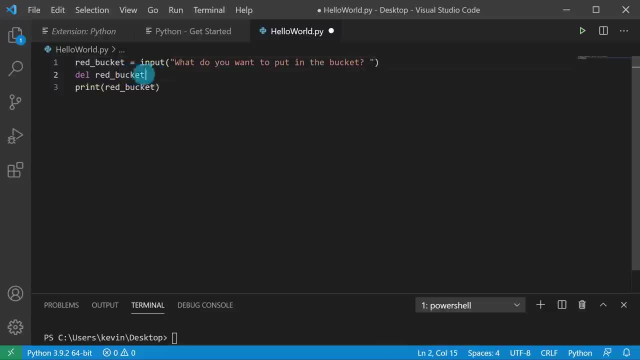 and then an additional space Now right down here. delete the variable. So I'll get rid of this. So right now I'm going to ask for input and then we'll print out whatever the input is. So here let's click on the run icon and this will run it. 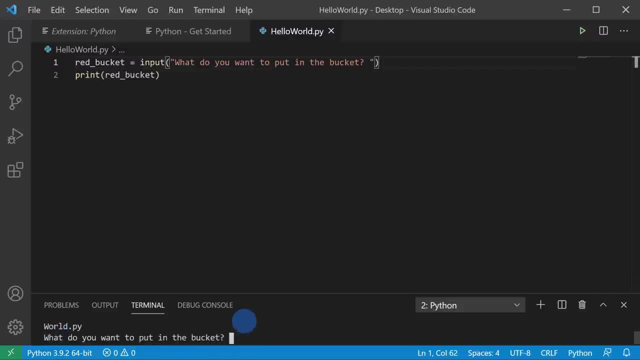 Right down here it says: what do you want to put in the bucket? And so maybe I want to put a shovel in. So I'll click down in the terminal type in shovel and then hit enter. And here now it prints out shovel, because that's now the value of the red bucket variable. 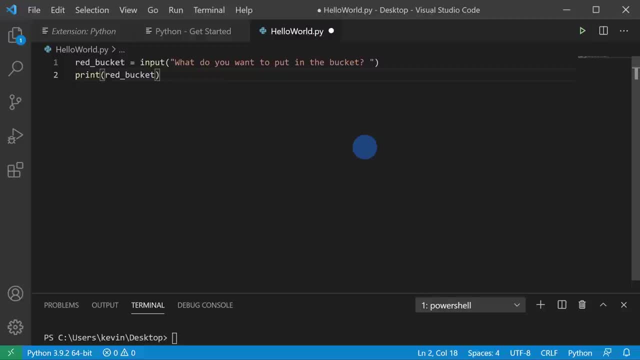 Next, I want to show you how we can start using conditional logic in our code. Basically, any expression that you enter in breaks down to either true or false, So let's just take an example. I'll go down a few lines and let me enter in print And I'm 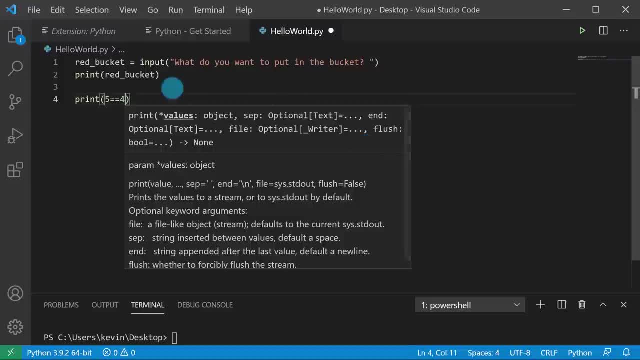 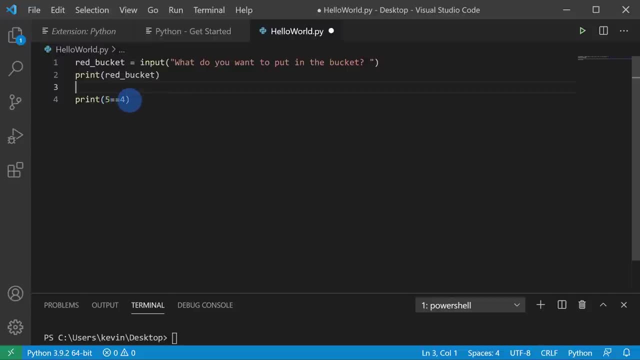 going to ask: is five equal to four? One of the things you'll notice is, when I ask this question: is five equals to four? I entered in two equal signs and that's not a typo Up above. I just entered in one equal sign, So why do I enter one here and down here I enter two. Well, 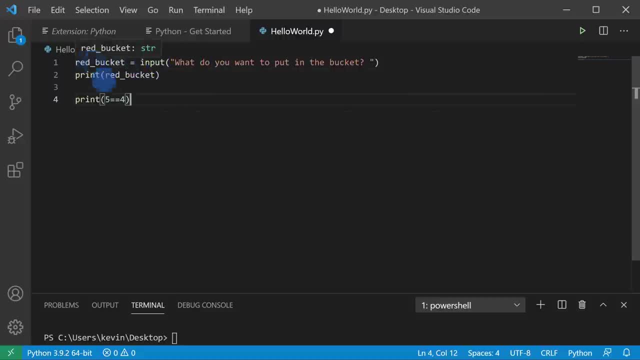 I'm going to run a test for equality. I basically want to check: are these two equal? And when you test or check for equality you use two equal signs. So here let me remove the code up on top and I'm simply going to print out: is five equal to four Here? when I run it here, we'll see that. 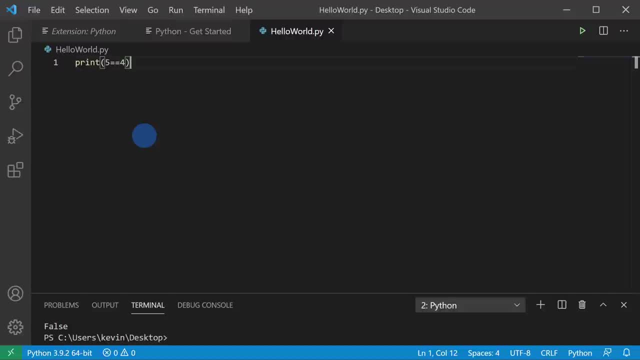 no, it's false. Five does not equal four. Now you might be saying: well, of course, five isn't equal to four, It's not equal to. So over here I can also check, are they not equal to one another? So here, instead of the equal sign, I'll insert: 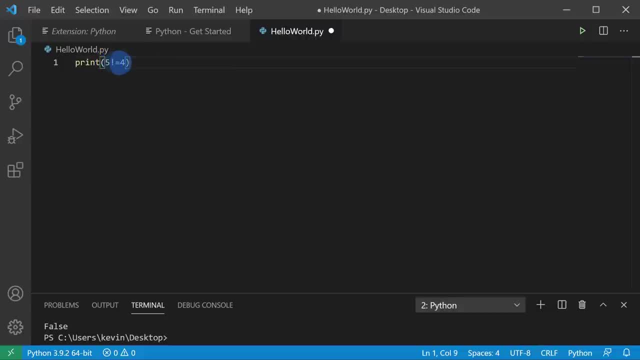 an exclamation mark. So here I have an exclamation mark followed by an equal sign. So this is my way of asking the computer: is five not equal to four? And I think we all know that's true. So when I run it here I get true back Along with equal to and not equal to. there are many other operators that 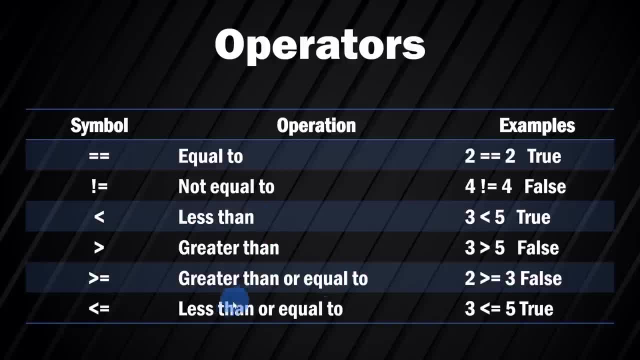 I can also use. I have less than, greater than, greater than or equal to, and less than or equal to, And here you can see the symbol that you can use for these different types of numbers. So I'm going to go ahead and type in the number of these different operations And over on the right hand, 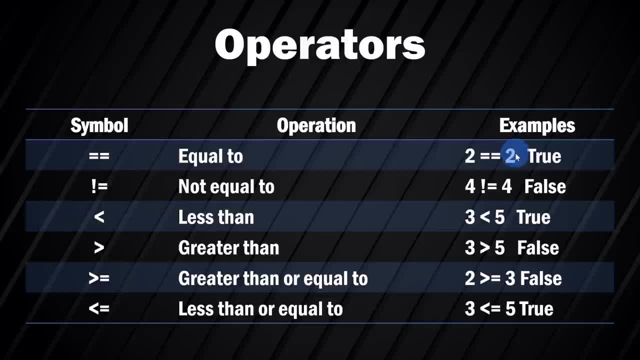 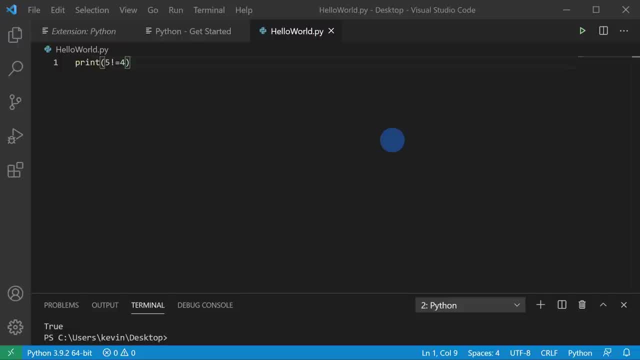 side, you'll see a few examples of how you could use this, So I could insert any one of these into that print statement and you'll get this corresponding result. We can now take these different operations, and we can combine it with variables that we just learned about, And so let's. 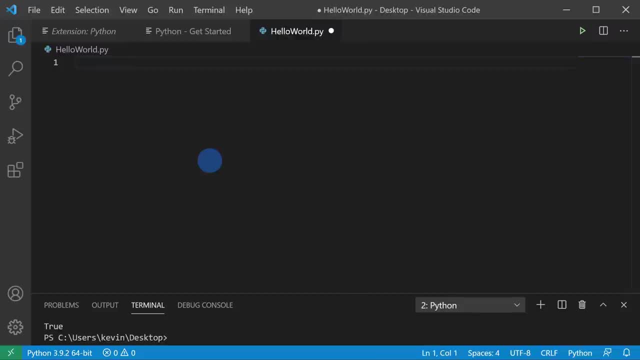 type in an example here. So I have a young son at home. His name is Thomas and he's just three years old. So let me create a variable and I'll call it Thomas age, and it's currently equal to three. So I'm taking this value of three and I'm assigning it to this variable. Now let's say I want to check. 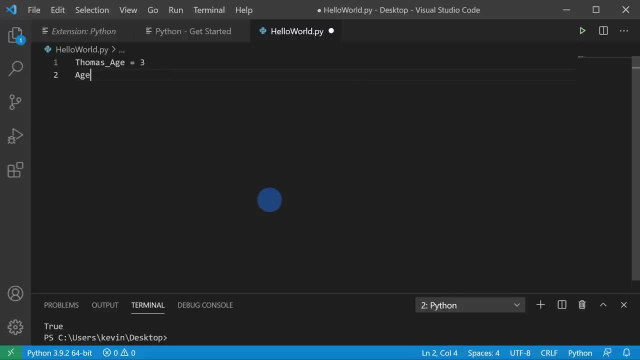 well, is he old enough for kindergarten? So maybe I type in age at and I'll type in kindergarten, and maybe age at kindergarten is five, So I'll enter in equals five. So I now have two different variables and I've assigned a value to each of those variables. Now down here: 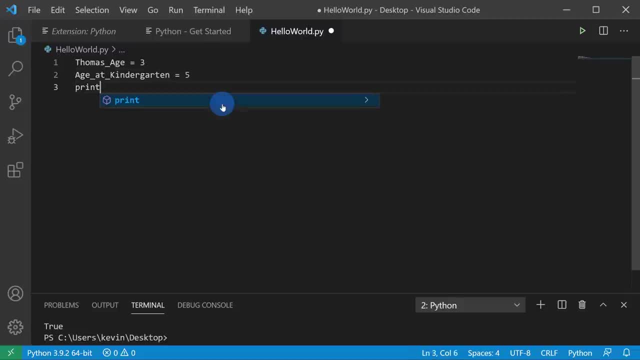 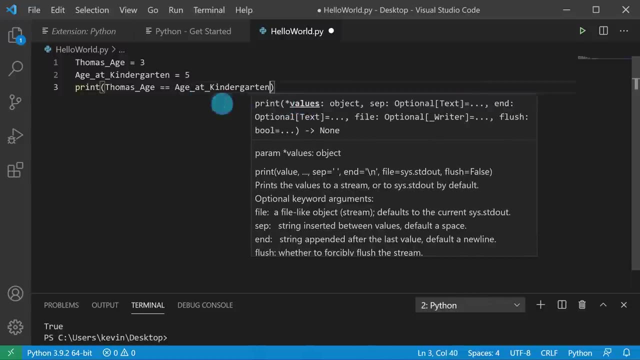 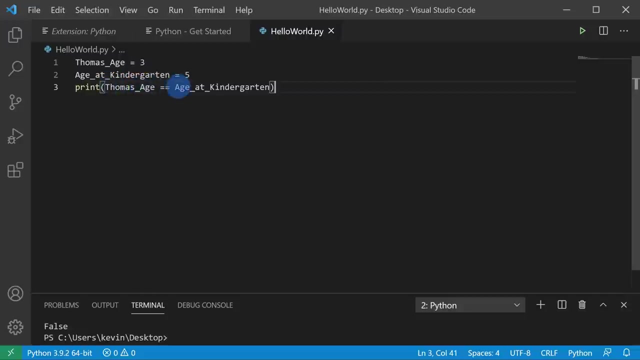 I can check the equality of these. So maybe I'll say print and let's check: is Thomas age, is that equivalent to the age at kindergarten? And so then I'll hit run and here we'll see that's false because basically Thomas age is coming back as three. age at kindergarten is five. 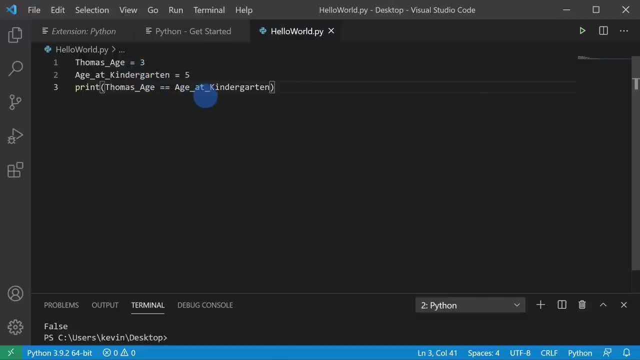 and those don't equal one another. So we can do this same type of check, except we could do it using variables. Now, with this expression here, I'm simply checking: is Thomas's age equal to the age at kindergarten? And it comes back as false. but what if I want to do something a little bit more? 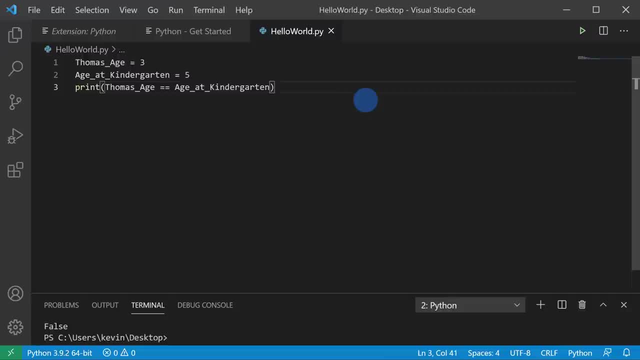 complex. I want to check. well, if Thomas is less than the age of kindergarten, well, he should probably be in preschool or daycare, And if he is five he should be in kindergarten. But if he's older than five he should be in some other class. And right now this is just doing one check, It's just looking. 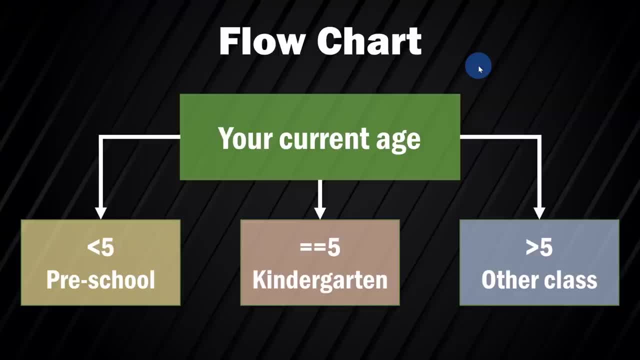 at one point Is he at the age for kindergarten? The easiest way to think of this is like a flow chart. So here I have the current age and, depending on his age, any one of these different scenarios could be true. Now, I won't be able to do that with the simple expression that we wrote, That's. 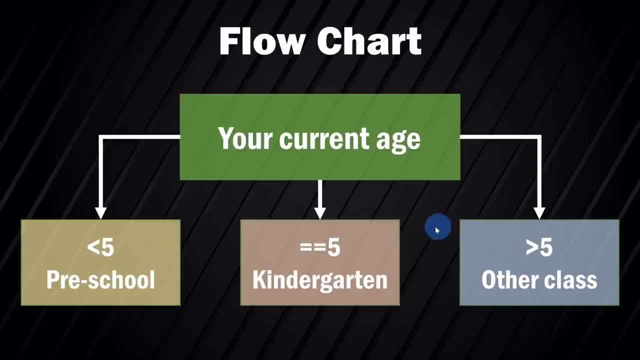 just checking one thing. If I want to check multiple different criteria, this is when I can use an if statement. So let's jump back into Visual Studio Code and let's look at how we can use this Back in Visual Studio. I'm going to delete this last line and I'll keep these two variables. 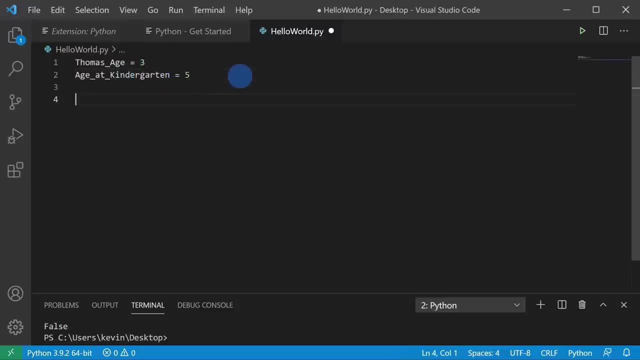 the one with Thomas's age and the other one with the age at kindergarten, And I'll enter down a few lines. Once again, the white space doesn't matter, so don't worry, You could enter down a few lines. And now we want to enter in an if statement. 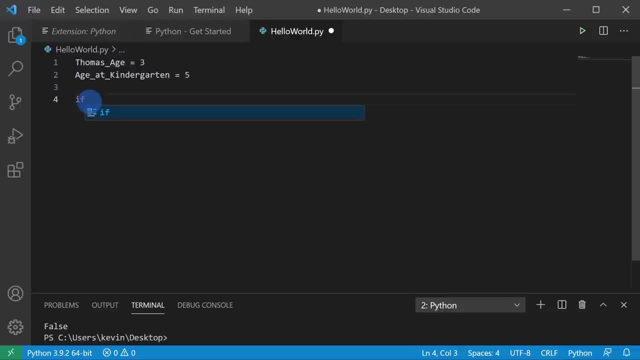 An if statement is really easy to write. You simply type in if, And here now I can do my check. So first I want to know: is Thomas's age less than the age at kindergarten? So here I could type in my variable Once again. it gives me this helpful suggestion of using Thomas's age. 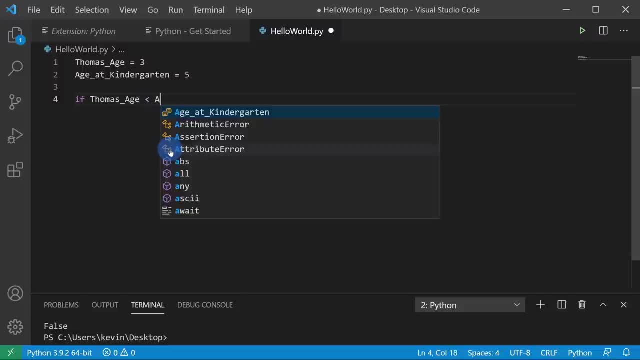 And first I can check if he's younger than the age at kindergarten. So let me enter in the age at kindergarten. So this is going to be my first check. Once I finish entering in this statement, and when I hit enter, this drops me down to the next line. One thing you'll notice is it: 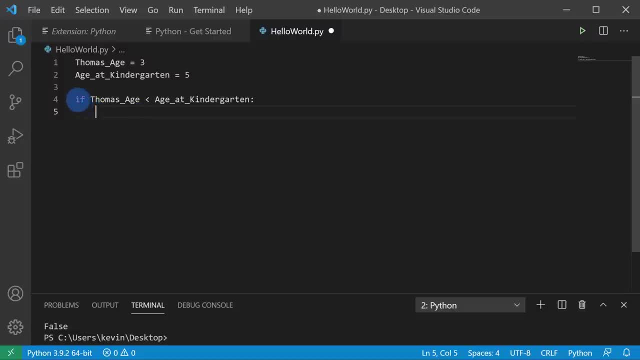 automatically indented the line- What'll happen is it'll check this And if it turns out that Thomas's age is less than the age at kindergarten- in this case, Thomas is 3,, the age at kindergarten is 5, so this would be true- it's going to evaluate this code. So whatever code I enter in here, 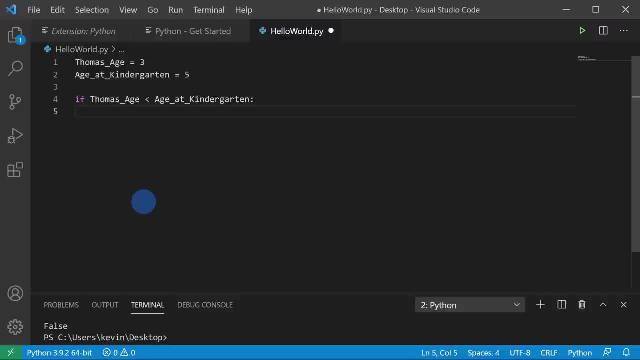 it'll go through and it'll execute that. So let's test this out and let me type in print, And maybe we say something like: Thomas should be in preschool. Once I finish typing that in, I'll go to the end of this line and hit enter again. Here you see that it continues to indent. 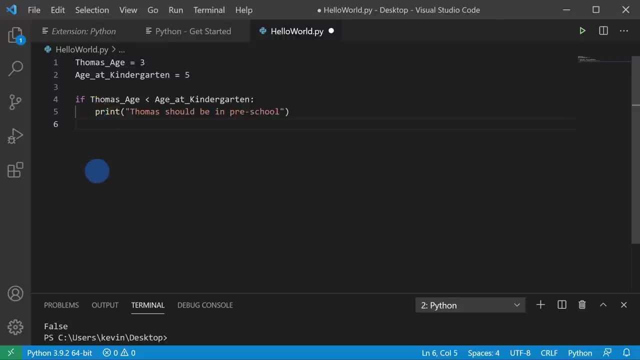 it. So, basically, I can type in additional code and whatever I type in in this indented space, it'll go through and it'll execute all of this code. Now I don't have anything else I want to run. I simply want to print out this message. Let's now test this out to see how it works. I'll go up. 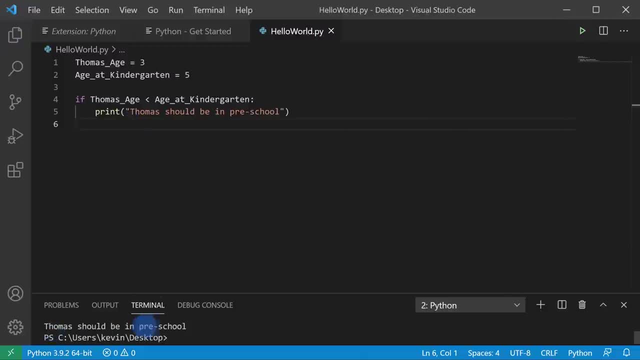 here and click OK, And then I'm going to type in print, And I'm going to type in print, And then I'll click on run And here we get the text that says Thomas should be in preschool. Now let's say that. 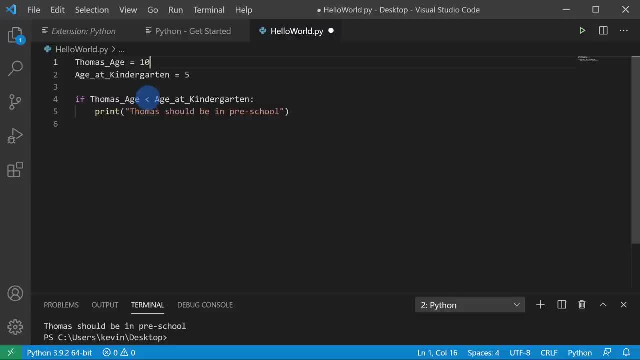 maybe Thomas is 10 now. So here Thomas is age 10 and that is not less than the age of kindergarten. So when I run here, I get nothing back, because it evaluates this and it comes back as false, so it doesn't execute this code. Now there's nothing else here, so it simply returns nothing. 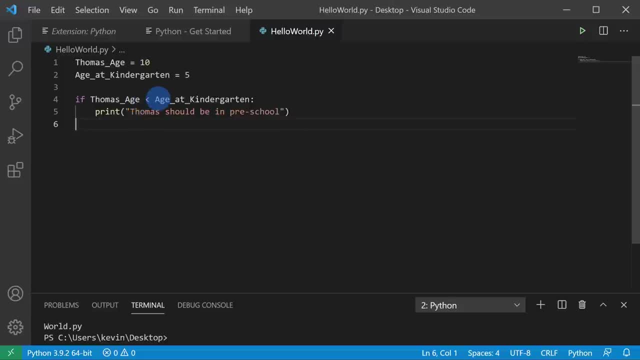 Now let's say I want some fallback. So let's say: if this is false, I want to say something else Down here I can use else. So it'll check this and it'll check if this is true. but if it turns out being false, 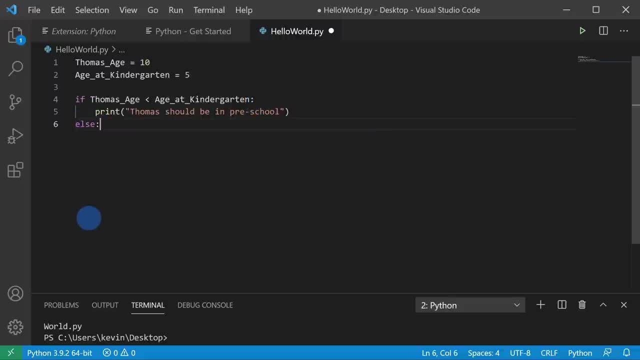 then it'll fall back to else. So here I'll enter an else, a colon, and here again it indents out. So here I could say: well, if this isn't true, then execute this block of code. So here, maybe. 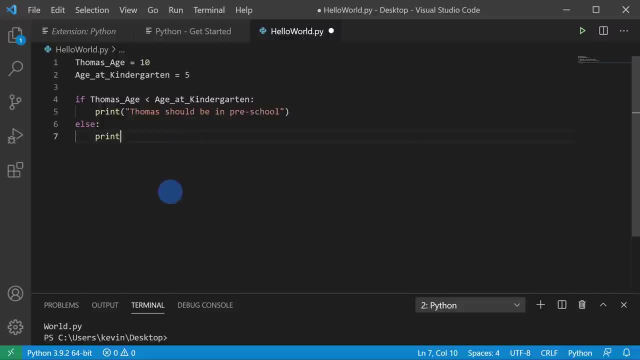 I'll insert another print function. So let me type in print. I'll open up the parentheses and let me type in: Thomas should be in kindergarten or another class. So I've now typed in my else statement, So let's try running it to see what it'll happen. So it'll check the first if. 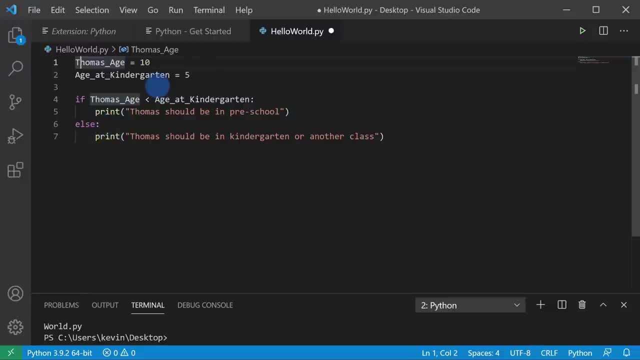 statement That'll evaluate to false and then it should fall back to else. Let's test this out. So when I hit run here, it says Thomas should be in kindergarten or another class. So this logic is working exactly as we expect it to. 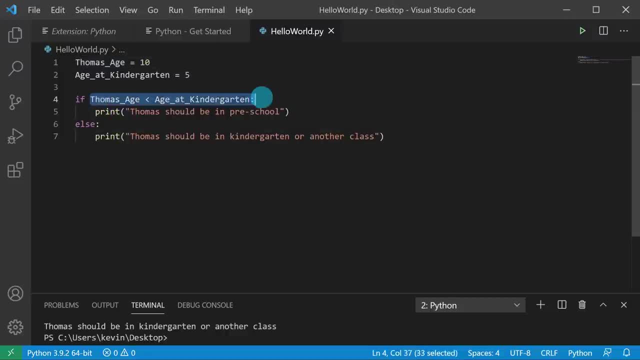 Right now I have two conditions here. I basically check the first condition and if this is false it just falls back to this one. But let's say I want to check for additional conditions Here. I'll enter down and let me get out of this block of code. So I'll hit the backspace key and right. 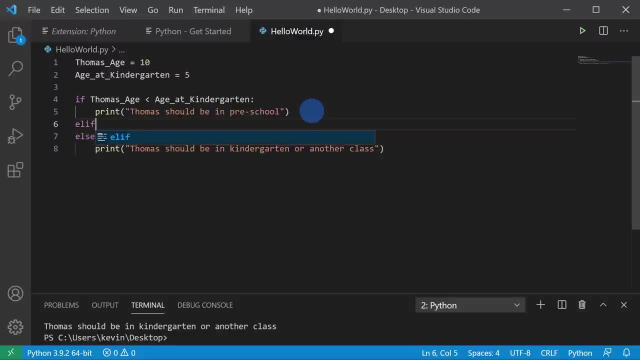 here I can enter something called elif, basically else. if So, you can go through and check any number of conditions. It'll start at the top and when it finds one that's true, it'll display that message and then exit. But if this is false, it'll go to the next one and check that condition. 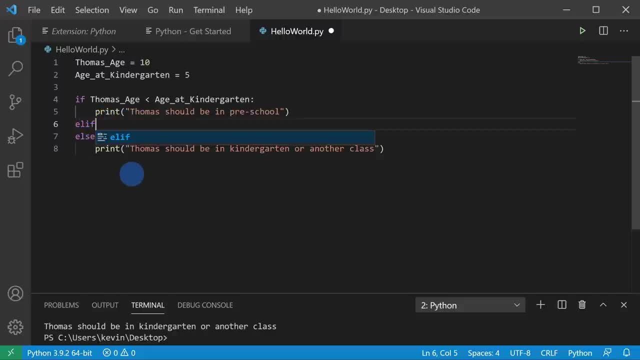 and I can add any number of else ifs in here. So I'll type in elif and maybe for this condition I want to know if Thomas is five. well, he should be in kindergarten. So here I'll say Thomas age and here once again I want to check if it's equal to the. 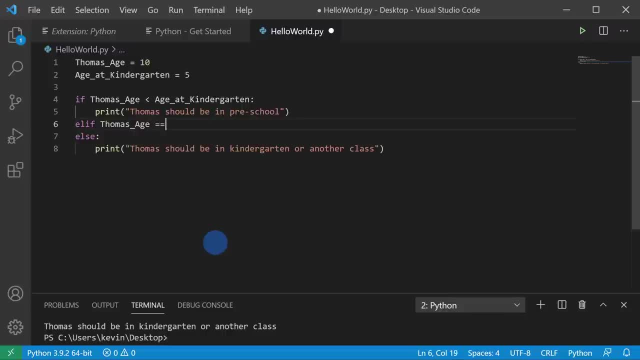 age at kindergarten. And remember, we don't enter in one equal sign, we enter in two, And here I'll enter in the other variable: age at kindergarten. So this is going to be my check And if this is true, we now want to evaluate some code Now, just like we did before, where? 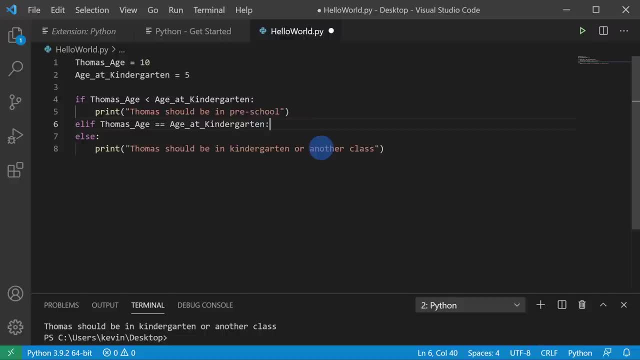 I entered the colon. let's make sure we enter in a colon here at the end. That's part of Python syntax. I'll hit enter and this automatically indents me Here. I'll type in print. I'll type in some text that says: enjoy kindergarten. Now I've added this. else, if 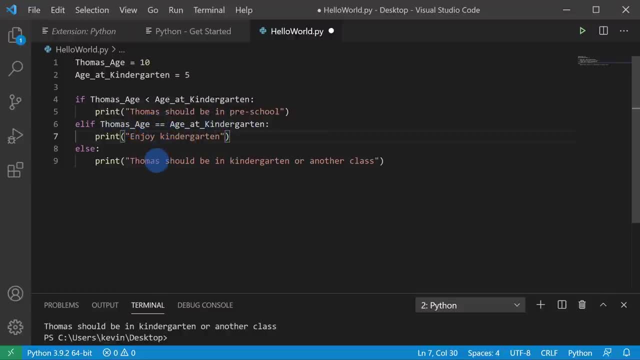 statement that checks to see if he's in kindergarten. So this last statement no longer makes sense, where I say Thomas should be in kindergarten or another class. So maybe I simply remove this and I say Thomas should be in another class. So this will just. 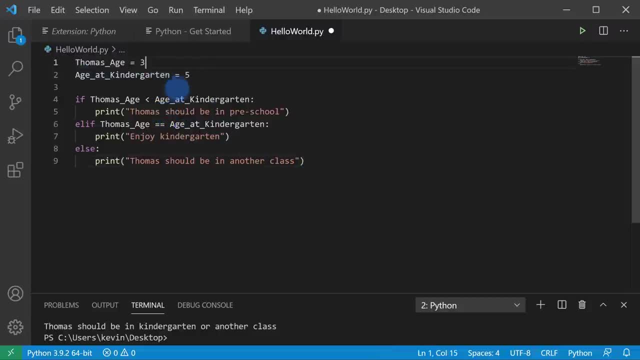 be my catch all at the end. So let's test this out to see how it works. So let's say Thomas is three and I run it. In this case the first condition here is true. So Thomas should be in preschool. And here I get the text down below: Thomas should be in preschool. Now let's say 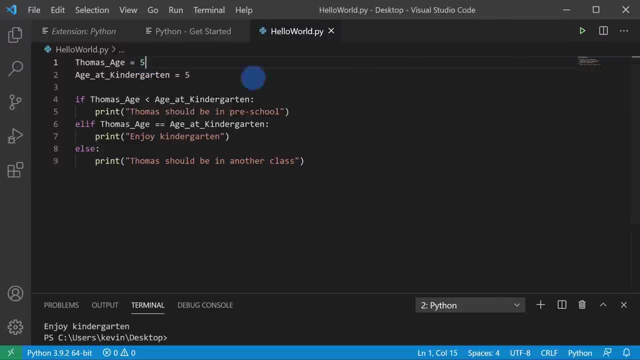 Thomas is equal to five, or maybe he's five years old now And we run it Here. the first condition is false, So it skips over that one. It looks at the second condition, this l if, And here Thomas is five, and that's the age at kindergarten. So here I get the text saying: enjoy kindergarten. 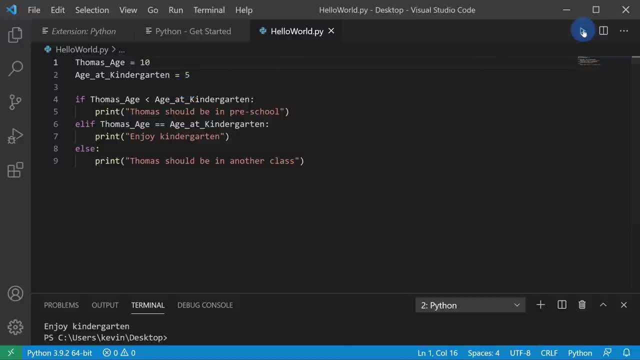 And let's say now that maybe Thomas is 10.. So here, when I run it, it evaluates the first statement. And well, he's older than the age of kindergarten, so that's false. His age is not equal to the age of kindergarten, So that's also false. And then it falls back to the l statement. And so Thomas. 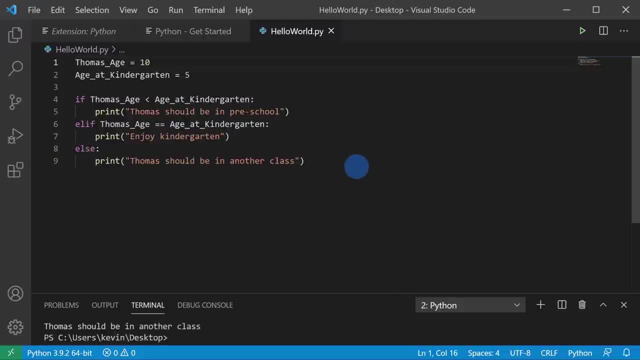 should be in another class. So here we've just tested that this is working just like we expect it to. Next, I want to show you how we can use functions in Python, And if you've ever used any other programming language before, you might know them as a subroutine or method, but it's all the. 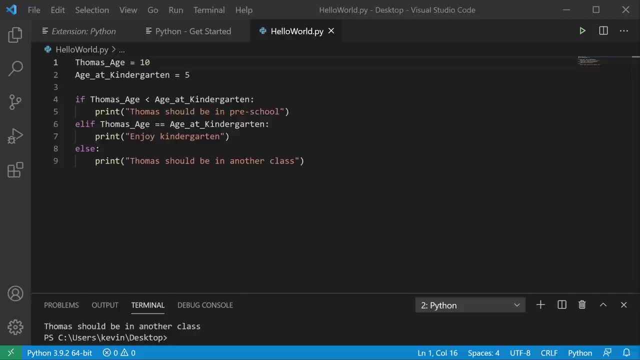 same thing. So we're going to use functions And you've actually already been using a function. We used the print function Right here. we've been using print multiple times. This is a function. You call this function, you pass in. 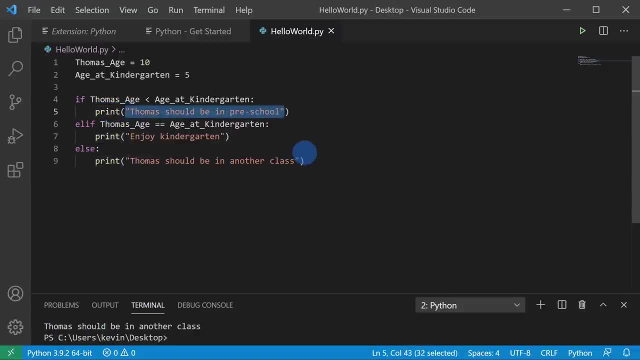 some text and then it prints it out on the screen. So that's just a basic example of a function that we've already been using. Now, the cool thing is, we can create our own function. So what is a function? Well, it's basically a block of code that you can package together with. 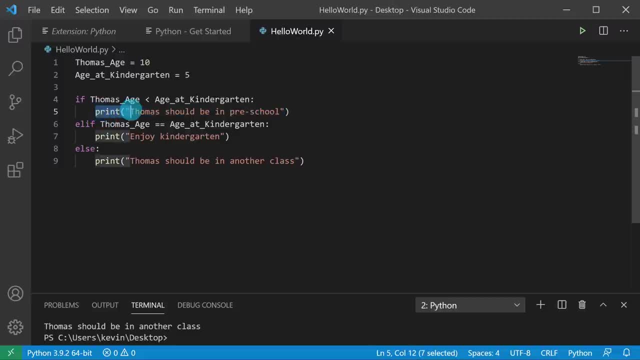 a name and it does something. So in this case, anytime you call print or input, it takes some action depending on the type of function that you're using. So in this case, anytime you call print or input, it takes some action depending on what that function is. 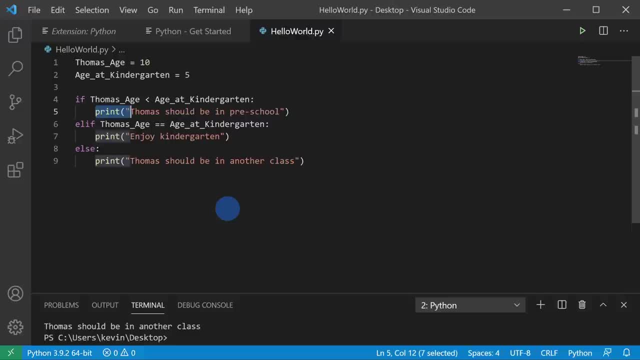 The neat thing is it makes your code more modular and also reusable. So here, for example, every time we want to print something on the screen, we simply call this function and then it takes that action. We don't have to enter in all the different code associated. 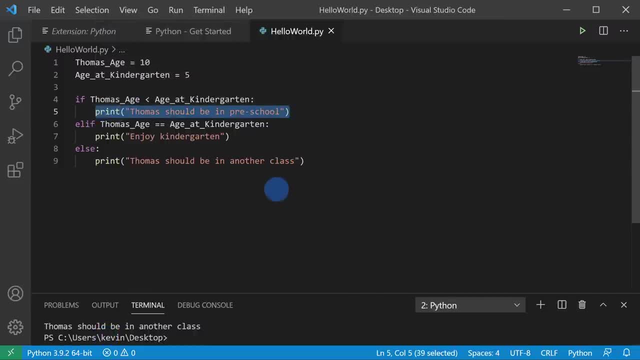 with printing your text on the screen. We simply rely on this function, So it makes your code a lot more reusable. So let's go through and create our own function. Right now, I'll go through and delete all of this code that we had And let's say: 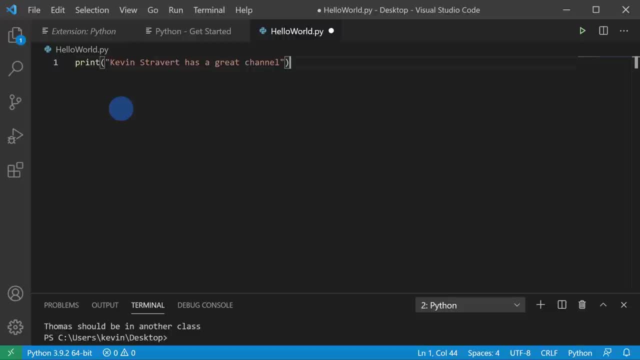 just to show the value of functions, let me just enter in print. and then Kevin Stratford has a great channel. I'm going to enter this in three times, I figure. the more I say it maybe the more it sticks, And the more you read it you might start to believe it. 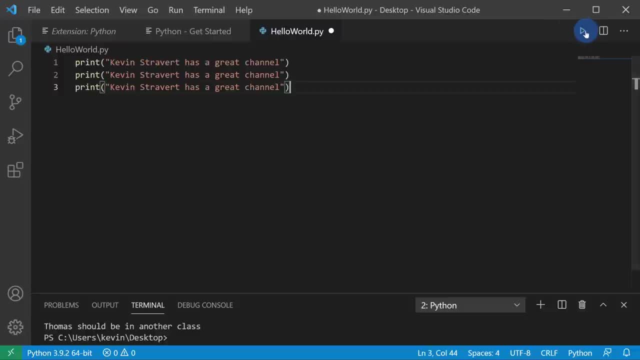 So here I've typed it in three different times and now I'm going to run it Here. I'll expand the terminal just so we could see it, and here print it out three times. Oh, but actually, look at that, It looks like I spelled Stratford wrong. Stratford has a T in the 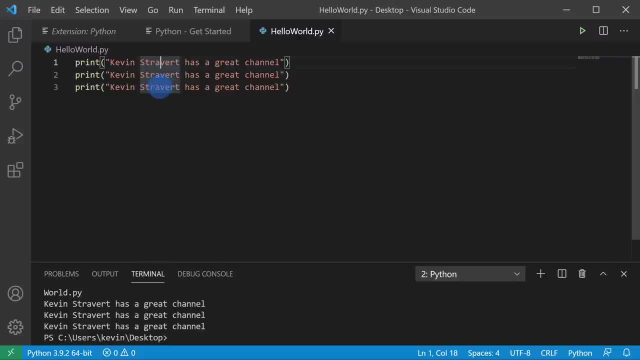 middle. and here I just say Stratford Now, because I'm not using a function for this while I'm using the print function. but I haven't created a function to print this out three times, So I'd have to go through and I'd have to correct every single Stratford throughout my code. 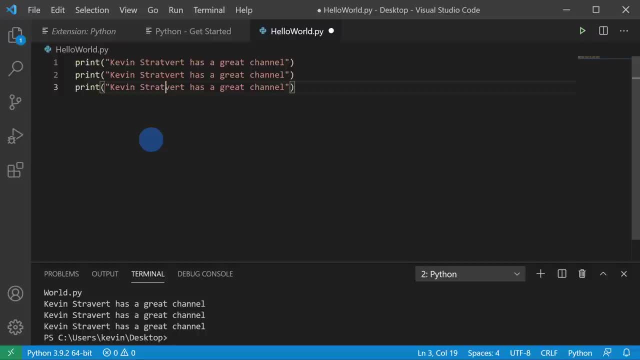 to correct this. And imagine that you reference something many, many, many times in your code and maybe you make an error. you need to update something. It could be a pain to have to go through all of your code to update it, So instead you can create a function and I'll show you how we. 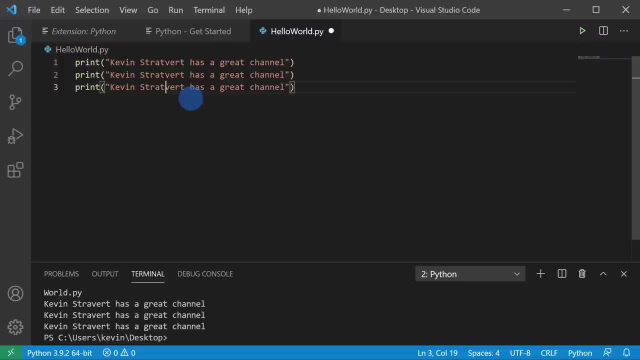 can create a function, to print this out multiple times and then we can call it whenever we want. Okay, So let's create a function. I'll simply go down a few lines. To create a function, we have to type in def. This is basically stands for define. So I'll type in def. and here we can. 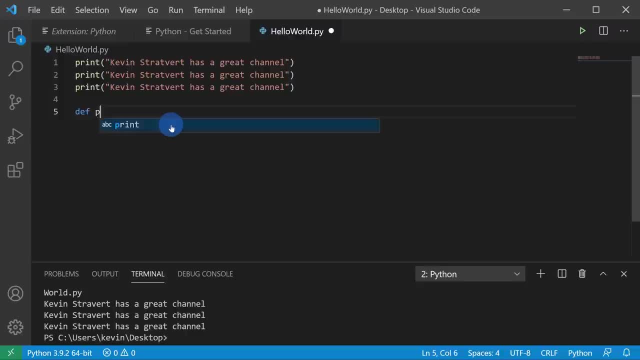 type in a name for our function And I'm going to call this function, let's say, print Kevin. So I've typed in my function name and then all functions need to have parentheses at the end. So I'll close the parentheses and right down here once again, just like we did with the if. 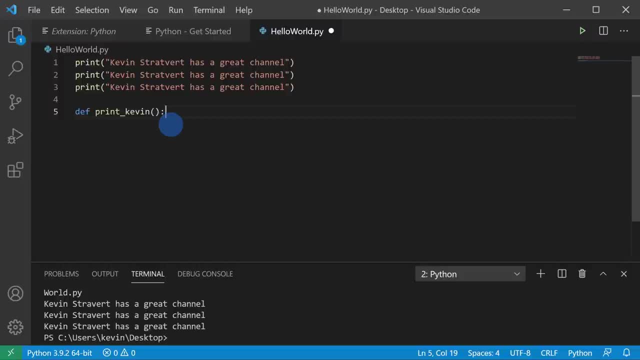 statement, I'll insert a colon. So I now have my function. When I hit the enter key, here too, just like with the if statement, you see that it indents it automatically. So once again, it indents, and any of the code underneath here will be part of this function. 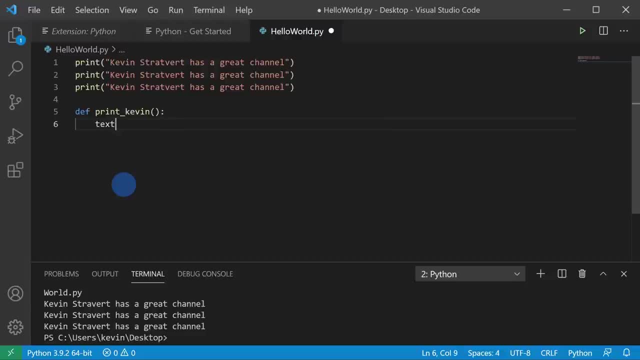 Next, I want to enter in some code in this function. So maybe I'll set up a variable and I'll call this text And let me insert some text here in quotes, and maybe I'll say: Kevin has a great channel, So that's going to be my text, And here maybe I'll just 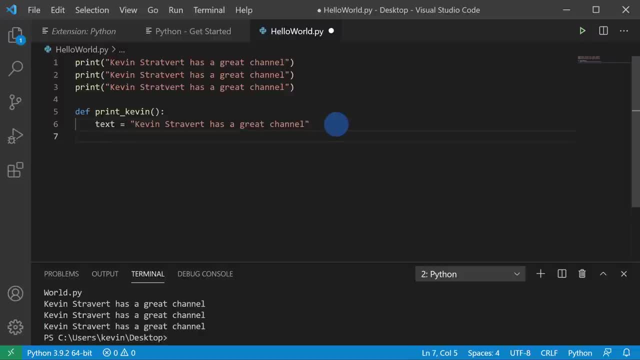 make the error again where I don't have the T Now, right beneath that here I could use print and maybe I say let's print the text And I want to print this three times, So I'll insert it in three times. right here, I'm going to delete this earlier example here. 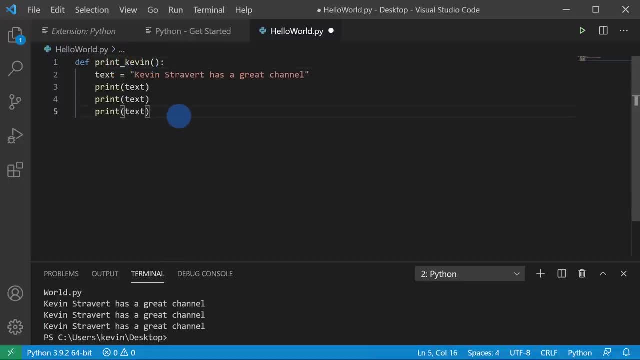 So we just have the function. So I have my function. now Can I run it? Let's try clicking on run. So I click on run and I get nothing back. And the reason why is right up here. we've defined a function, but we haven't actually called this function. 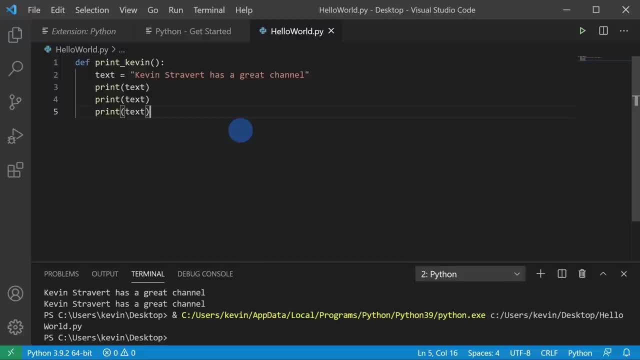 So I've defined what should happen when I call this, but we haven't called it yet. So here I'll go down and I'll backspace, So I'm out of this block of code that's associated with this function And here now I can call my function. So just like we called the print function, 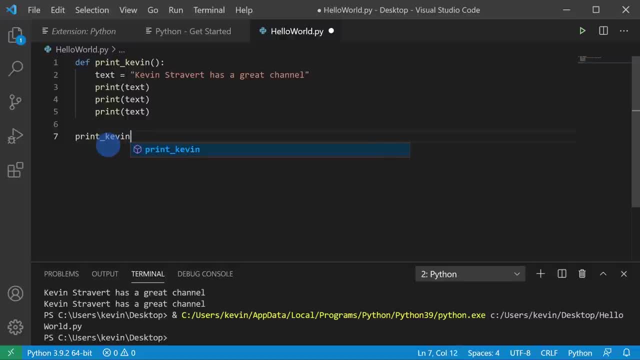 here I could say print and let's type in underscore Kevin, and then I'll open and close my parentheses. So right now this will call the function. So when Python sees print Kevin, it'll look up to this definition for Kevin and then it'll execute this. 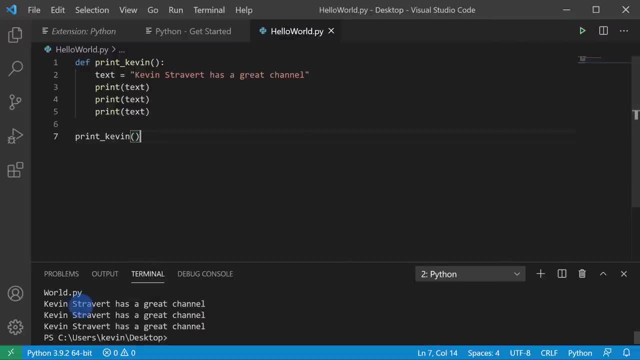 code. So let's click on run to see what happens. Now, look at that. Kevin Strafford has a great channel and it printed it out three times. Oh and look, there's that error in here. So right up here I could go to my function, I could add the T and then I can hit run. 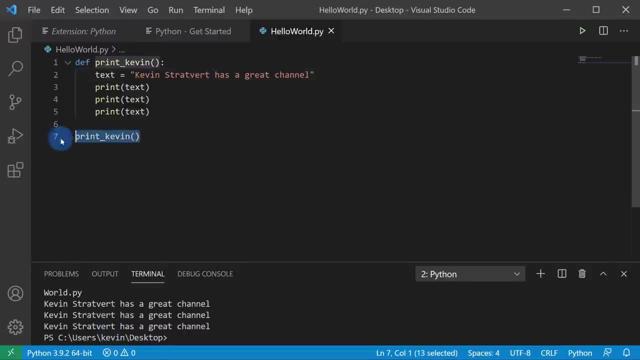 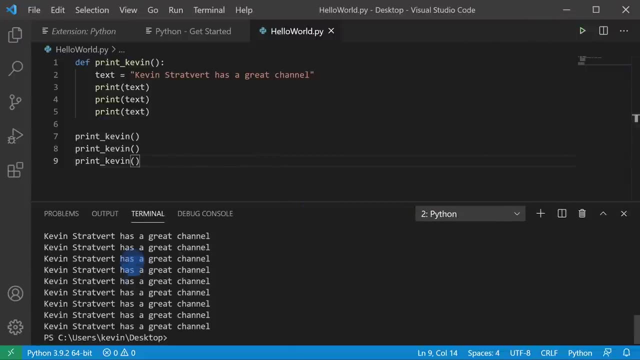 And it looks like that's now successfully updated in all cases. Now I could go through and I could call this function multiple times. This will really boost my ego. So now when I hit run, look how many times it's printed out: Kevin has a great channel. 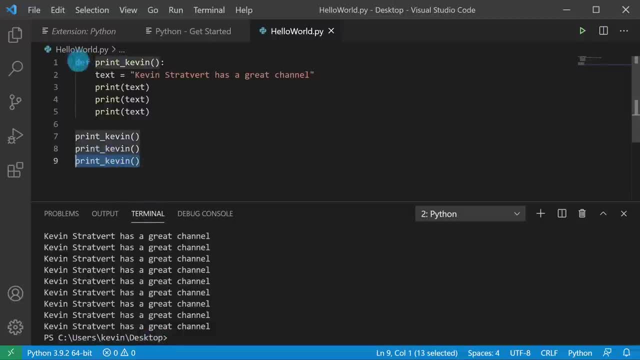 Every single time I reference this function, it'll go back up here, it'll look at the function definition and then it'll run this code within that function. With a function to be able to call the function, I first need to define it before I can call it. 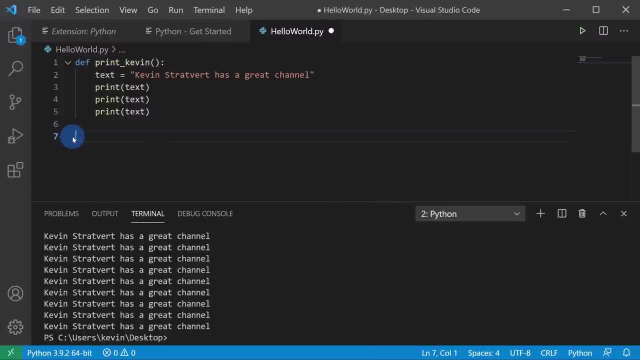 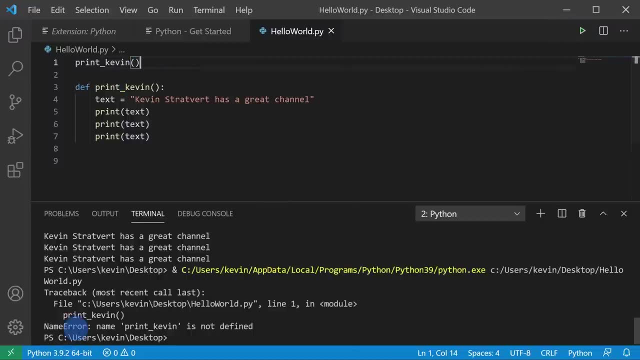 Here I'll remove these two references to the function. And so let's take the call of the function and I'll move it to the very top. So here I call the function and then I define it. So if I hit run now, here you can see that the function is now printed out. So now, when I hit, 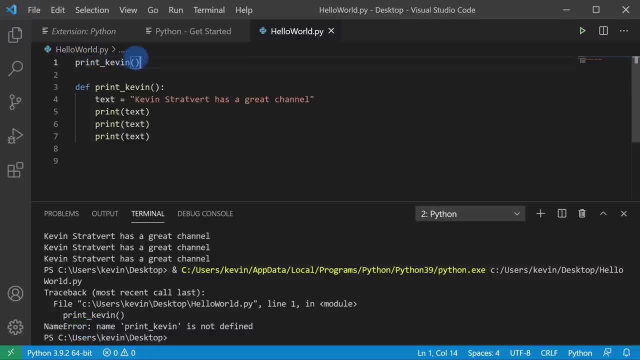 run. look how many times it's printed out. Kevin has a great channel. Every single time I reference here, you get an error because here it says: well, print Kevin. Well, it doesn't know about that function yet because it comes up later on in the code. So once again I need to make sure. 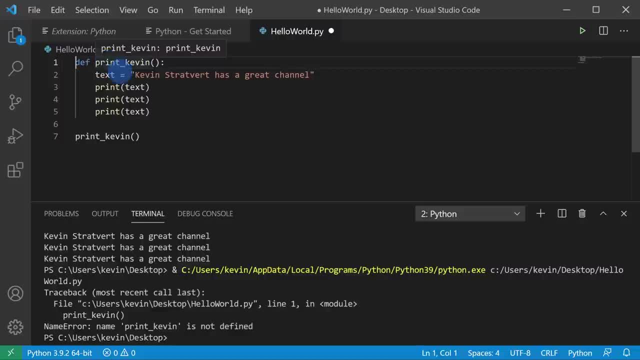 I call this function after I've defined my function So typically in code. you'll see all of the different definitions, or all of the different definitions of the functions, at the top. One of the neat things, too, about using Visual Studio Code is here. when I click over in the 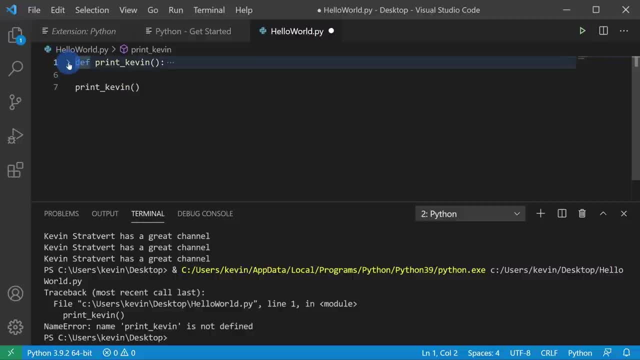 function and I hover over, I can collapse this function. So let's say I'm writing code and I want to have a whole bunch of functions, So I can collapse this function. So let's say I'm writing a whole bunch of functions that do different things. I can collapse it. and then 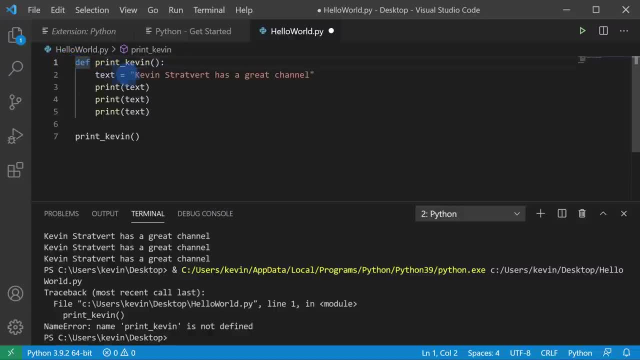 that way it clears up my view a little bit, and here I could expand it if I need to jump into this function and update any of the code within. With this one function that I defined on top, currently I don't pass anything into the function and I also don't get anything back from the 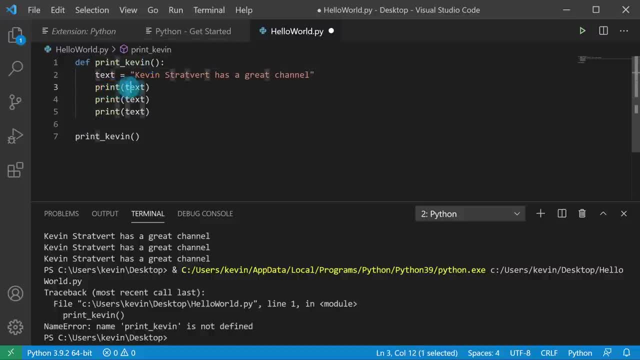 function. If you remember the print example here with print I'm passing in certain text that I want to print. So basically I'm sending in an argument or a parameter, and I could do the same when I create a function. So let's say, instead of entering the text here within the function, 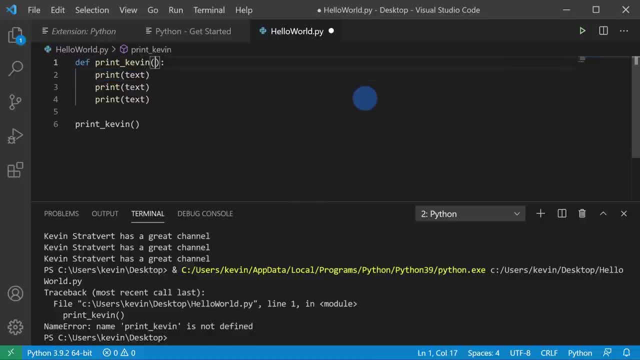 let me actually get rid of this line right here And right up here, as part of my function definition, I'll type in text. So, as I define my function, it's expecting me to pass in some value. So let's now go down here and look at the position where I'm calling my function. It says: print Kevin. 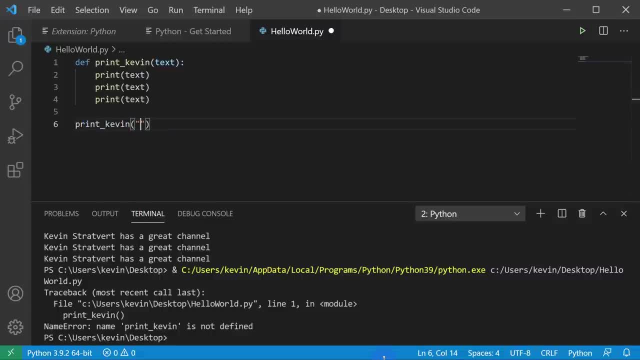 and here I can now pass in a value or basically pass in a parameter. So I'll type in. Kevin Stratford has a great channel. So here you'll see as I call this function. it's passing in this parameter or this argument. When I pass this in here, in the definition it says it's expecting. 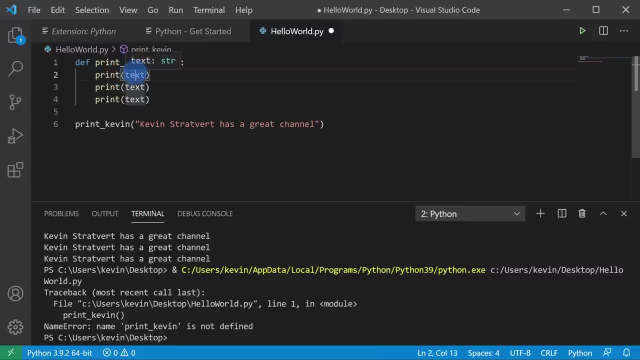 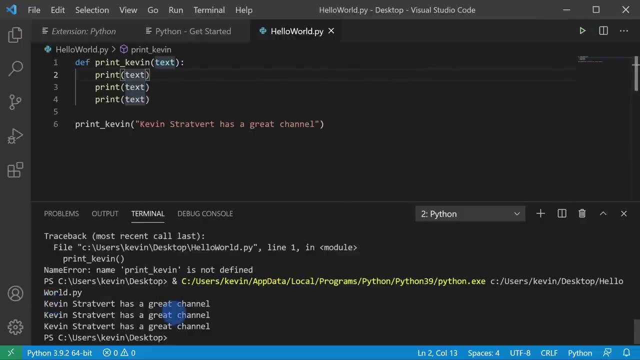 some text to be passed in, And down below the print is taking that text that I pass into this function. So now, when I hit run here you'll see the same result. Kevin Stratford has a great channel, And this is just an example of how you can pass values into your function. Next, I want 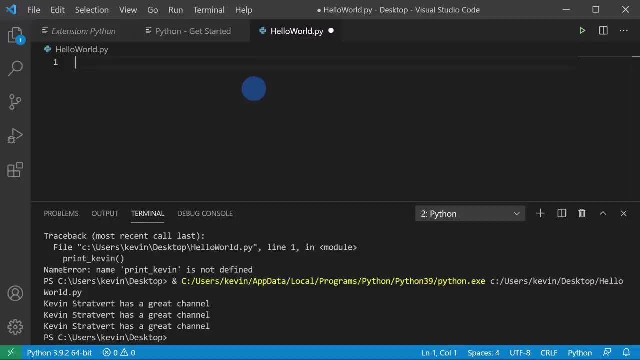 to show you how we can put an if statement within a function. So here again I'll type in D, E, F. This will define my function And I'm going to call this school age calculator. So I want to basically determine, based on a child's age, where should they be in school. And I want to get two. 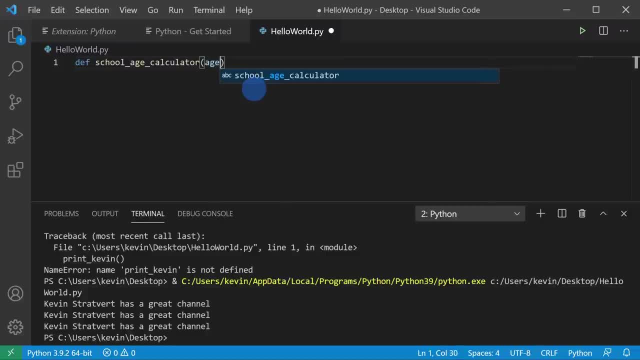 different values. I want to get the child's age, So I'll type in age as one of the parameters or arguments I want to get, And I also want the name of the child. Now, just like we did before, let's put in a colon here and then let's press enter. 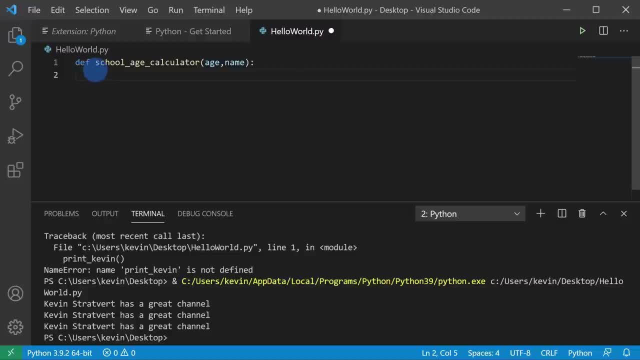 Here. once again, you'll see that it automatically indents me, And so that shows that whatever code I write here is part of this function. And now I want to insert my if statement. So I'm going to check first off. if the age is less than five, Once again I'll insert the colon, And when I press 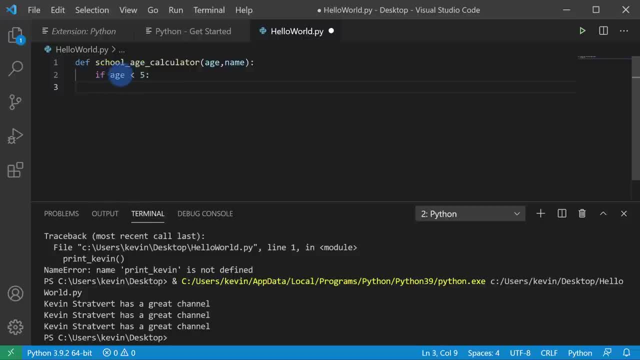 enter here, it indents me even more. So now I'm within this if statement. So if this evaluates to true, we're going to execute this code. If it's true, I want to display some text. So here I'll call the print function, Here I'll open it. 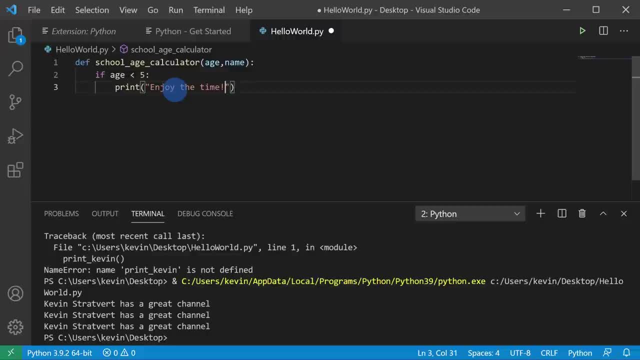 and maybe I show some text that says: enjoy the time, You're still a young guy, You don't need to be in school yet. So I've typed in some text Now. earlier we've just been printing out text, but I can also print out variables together with text, So here I could enter a comma and then I'll. 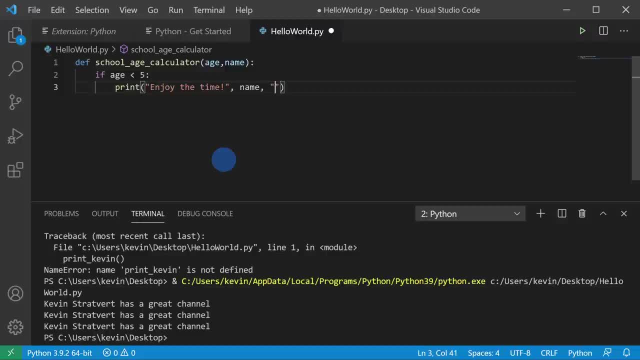 type in the name. Here I'll type in another comma and let me enter in quotes again And I'll say: is only Here I'll enter another comma and then I'll type in the variable age. So here you can see what it'll do. Let's say, the age is three and the name is. 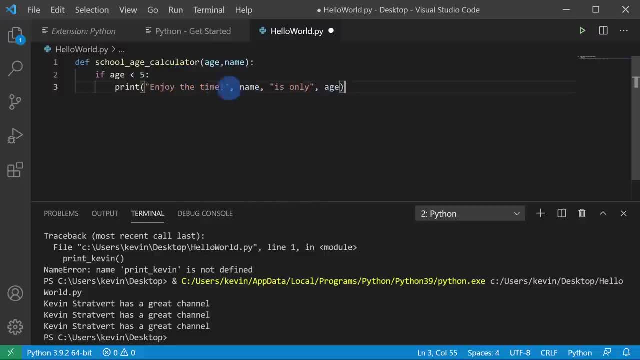 Thomas. It'll say: enjoy the time. Thomas is only three, So that's what we'll display. if he's under five, Let me hit enter. And here now I want to enter another condition, So I'll hit backspace, so I go back And here I'll enter elif. basically else, if, And I want to say if, age, let's say: 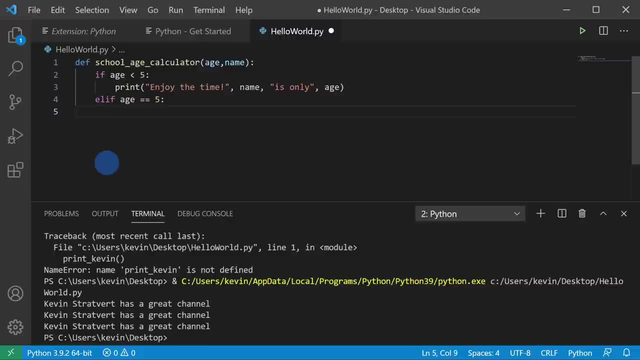 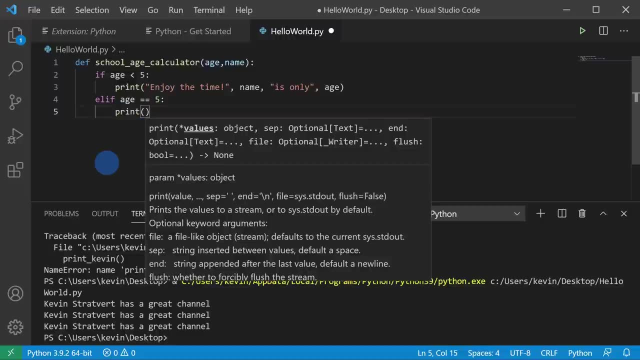 is equivalent to five, Then I'll enter the colon And here maybe I'll say enjoy kindergarten and then I'll show the name. So here I'll type in print and then I'll open the parentheses And I'll type in the quotes And here we'll say enjoy kindergarten And here I'll type in a comma. 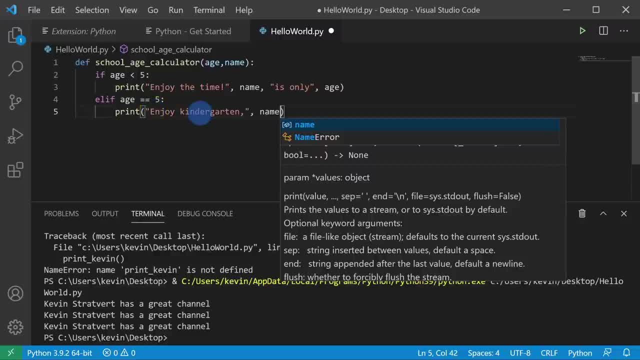 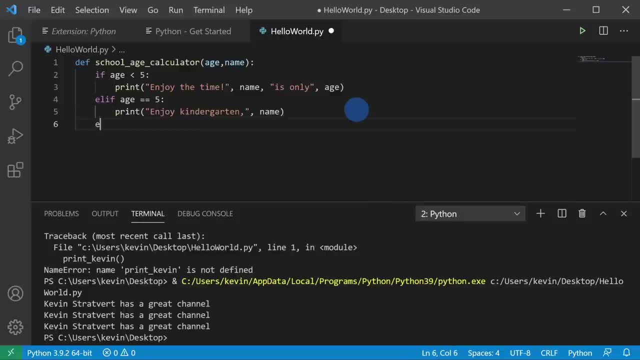 And let me type in another comma here And then I'll display the name. So here it'll say enjoy kindergarten, Thomas. And lastly, I want to add one more condition. So I'll hit enter backspace And here I can say else, colon, And here maybe I'll say print, And this one I'll just display. 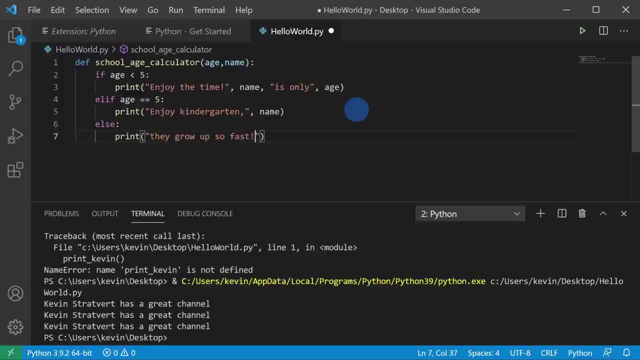 text And I'll say: they grow up so fast. exclamation mark. I've now finished defining all of the different conditions within the function, So here I could enter down and I'll press backspace twice so I exit out of both the conditions and also the function. 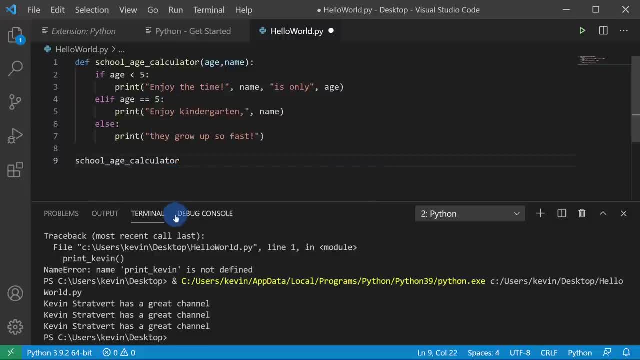 So now, here I can call my functions. I'll call school age calculator And here I need to pass in two different values. I'll pass in the age, I'll enter a comma And then I'll type in the name Thomas. So now, if I run this here, you'll see that it calls the function and then it goes through. 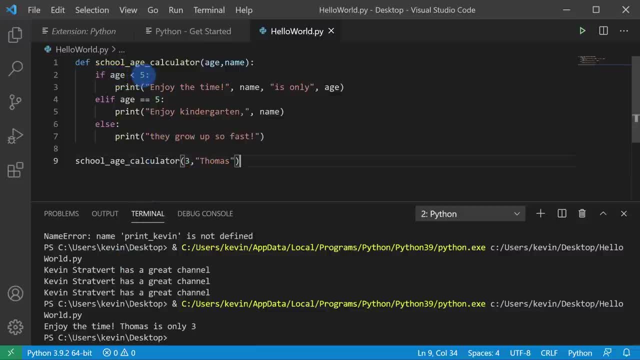 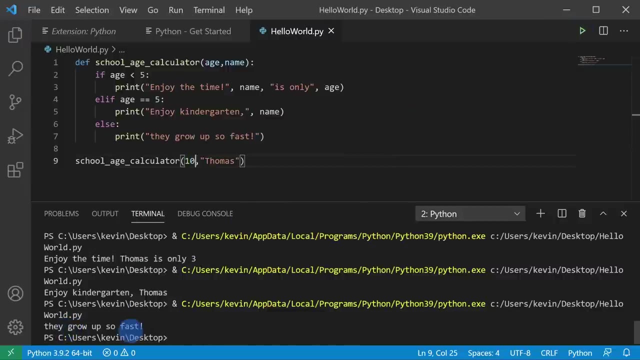 all of these different conditions. And so here, well, Thomas is the name Thomas. And then I'll say: enjoy kindergarten Thomas. And if I run it, here it says: enjoy kindergarten Thomas. And let's say Thomas is now 10. And I'll run it. And here it says: they grow up so fast. So here now you see. 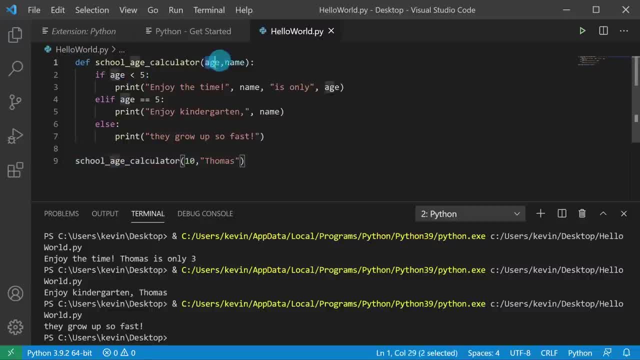 how we can call a function And here we pass in values into that function And it uses those values to run an if statement and to evaluate which one is true. Next, I want to show you how you can also run a function in a function. So let's go ahead and run a function in a function. 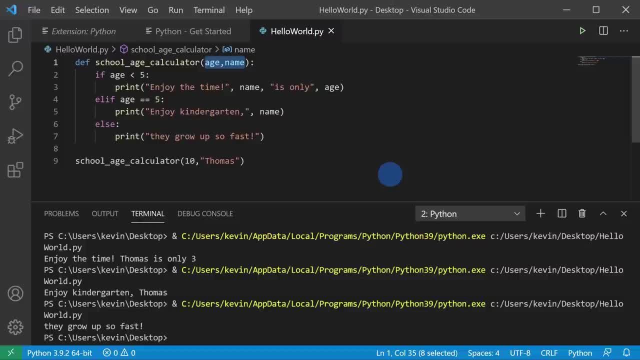 So let's go ahead and run a function in a function. So let's go ahead and run a function in a function, And now we're going to look at how you can get a value back from your function. So far we've looked at how you could just run a function on its own, how you could pass values into the function, And 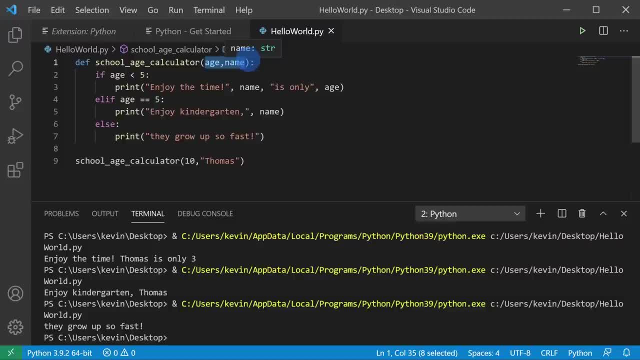 now we're going to look at how you can get a value back from the function I'm going to go through. let's remove this code right here and let's start again from scratch For this one. it's just going to be a really simple example. I want to know what is your age going to be in 10 years? And we'll use 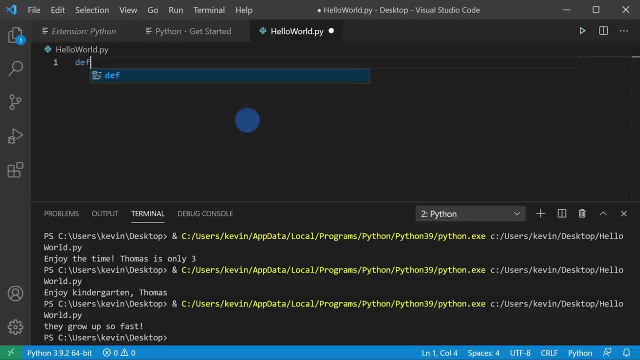 a function to do this. So here, once again, let's define a function by typing in DES, And here the function name will be add10 to age. Once I've typed in the function name here, I want to get one bit of input into my function or one parameter. Here I'll type in the age. 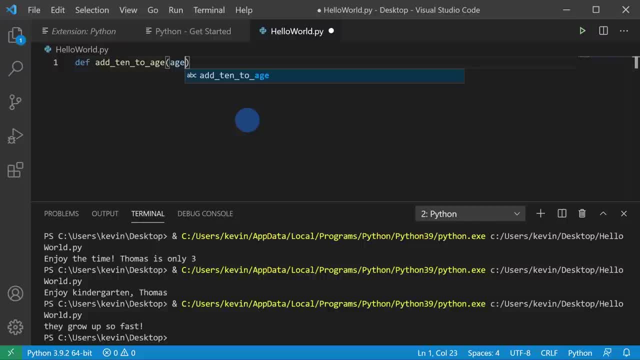 So someone will send in their age and then the function will add 10 to that age. At the end of the definition of the function, let's enter a colon and hit enter Here. this automatically indents me, And now, right now, I want to figure out what the new age is. 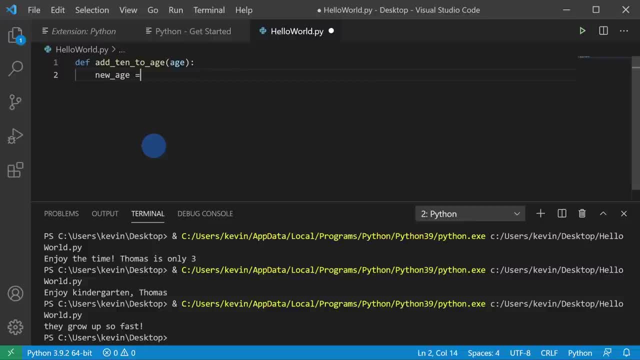 So here I'll create a variable called newAge And I want to set that equal to the default value, And here I'm going to write the value of age, And so what? I'm equal to the age that's being passed in. So I'll type in age and I'm going to add 10 to it, And 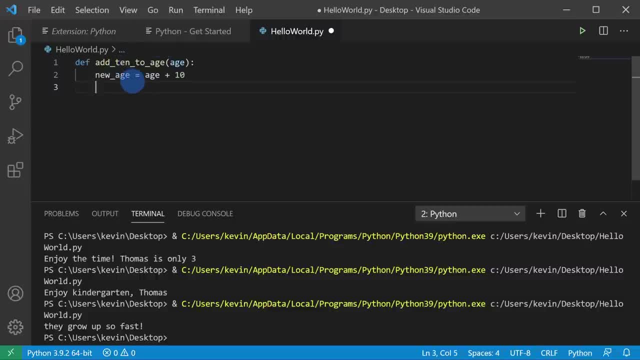 right underneath that. now, once the function runs through and it does its magic, I want to return that value. So here I'll type in return, and I want to return the new age, So I'll select this. This will send the value back or return the value once the function is done running Here now I want to 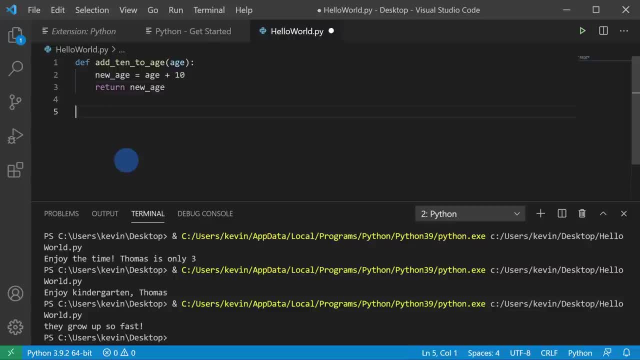 call my function. and when I call the function I can assign that return value to a variable. So here maybe I create a new variable called how old will I be, and I can set that equal to my function. So here I'll call the function add10 to age. and here I want to pass in, let's say, my son who's. 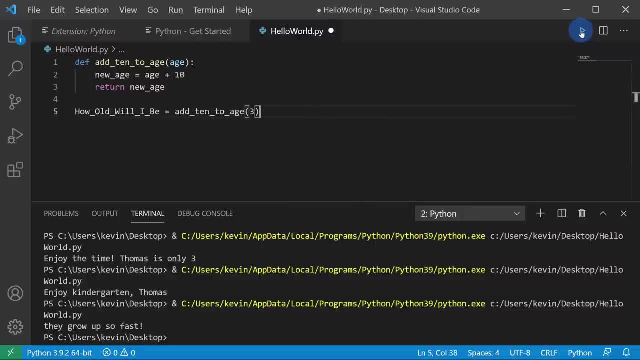 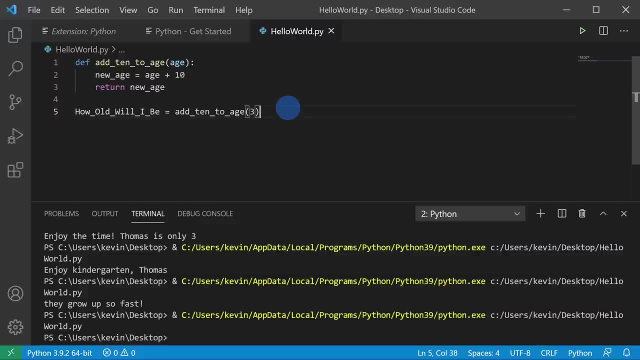 three, so I'll pass in three. So once again, if I run this right now, it won't actually do anything. It's assigning the output, which is 13, to how old I be, but now I need to print it out. So right down here let me type in print and I'm going to print in. 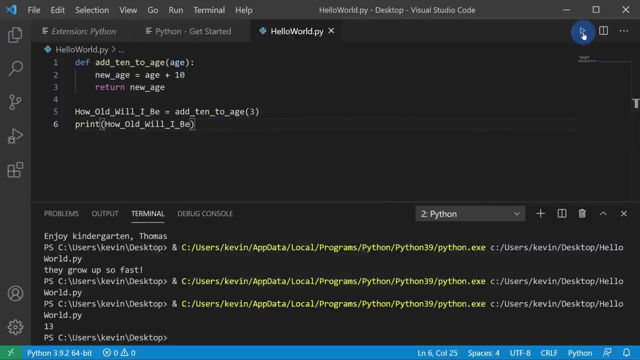 how old will I be? And now, if I hit run here, we'll see that that comes back as 13.. Now, once again, just to see how this works: here I'm saying how old will I be? This is a variable and I'm 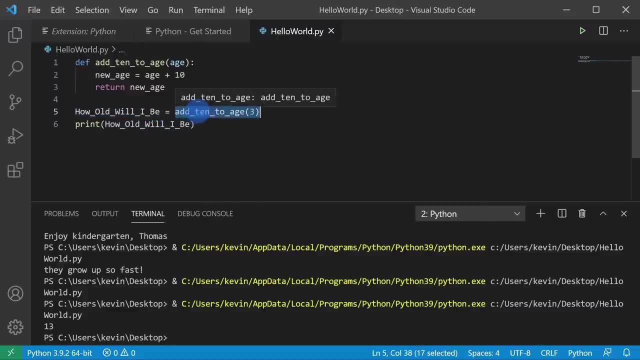 assigning this value to it, which is basically my function of add 10 to age, and I'm passing in 3.. So here it gets the age of 3.. It takes 3, adds 10,. it assigns it to new age. 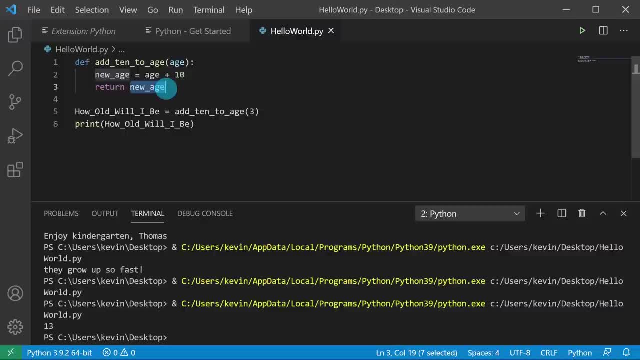 and once it's done, running through the function, it returns the new age. So the new age is 13 and it assigns 13 to how old will I be, And then here it prints out 13.. So that's how it works and that's how you can get or you could return a value from a function. 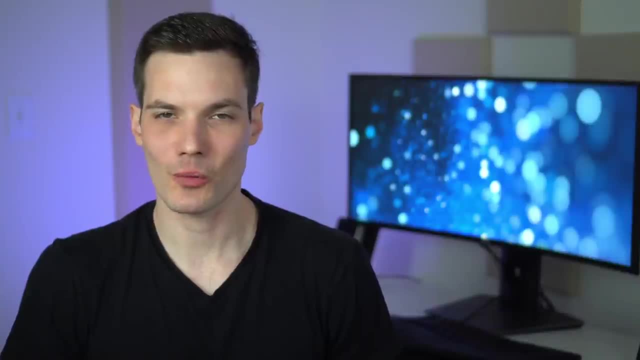 Next we're going to look at how you can use loops. What is a loop? Basically, it allows you to execute a block of code multiple times. So think of it this way: Every single week, my wife comes to me and says, Kevin, can you take out the trash? And she asks me that every single week. So, in a sense, 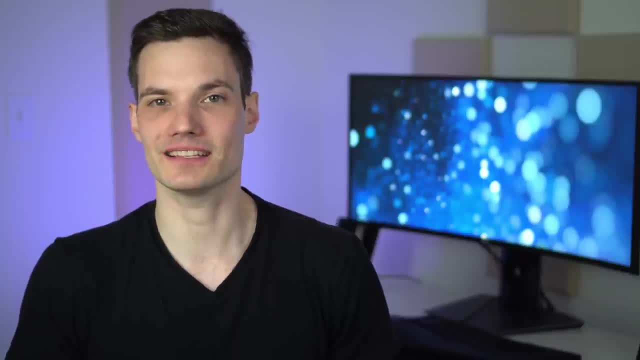 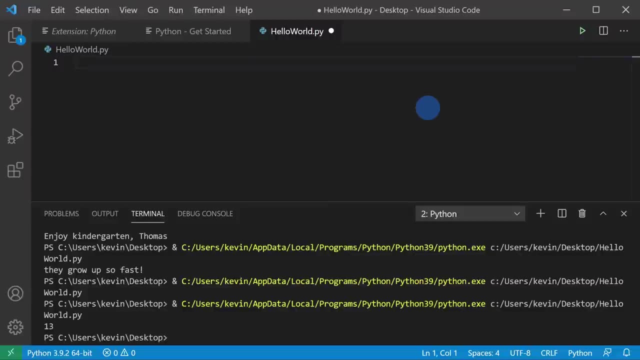 that's kind of like a loop. All right, let's jump on the PC and let's see how we can create a loop in Python. So let's now create a loop, and there are two different types of loops. One of them is called a while loop and the other one is called a for loop. We're going to start with. 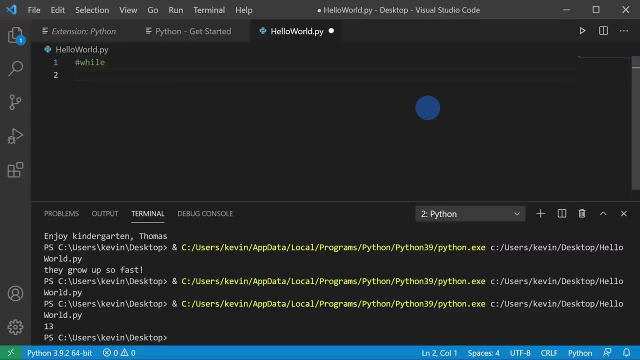 a while loop, And it's actually pretty easy to do. I'm going to create a variable just called x and I'll assign it the value of zero. And so here now I can type in a while loop. So I'll say, let's say while. 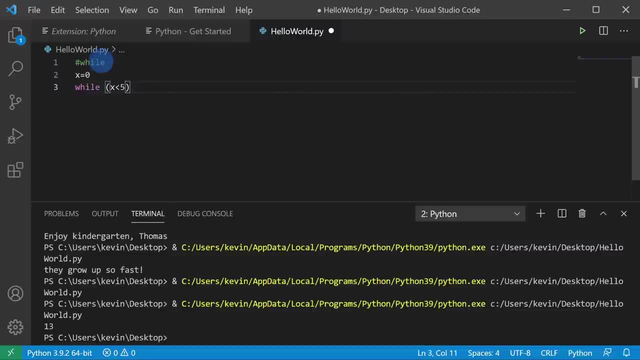 and let's say x is less than five. So while this value is less than five, I want it to execute some code. So here I'll insert a colon. We do this with our if statements, with our functions Here. when I hit enter now, it automatically indents me. So I'm now within the loop. 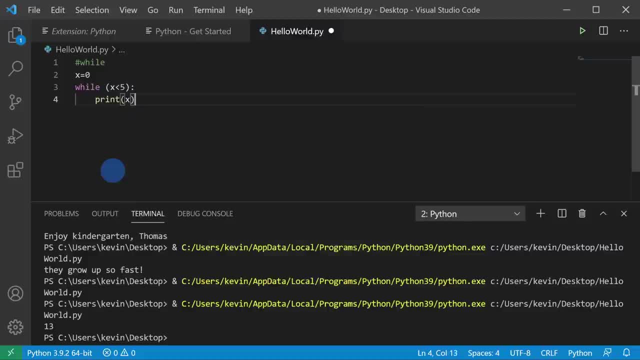 And here I could just say: let's say print x, So I'll enter that in. And then, right after I print x, I want to make sure I increment x, Otherwise it'll be an infinite loop. So here I'll type in: x equals x plus one. Just a really simple example. We start out at zero. 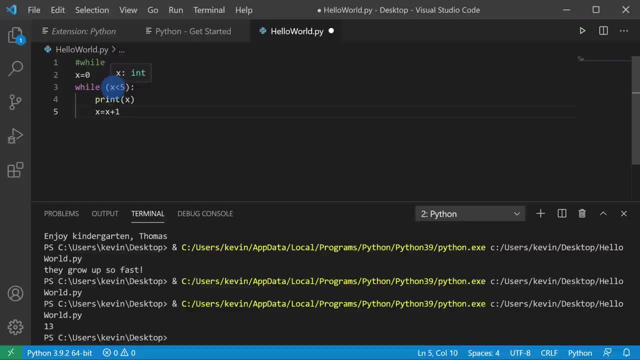 and here it'll say: if x is less than five, in which case it starts at zero, it is So, then it prints x and then we add one. So now x is one and x is still less than five, So it'll keep executing until it reaches four. So let's run this to see how it works. 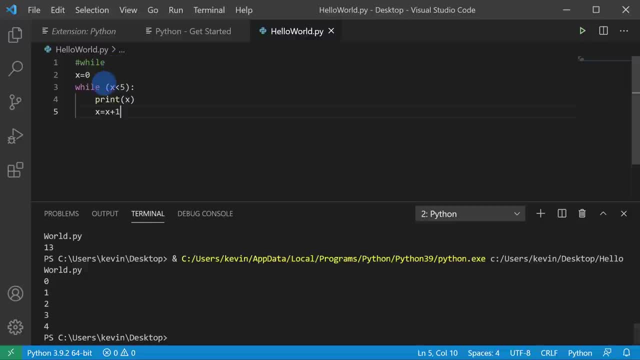 So here it prints out zero, one, two, three, four, And then once x equals five, well, it's no longer less than five. So then we exit our loop and it's all done. That's the basics of how you can create just a very simple loop. There's also another loop called a four loop. 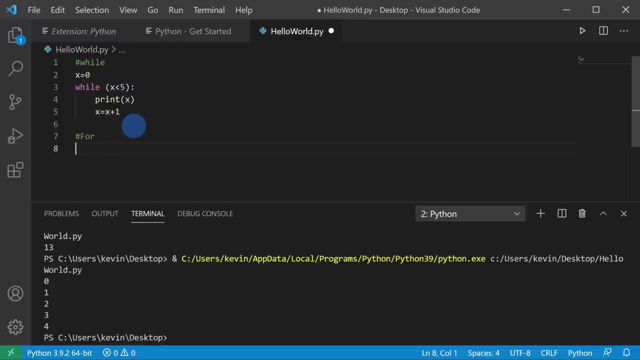 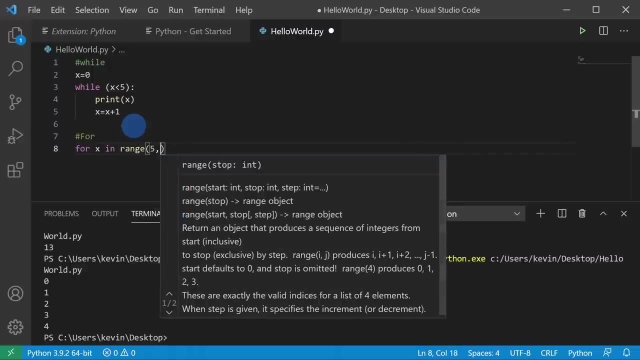 So I'll go down right here and let's type in four- And this is also pretty simple. Here I can type in four, and let's say four, x in range, let's say five through ten, And then here I'll close the parentheses, enter a colon, and here too I'll print the value of x. 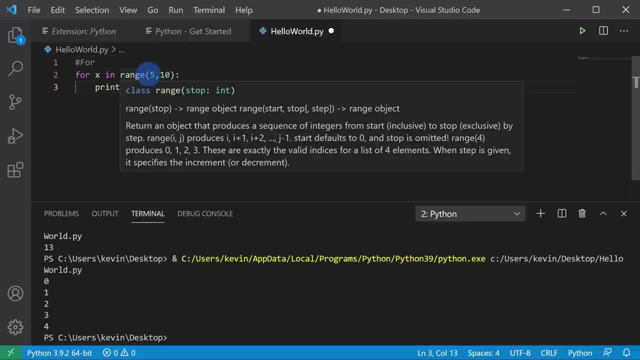 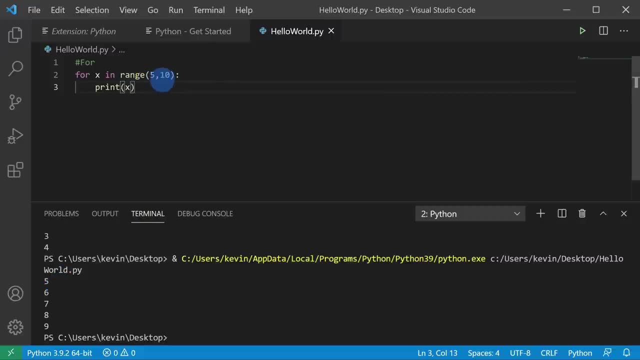 Let me delete the code up above And here. what it'll do is it'll go through that range. So when I hit run here, you see that it starts at five and it goes all the way up until ten, but it doesn't include ten. So this is another form of a loop that you can use. 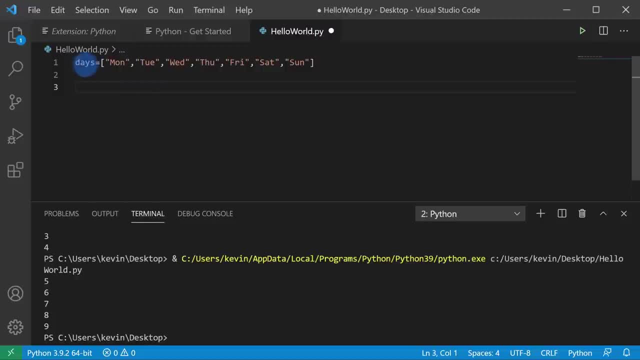 You can do some pretty neat things with loops. Here, for example, I have the variable days and I have an array assigned to it And these are just the days of the week. Here I can use a four loop to write out all the days of the week. 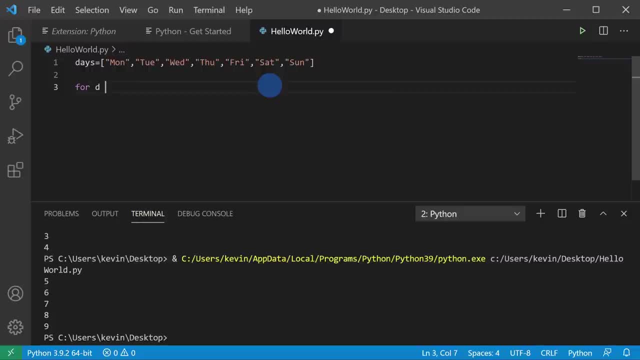 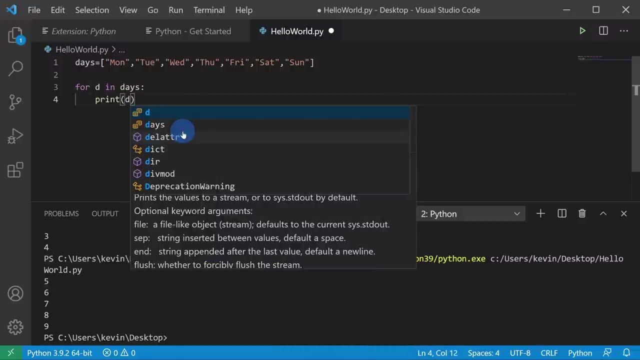 So here I could say four d. here I'm creating a variable And I'll say in days. so here I'm looking at this variable, Here I'll insert a colon and maybe I just want to print out the value of d, So as it goes through each day of the week. 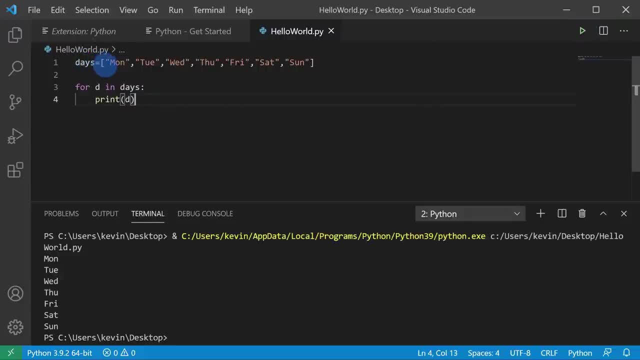 And here I can enter run, and here it'll go through the variable of days, and here it prints out every single day of the week. So that's pretty cool. Now, one of the neat things, too, is you can start using some of the logic that we learned up above in your loops. So let's say that I want to know. 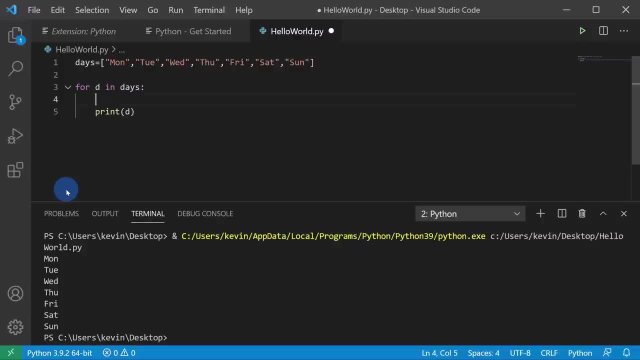 what are all of the days before Thursday. and once we hit Thursday, I want you to stop Here. I can insert an if statement, So I'll say if. and let's say if d is equivalent to, let's say, Thursday, So I'll type in Thursday, and at this point I want it to stop, So I'll type in break. So here, if we, 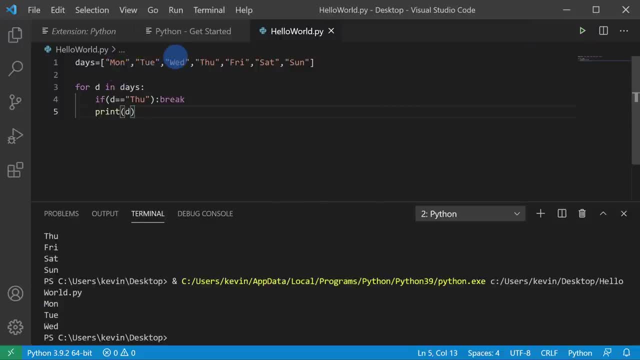 click on run here, you'll see it goes through Monday, Tuesday, Wednesday and then it looks like it hits Thursday and at that point we stop the loop. So at that point we break and we no longer print any of the other days. With loops we can also skip over items, So let's say that once. 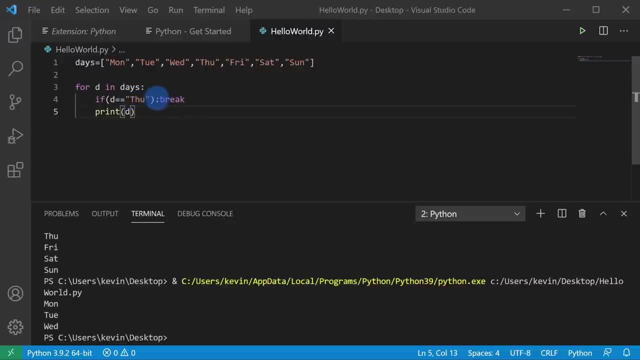 we get to Thursday. I don't want it to include Thursday in the list, but I still want it to continue and look at Friday, Saturday and Sunday. Instead of using break, I can use something called continue. So now, when I run this, 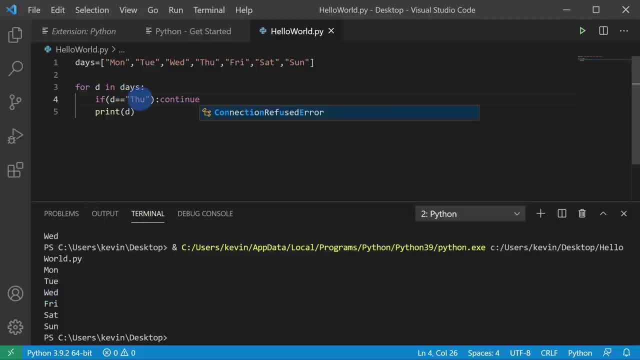 code. Here you'll see Monday, Tuesday, Wednesday, and then it found Thursday and we simply want to skip over that item, So we added continue. So here you see, it skips over, and then we get Friday, Saturday and Sunday. So once again you can use logic in your loops. You could also have it break. 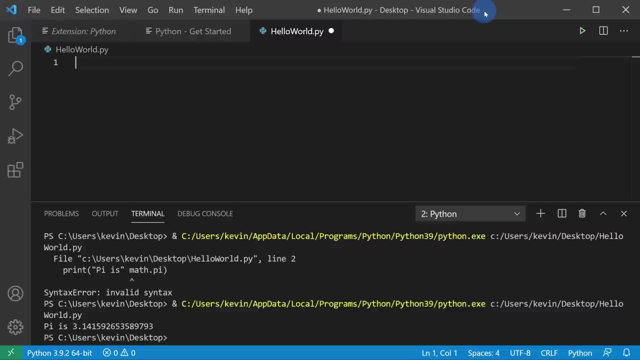 and continue. So far, throughout this video, we've been looking at some of the fundamentals and we've been writing all of our own code. However, one thing you can do is you can build on top of what others have already done, using libraries and also modules, And there are lots of fantastic. 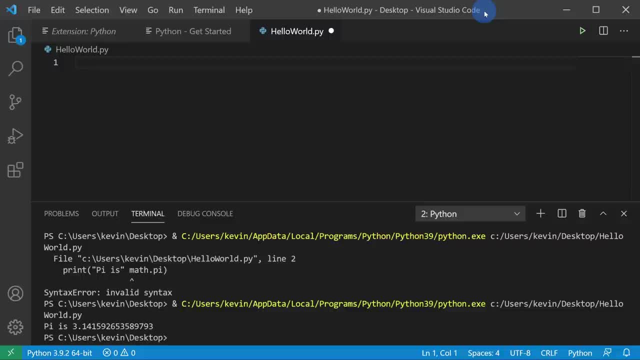 libraries that you can use. Let's say, for instance, that we want to print out the value of pi. It turns out there's an existing library called math. We could simply type in import and type in math, And right beneath that let's use our standard print function and here I'll type in: 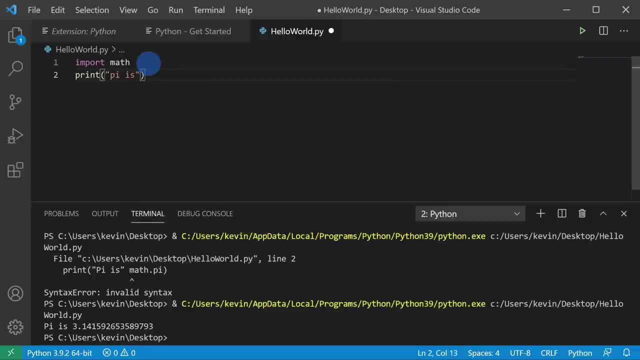 print. and why don't we say something like pi is, and then I'll insert a comma, And here I'll type in math, and then I'll insert a comma, And here I'll insert a comma And here I'll type in print. and why don't we say something like pi is, and then I'll insert a comma and here. 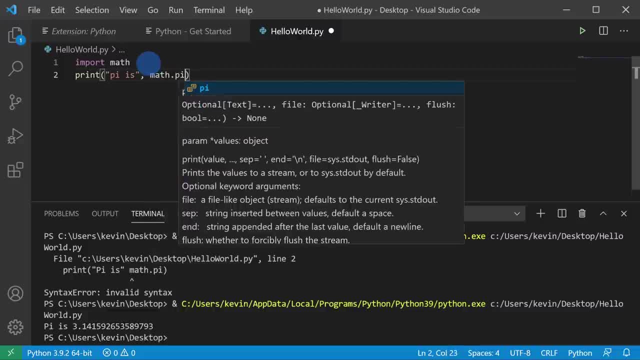 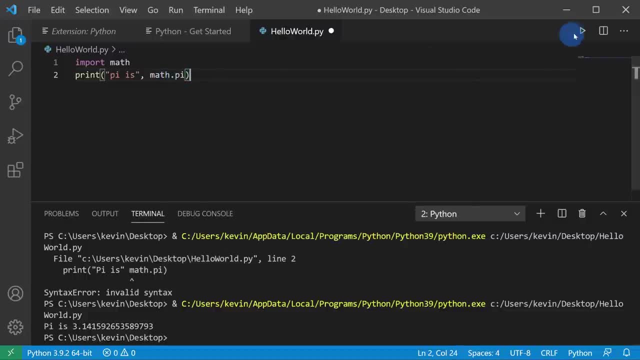 now I can refer to the math library and I'll type in py. so I want to get the pi value back And here, as I'm typing that out, you'll see all sorts of suggestions of what I could use. So here, when I click on run now, here it'll print out the value of pi. So once again, 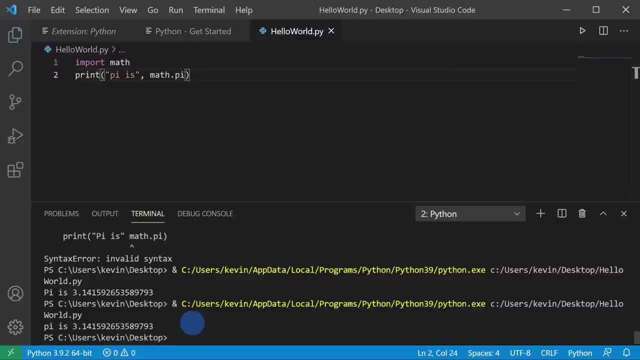 when you're programming, you don't necessarily have to write everything on your own. Instead, you can build on top of what others have done. If you were following along today, you might have occasionally run into different errors as you were trying to execute your code. 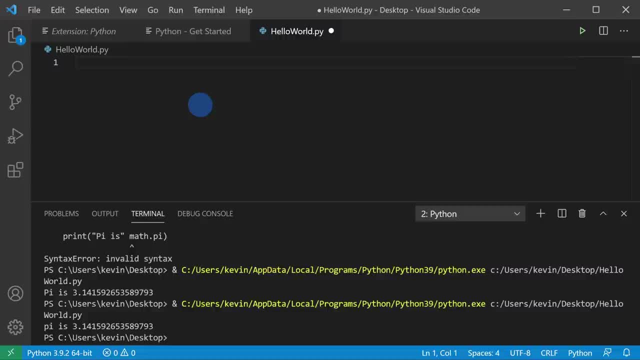 and they can really be a pain to resolve. I want to go through three of the key errors that you might run into and how you can resolve them. So let's take one example Here. I'm going to type in print and I'll type in: hello world. 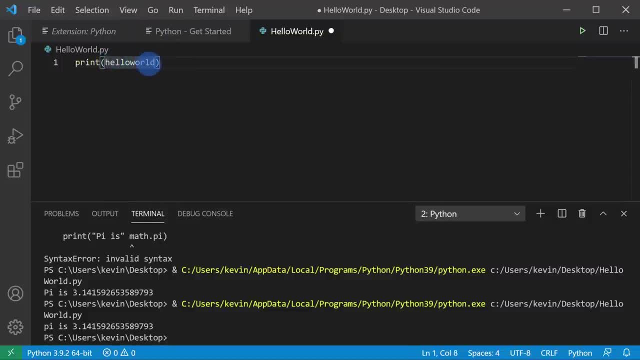 Now, if you've been following along, you probably know that every time I type in this function and I type in text, I need to include my quotes around this, but I haven't done that When I hit run right now here, I get an error, and this is referred to as a syntax error And the reason 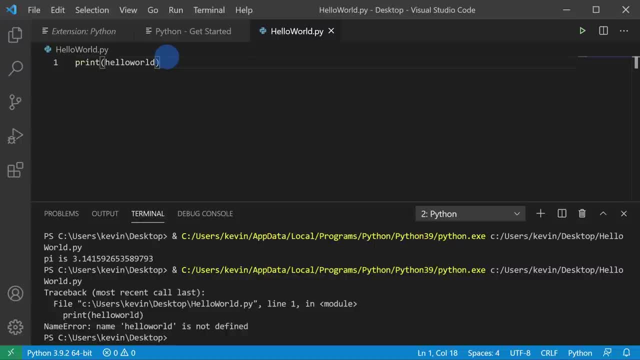 why is? I did not type in the text that I typed in. I did not type in the text that I typed in. I didn't follow the rules of the print function. I didn't follow the syntax rules for Python. The best way to troubleshoot these is to simply look through your code. 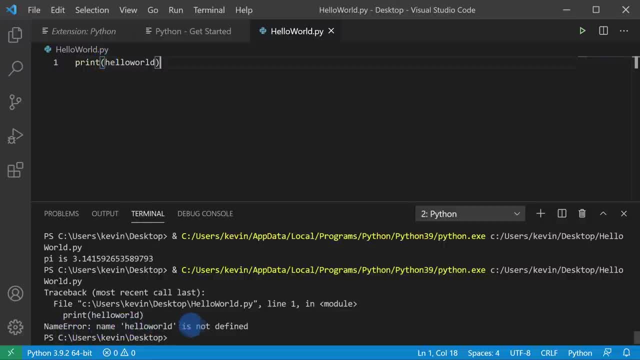 to find out where the error might be. So here I get name error. Hello world is not defined, So here it thinks hello world is a variable. So this is one way where you can look at the error message down here and that'll help you troubleshoot up above what the problem is. 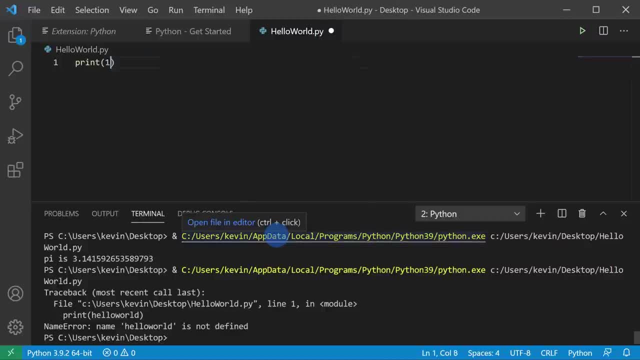 Now you might run into another type of error. Let's say I take 10 divided by 0, and then I try to run this, and we all know that you can't divide by 0. Right here I get a 0 division error. 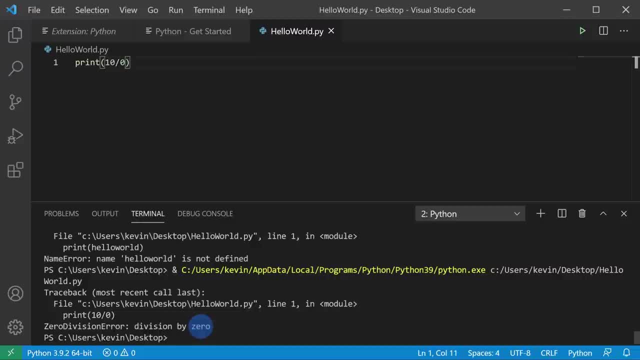 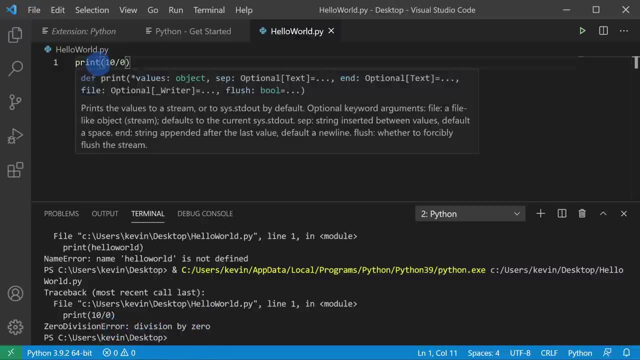 division by 0. This is referred to as a runtime error. It just fails. Now you could look down here at the error message to see what it was, and that might help you troubleshoot where the problem is in your code And typically when you get an error message.